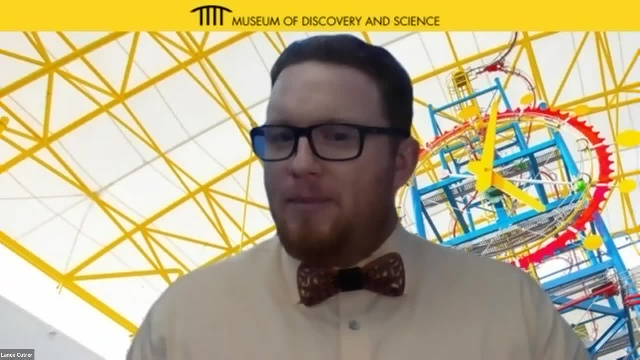 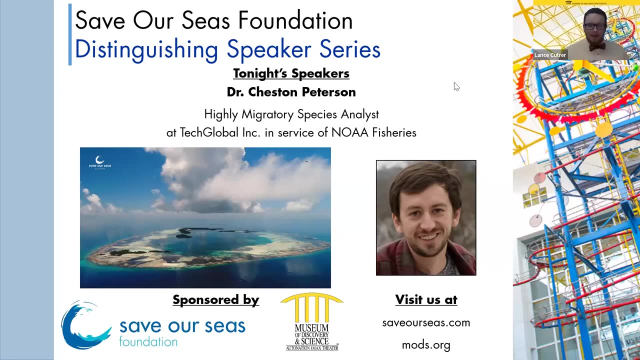 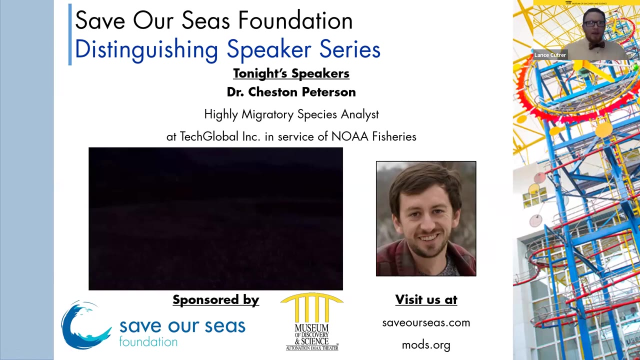 A few things about the, the museum and this program. We are very honored to be sponsored by the Save our Seas Foundation in doing these these talks. The museum itself is, like I said, based in Fort Lauderdale. The mission of our, of our museum, 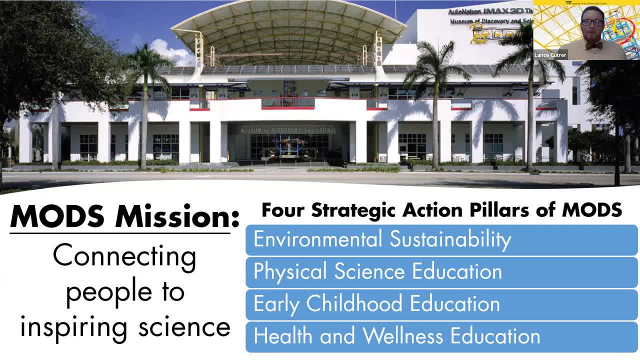 is to connect people to inspiring science And we do that through four different pillars here at the museum, that kind of drive everything that we do. Our strategic action pillars are physical science education, early childhood education, health and wellness education and where these talks fit in. 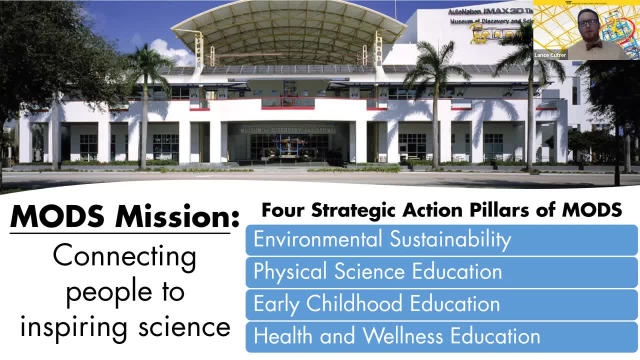 is into our environmental sustainability efforts that we are doing here at the museum. I am the director of environmental sustainability here at the museum and we're doing all kinds of things from paid internship for high school students to bringing in world-renowned scientists to spread information- all about ecology. 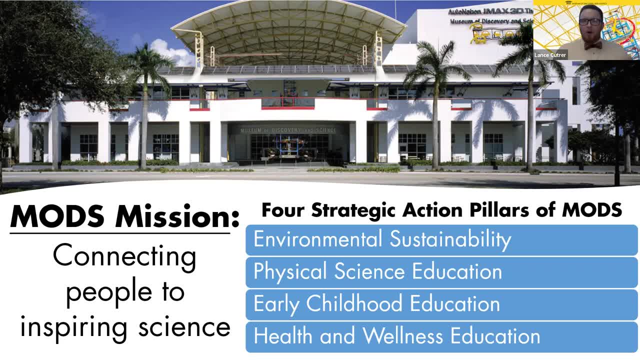 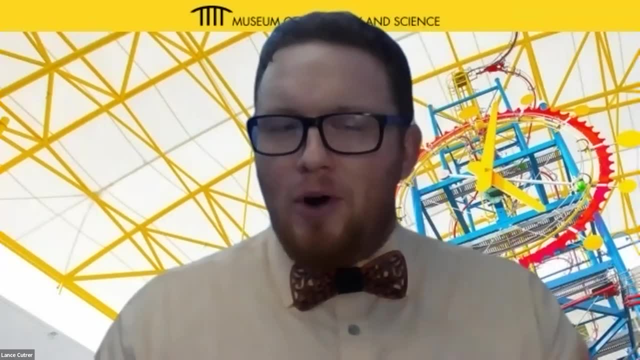 and conservation of the natural world. So we're always looking to do fun things and educate the public wherever we can. So with that I will introduce Dr Peterson and we'll turn it over to him. So we'll go. Cheston is a marine fish ecologist. 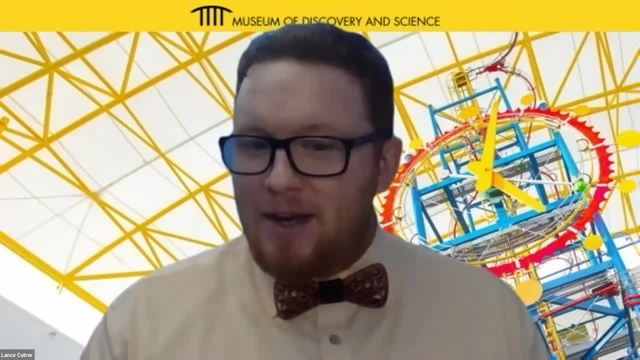 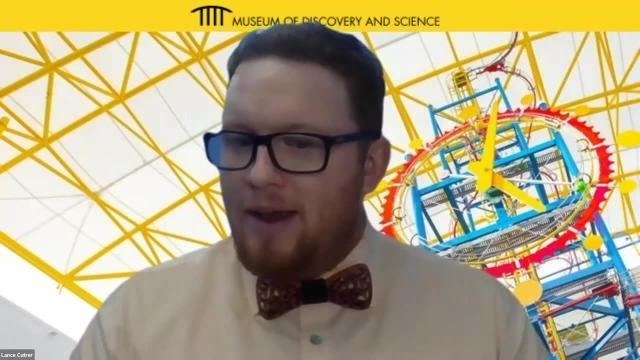 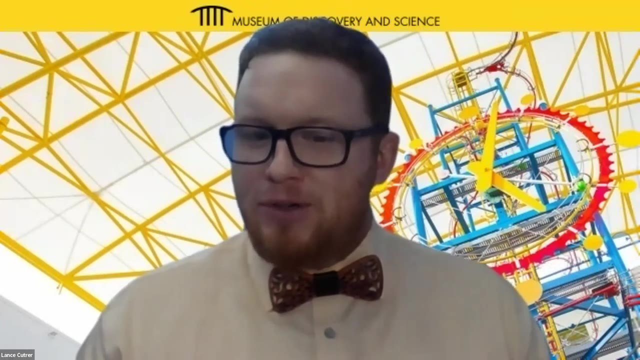 who specializes in coastal sharks. He's been fascinated by the natural world from a very young age, but nothing has captivated Cheston like water and everything that lives within it. When he was growing up in Tennessee, his first loves were frogs and especially salamanders. 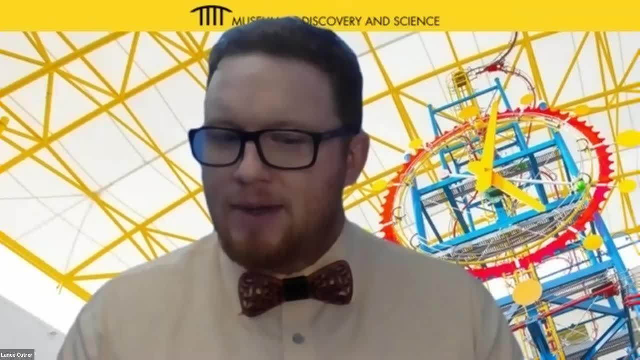 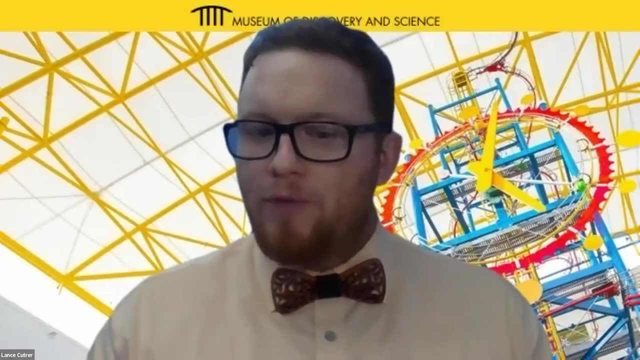 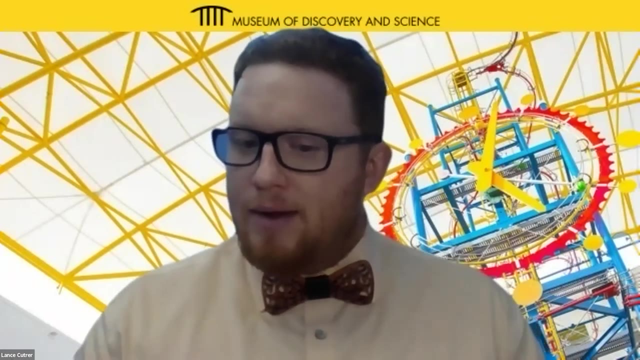 but later transitioned to fish. sharks and rays became, I think, one of his favorite things to look into. During his undergraduate studies, his interests became more focused on fisheries management and conservation. Doing through volunteer work, Cheston gained some positions through the Mote Marine Lab. 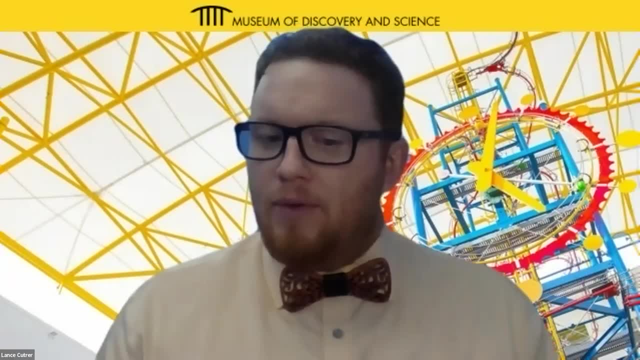 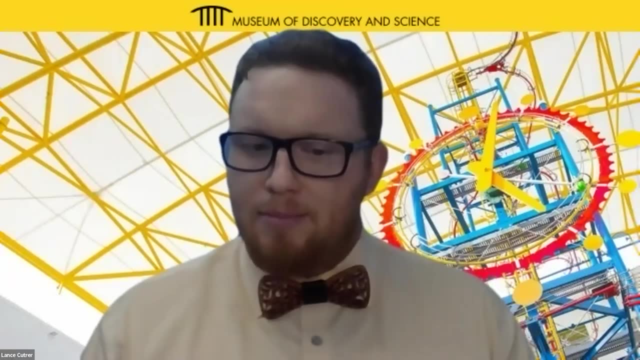 and an internship with them and eventually found himself on his way to graduate school. Cheston has been involved with several projects during his master's and PhD and he's been involved with several projects during his master's and PhD. and he's been involved with several projects during his master's and PhD. 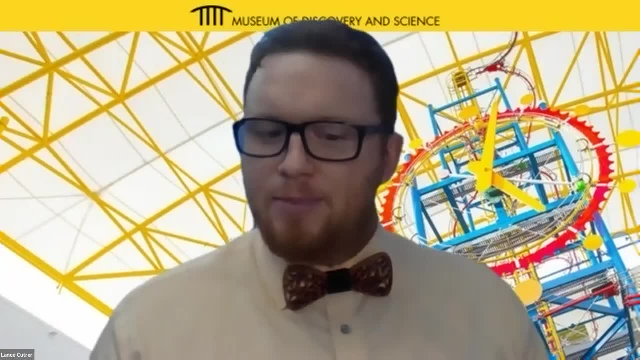 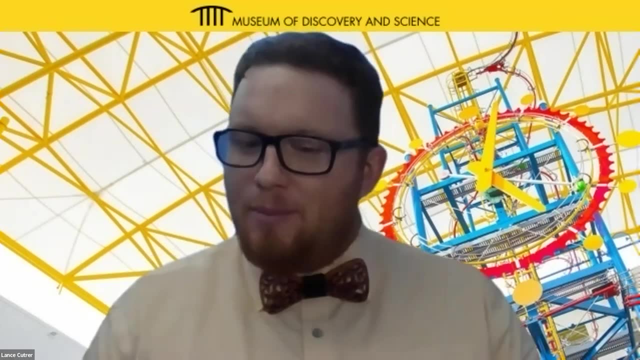 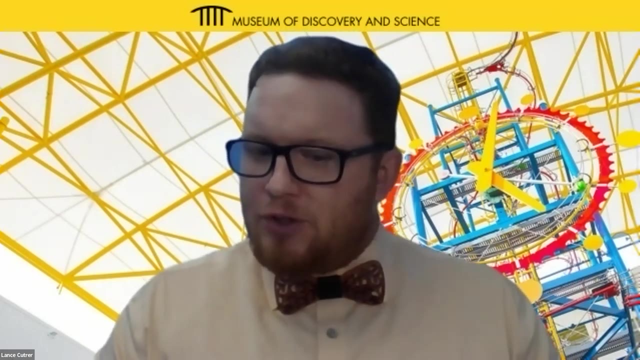 most of which involve or revolve around various aspects of coastal shark ecology, from topics such as spatial patterns of distribution, where the sharks are- and abundance of fishes. in Florida, especially in the Big Bend Panhandle area, Cheston has tried to find the intersection. 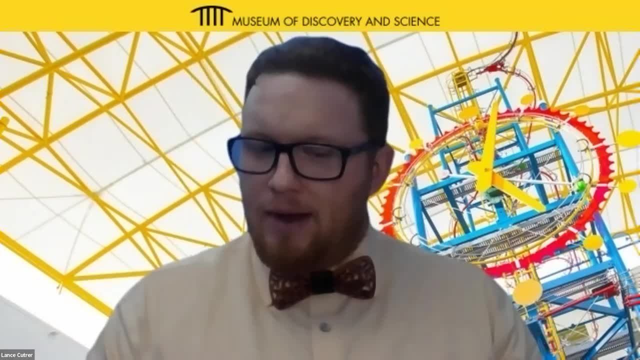 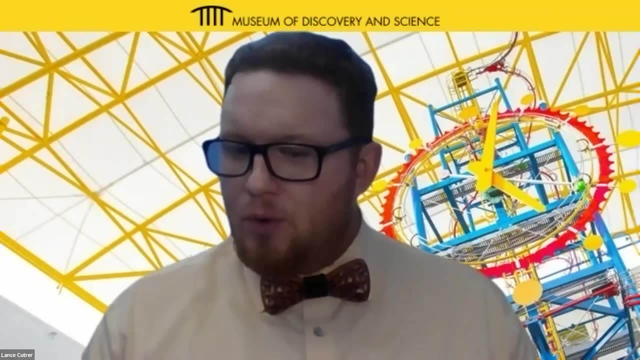 and the basics of applied science, and maintain a balance that work by pursuing questions and maintain a balance that work by pursuing questions and maintain a balance that work by pursuing questions fundamental to ecology, while collecting data that are also useful to management and conservation. 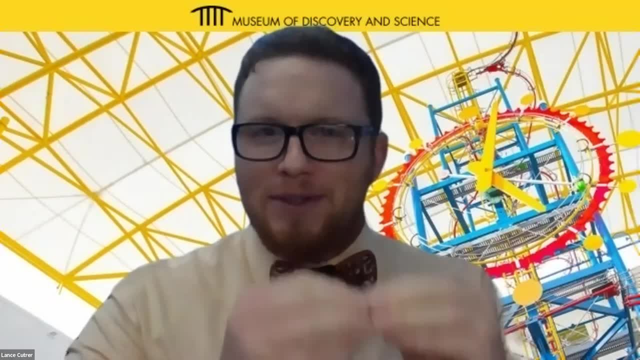 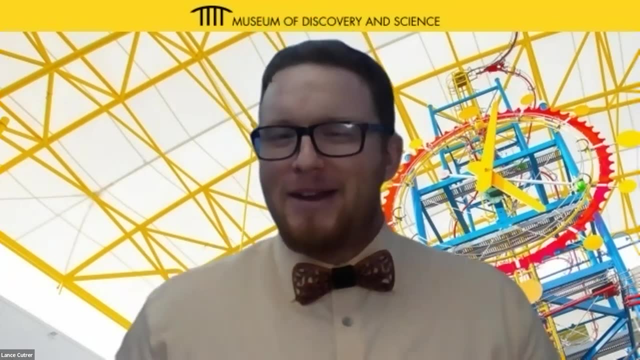 So marrying those two things of useful science right Where we can take it out into the field and use it for something to make our world better, So that's really awesome. I'm really excited about that. So, without further ado, Cheston. 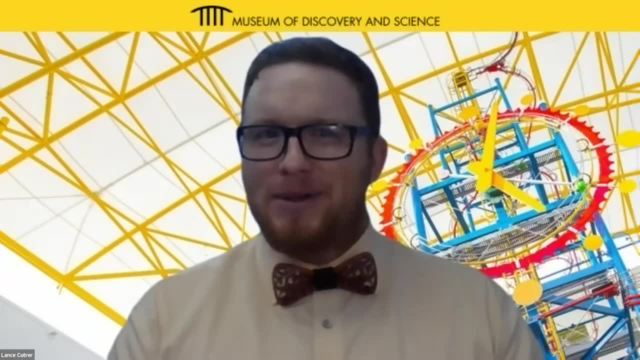 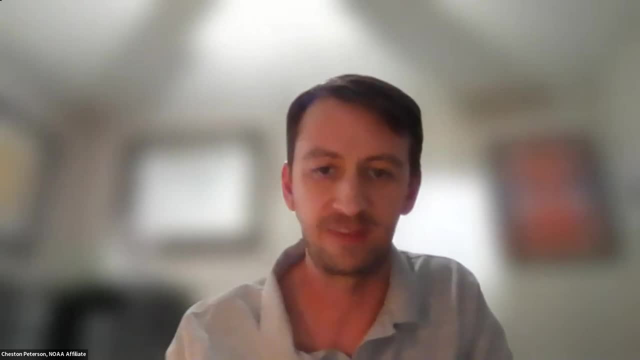 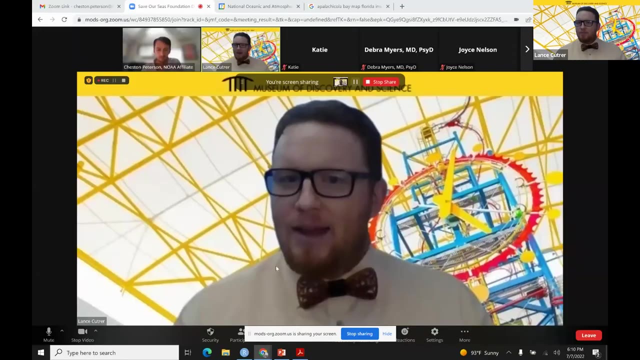 welcome to the Distinguished Speaker Series. Thank you, Lance. I'm excited to be here. I appreciate that introduction. That was great. I'm gonna share my screen here. Yeah, go ahead, share your screen And, like I said, if anyone has any questions. 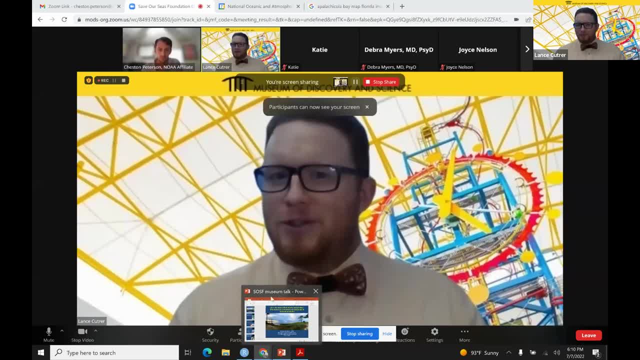 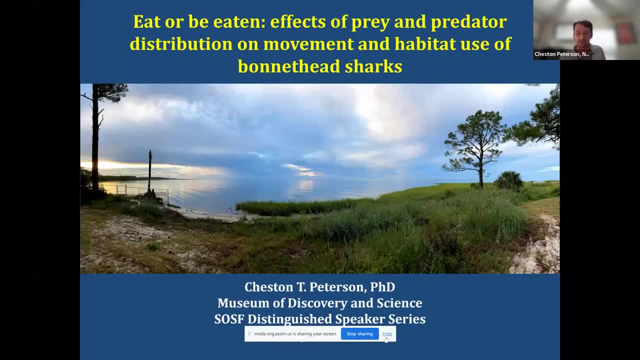 please feel free to put it in the chat and we will go through all right, All right. so thank you again, Lance, for that introduction. Thanks everybody for coming. I appreciate you taking time to tune in and hear me speak. I'm really excited to be invited to do this. 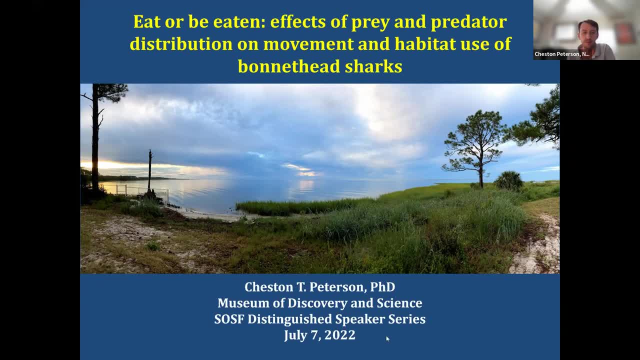 and give this talk. I think this is a great series and just excited to be a part of it. So, as Lance said, I'm going to talk to you guys mostly about bonnethead sharks in Apalachicola Bay, The title of my project, which was sponsored by Save Our Seas. 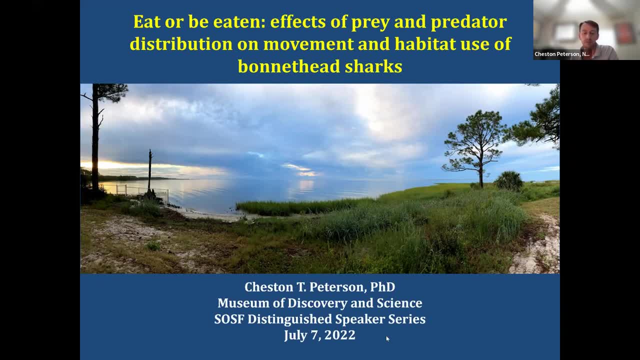 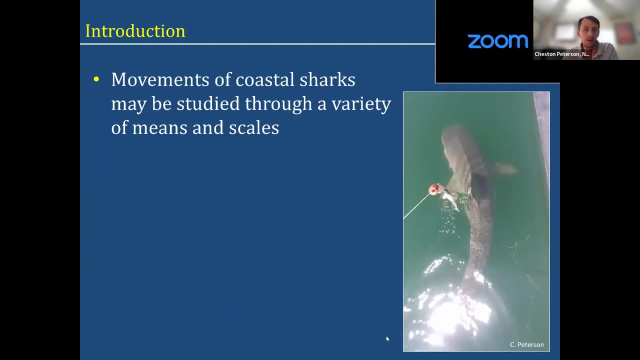 was Eat or Be Eaten. Effects of Prey and Predator Distribution on Movement and Habitat. Use of Bonnethead Sharks. And, as Lance said, feel free to throw a question at me And if there's any kind of terms or jargon I'm throwing around just to clarify, just speak up And so I'm going. 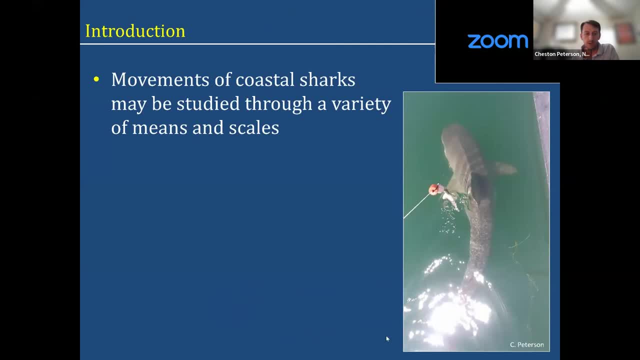 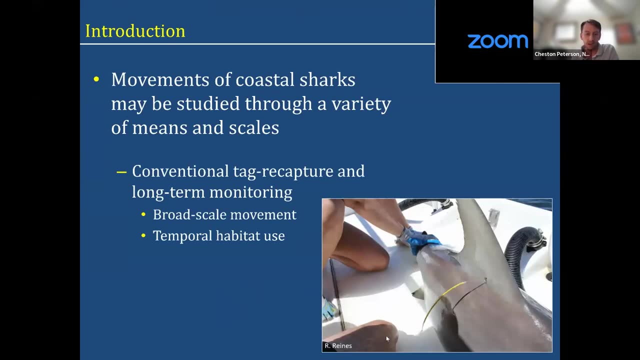 to give just a brief introduction about why we study movement and how we study movement of coastal sharks, which can be studied through a variety of means and scales. Conventional tag recapture and long-term monitoring are what you might see a lot of, where we just simply put a tag in a shark and if it's recaptured, and by fishermen- 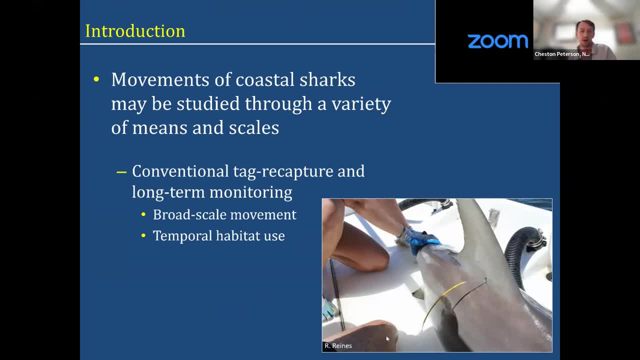 by other scientists. they hopefully will call that in and tell us where they caught it, how much it's grown and that kind of thing. So we can get an idea of broad scale movement, some ideas of seasonal habitat use, things of that nature, Whereas we can use more advanced tagging technologies such 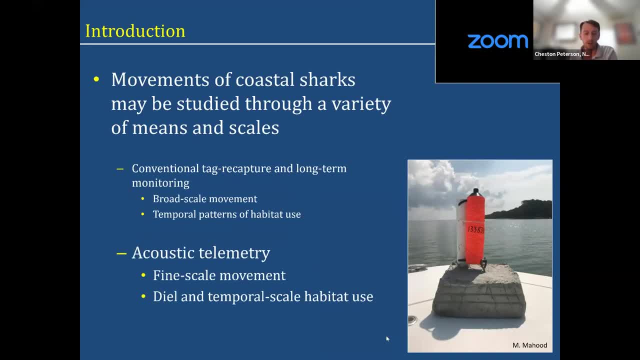 as acoustic telemetry to look at fine-scale movement, and we can look at diel, or patterns throughout the day, or temporal scale patterns throughout the seasons or years of habitat use, and so this gives us much more fine-scale, detailed information, usually over a shorter period of time, where we don't 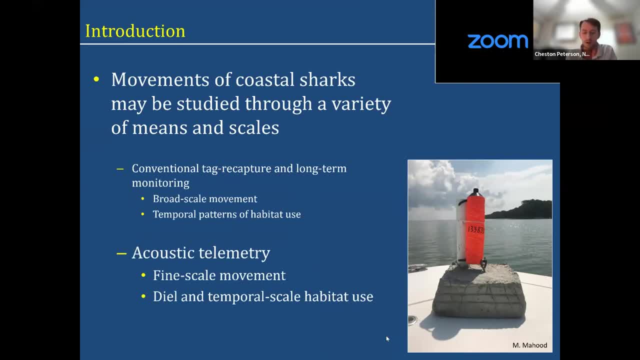 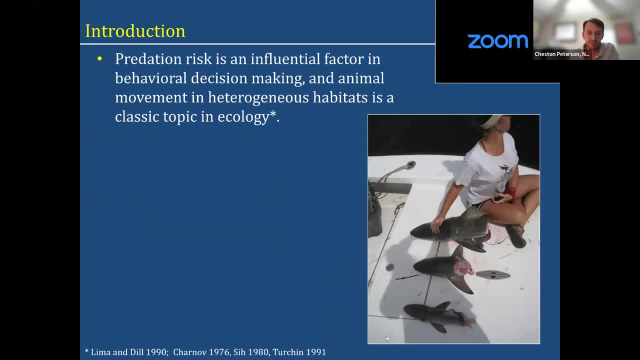 have to fill in those gaps quite as much, and so that's what I'll be talking about and using today, And so I should mention- there are a couple pictures here, just some- some sharks eaten by other sharks, so hopefully that doesn't bother anyone, but this is a major thrust of this project, So predation risk is an. 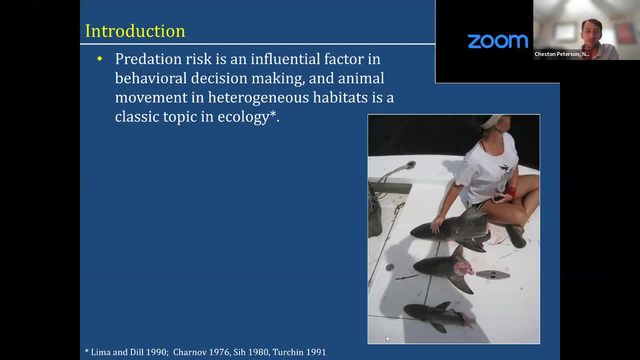 influential factor in behavioral decision-making and animal movement, and heterogeneous or mixed habitats as a really classic topic in ecology, and so a lot of research done in these fields has been historically with terrestrial organisms such as insects and spiders Looking at how they move through a patchy landscape of it could be bushes or 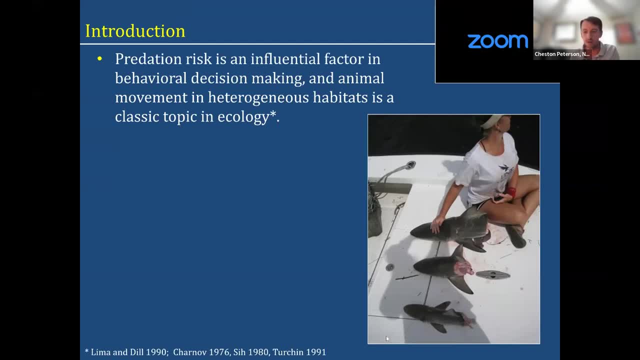 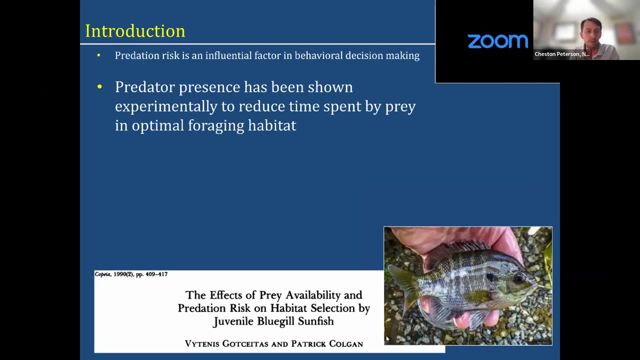 forests or whatever. and now we're trying to kind of turn those concepts to other species which may be a little more difficult to study, such as marine fish, especially sharks. And so we know the predation risk is an influential factor in decision-making and experimentally predator presence has been shown to 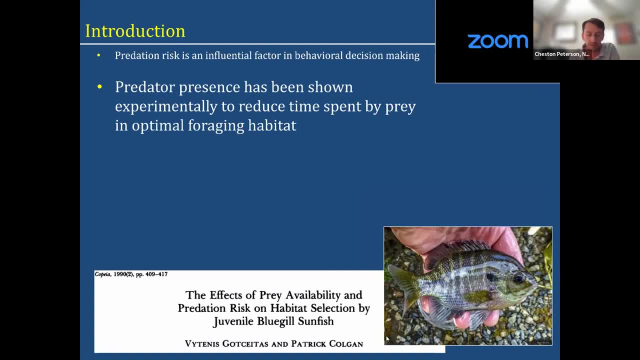 reduce time spent by prey in optimal foraging habitat. So this is an example of that. So some very classic work in ecology done with sunfish, a freshwater fish species, where they basically put them in, put them in tanks and monitored their behavior in the presence or absence of a predator. 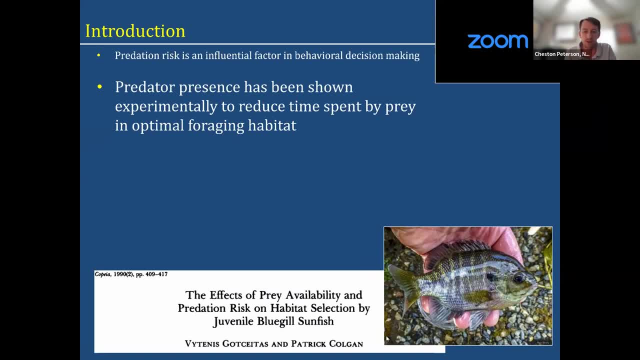 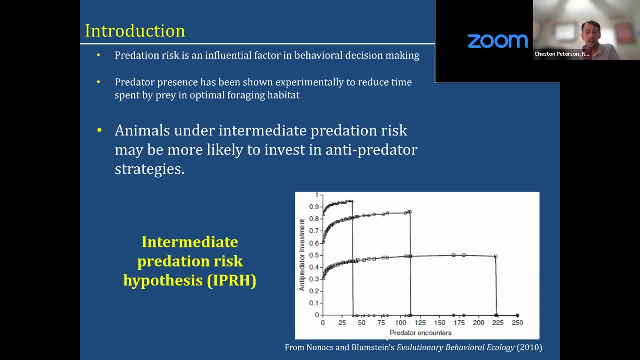 and it showed that they they essentially reduced how much time they were in the best habitat when the predator was around, And so we also think that animals under an intermediate risk of predation may be more likely to invest in anti predator strategies, and this is called the 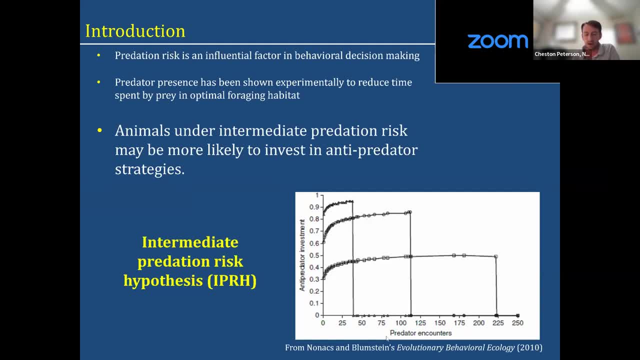 the intermediate predation risk hypothesis. And this is another kind of crux of my project. The idea here is that if I am a fish type of species that experiences a lot of predation, usually that is kind of ingrained in my life history So I may grow fast, mature quickly and make a ton. 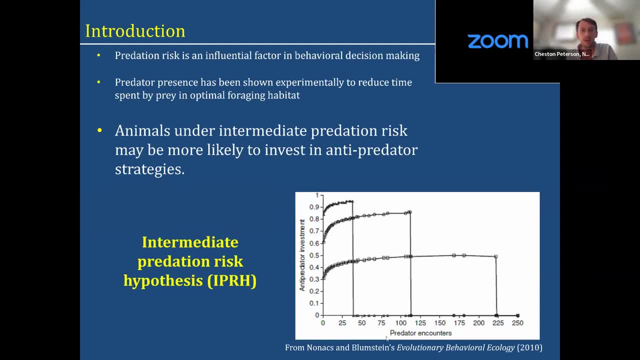 of babies, And if I do that, the risk of predation individually isn't that big of a deal because there's so many of us and we're so productive. So I as an individual may not try to avoid predators and invest my energy in that. Similarly, if I'm so large that the risk of predation is very 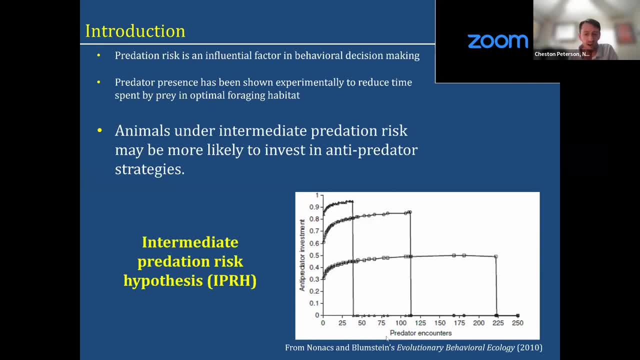 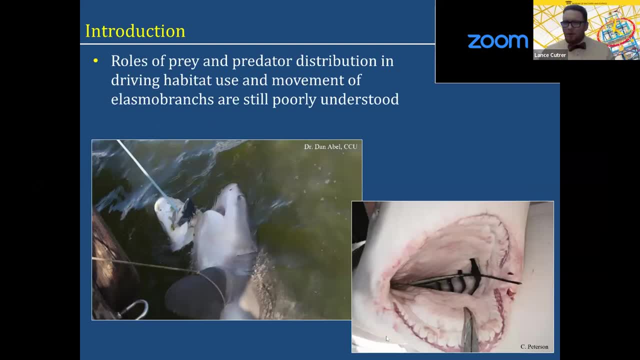 size, you may be the most likely to invest in behavioral potentials. So if you are at an intermediate risk, or of intermediate of my, my study species, Justin, can I ask a question? Oh sorry, Sorry, Can I ask a question? 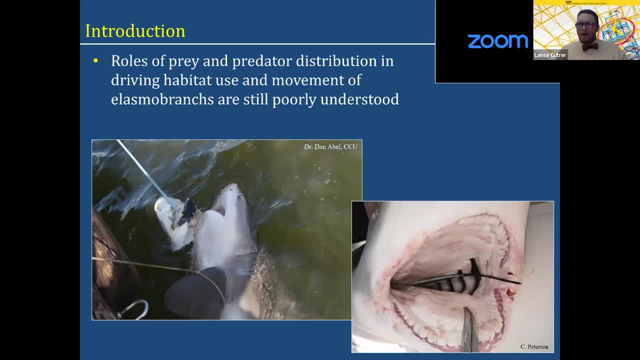 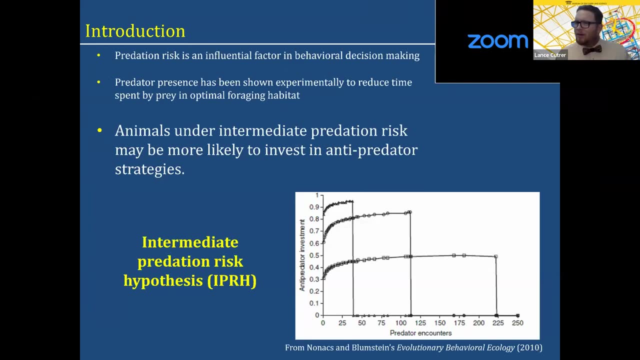 Sorry, Yeah, sure. When you're talking about anti, anti-predator strategies, what, what, what is, what are some examples of that? That could be modifying your movement patterns or habitat uses. Obviously, what comes to mind when I'm talking about this, where you're say I'm not 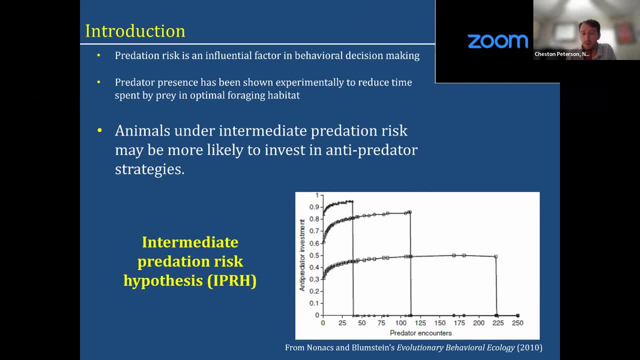 going to go in the most risky habitat, even if my opportunities to find something to eat are best there. So I'll go. I'll go somewhere where I'm I'm less likely to find food, but I'm also less likely to be eaten, And so that can be a fine scale thing where it may be how, how animals. 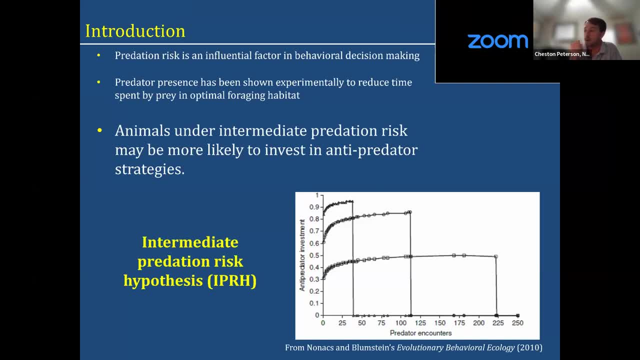 respond to the presence of a predator, or it may be a broad scale, kind of like an evolutionary adaptation to avoid high risk areas. Right, So so the animals themselves, in this case bonnets, which we'll get to in a second. 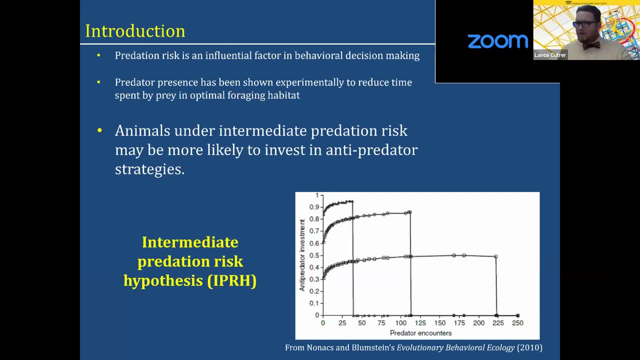 I'm sure. but they can remember essentially if they've had a risky situation happen to them and they would not go to that area again. maybe That's an excellent question. I don't know if it's remembered or the. I think the idea that this would be kind of ingrained And so that. 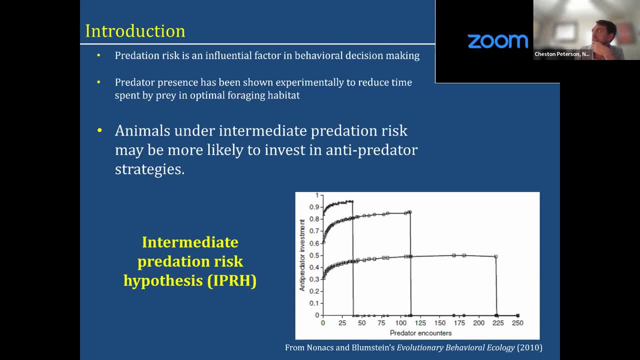 yeah. so I'm not sure that's a. that's a whole nother level of behavioral ecology to think: why are they doing These things? Well, I actually I can't answer, So you know, I guess there could be some triggers. 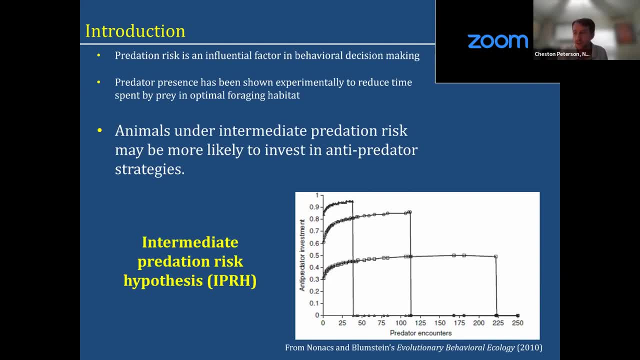 for that, because it's always a stress response, right, And so there's- usually there should be- a kind of a hormonal cascade that's going on, just like you or me. if we get nervous or something stressful happens, adrenaline starts pumping and our body kind of engages with that reaction, And so 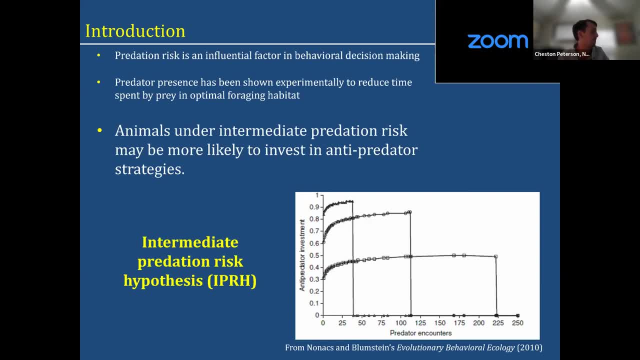 there could be things like for pheromone cues or smell cues. if they smell a predator, they're more likely to react. So they don't just be memory, It could be stress, that kind of thing. So that's a that's a great question. 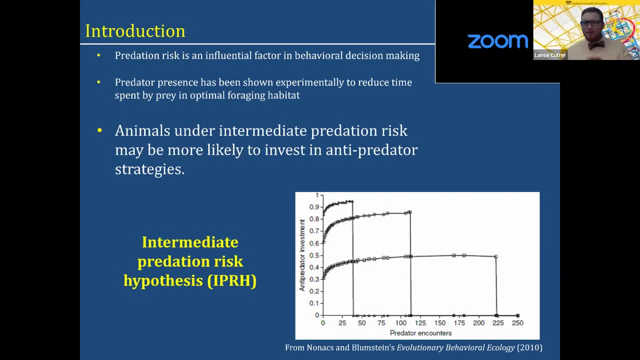 That's interesting. So, okay, So we're trying to figure out where they go, based on their risk assessment, whatever that means to them, right, Cool, Exactly, I understand. And so the these dynamics and sharks are really poorly understood. The role of predator and prey. 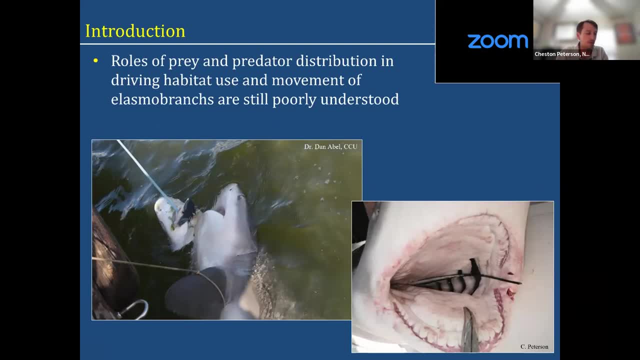 distribution, driving habitat use and movement is not well known. We've seen more of this research. some really more classic or things that have broken into the mainstream would be like: the reintroduction of wolves in Yellowstone is thought to modify the behavior of deer, which has led to the return, kind of. 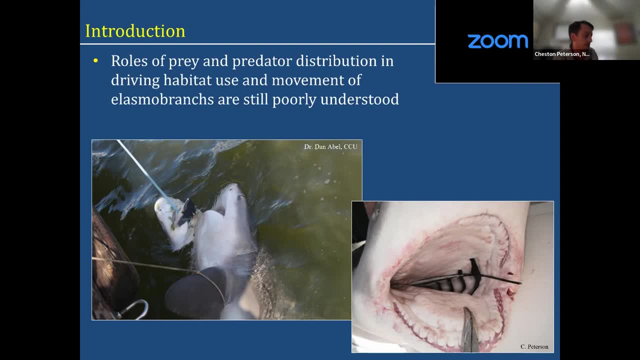 cascading effects of reducing pressures, essentially reducing pressures on plants so that native plants can come back after the deer have kind of hammered them. There's also a lot of research in the in Africa and the Serengeti looking at how, where you have a diverse community, 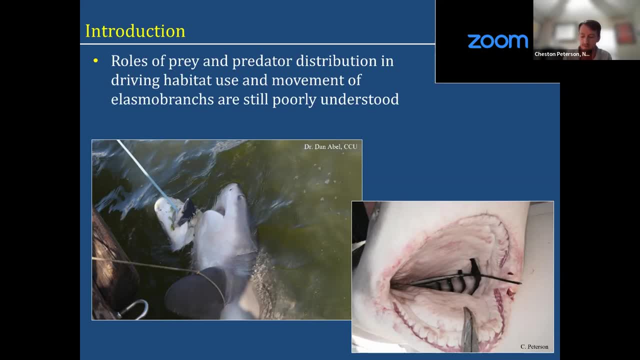 of predators kind of affecting each other And we have these guilds of dominance and that kind of thing. but but in sharks this is poorly understood and we're just kind of cracking into this. And so now we'll get to our, our study species. the star of the show, the bonnet heads. 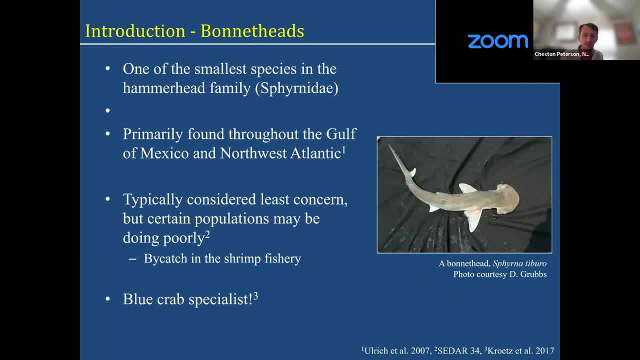 So this is one of the smallest, if not the smallest, in the hammerhead family, the smyrnids. They're often mistaken as a baby hammerhead. I get that a lot, but they're the only hammerhead with that- the distinct rounded front end on their cephalofoil or their head, so it gives them their. 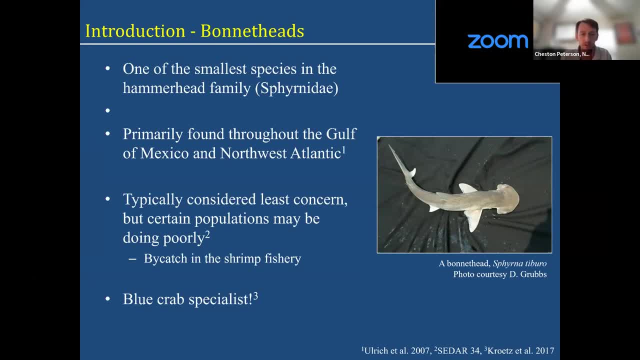 bonnet head name, Primarily found throughout the Gulf of Mexico and the Northwest Atlantic. Typically, they're considered a species of least concern in terms of a conservation concern, but certain populations may be doing poorly. This is coming from recent stock assessments. 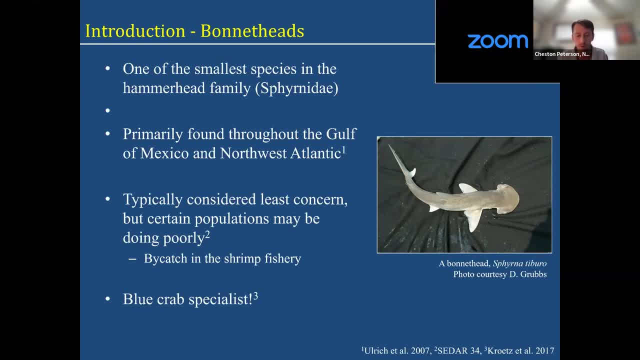 they're caught a lot as bycatch in the shrimp fishery and the trawl fisheries, and so that's a threat to them. then they're also a blue crab specialist, And so they love to eat blue crabs. That's ubiquitous across their range and very, very common, And so that's another really important aspect of them. 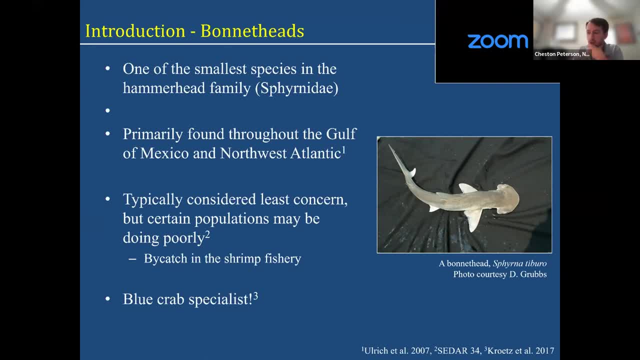 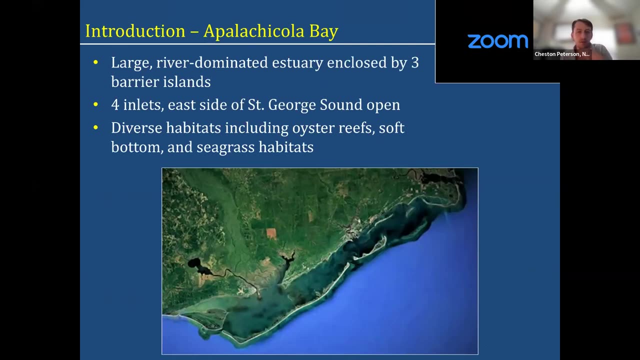 Bonnetheads are a small coastal shark. They're managed in that complex. They only get about three to three and a half feet long, about a meter long, And just really, really cool animals. And so our study system was Apalachicola Bay, which is a large river-dominated estuary. 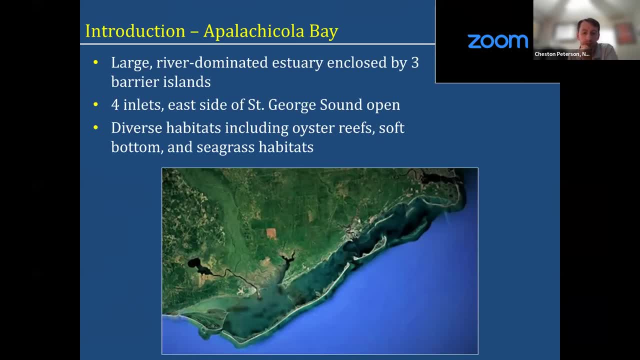 enclosed by three barrier islands And there's four inlets into Apalachicola Bay, but it's otherwise a very enclosed system And it's very diverse. So habitats include oyster reefs, soft bottom mud, basically, and seagrass, And so if you're not familiar with Apalachicola, 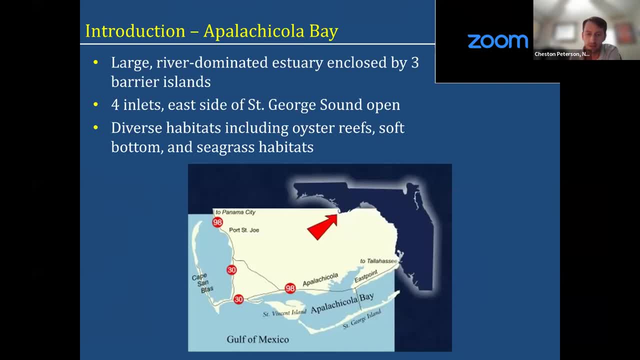 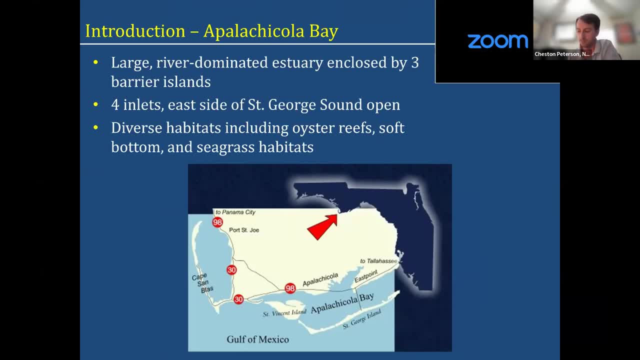 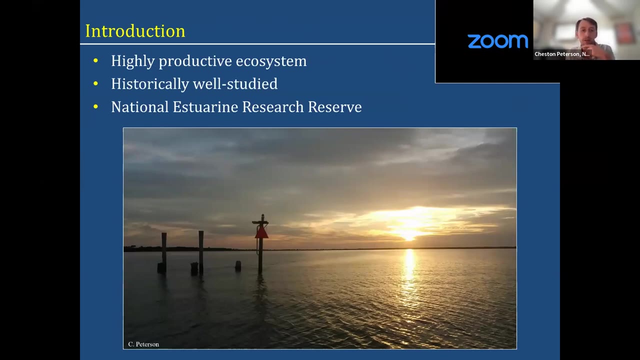 off the internet, But this was a major oyster production area. There's a huge oyster fishery here, And so you may be familiar with the region. This is a highly productive ecosystem, as most river-dominated estuaries are. It's a National Estuarine Research Reserve, And so historically, 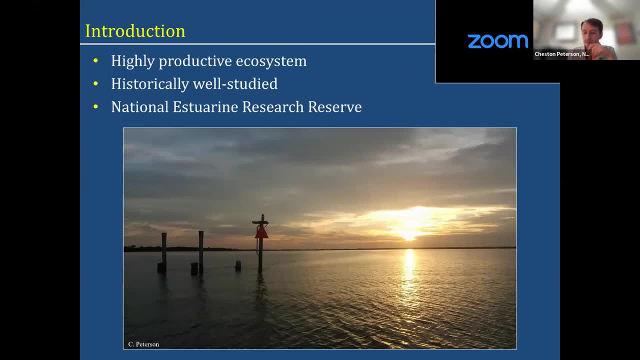 it's very well studied. The invertebrate communities and the small bony fish communities are really well studied throughout the Bay And there's been some work done on the sharks and rays, the elastomer brinks, but not as much There's been more. 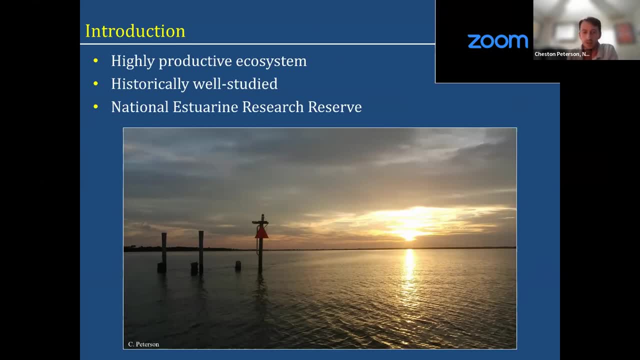 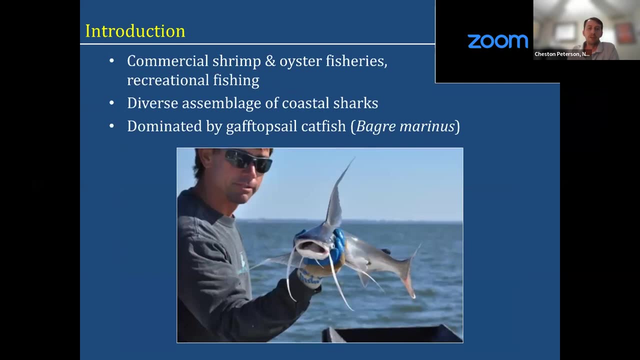 work on the sharks on the outside of the Bay and in St Joe Bay and some of the neighboring areas, mostly done by NOAA, And so, as I mentioned, there are commercial shrimp and oyster fisheries. There's also a lot of recreational fishing, mostly for sport fish and kind of inshore. 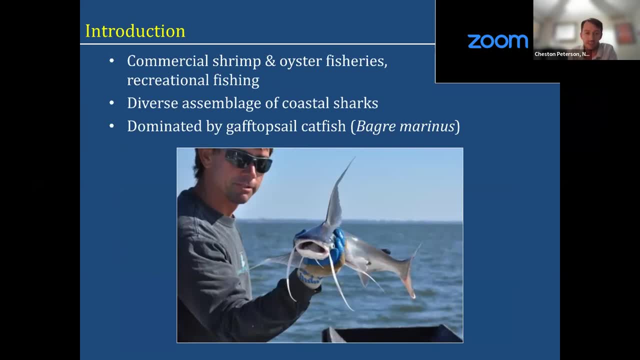 species like red drum and spotted sea trout, But the whole system is dominated by gaff-type sail catfish, which you see my former advisor, Dean Grubbs, there holding a gaff-type sail catfish, And so these guys are super abundant. They're actually another part of my project that I won't. 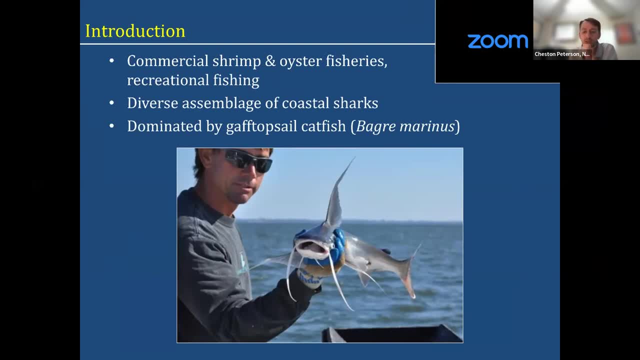 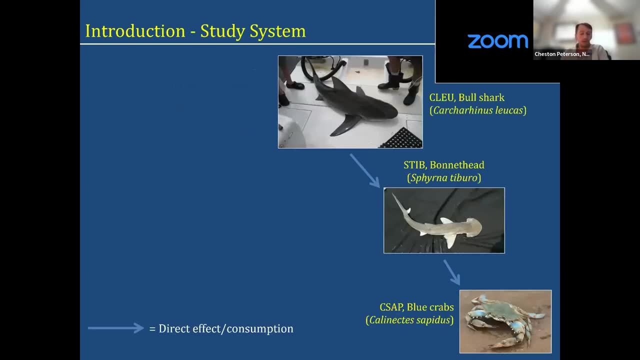 talk about today, But they're definitely the dominant fish species in Apalachicola. All right, So kind of getting into the thick of the study system here. I had three focal species that I looked at their interactions or tried to look at their interactions. So 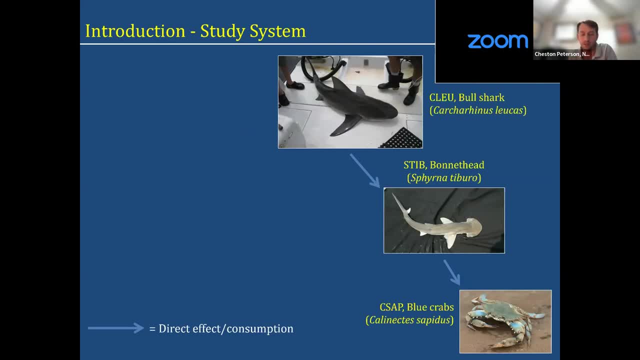 I've got these four-letter codes here that are just the first letter of the genus and the first three of the species. I use those throughout the talk just to refer to the different species. So bull sharks are C leu, C leu, Carcharhinus lucas, And then bonnetheads are STIB, S-T-I-B. 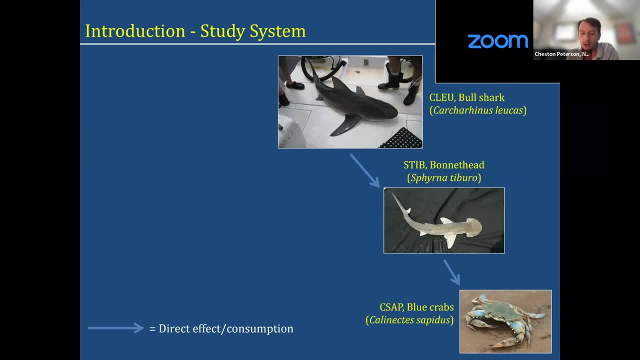 Spironotibaro. And finally, blue crabs are C sap, Calonectes sapidus, And so I have just a really simple food chain here, where that blue arrow indicates a direct effect or essentially an assumption. So that means you know we're looking at a direct interaction there. 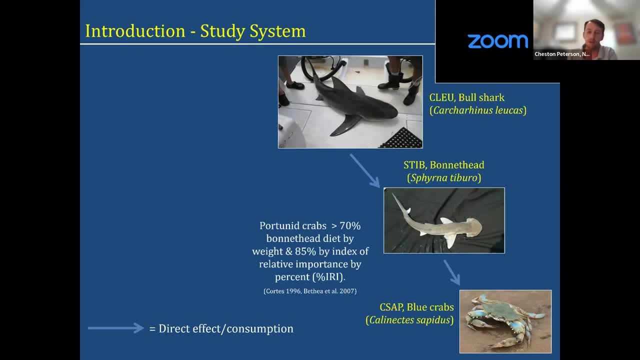 So Fortuna crabs, like blue crabs, make up greater than 70% of bonnethead diet, by weight, more than 85% by the index of relative importance, by percent or percent IRI. So there's a few different ways to quantify the importance of prey items. based on gut contents, These 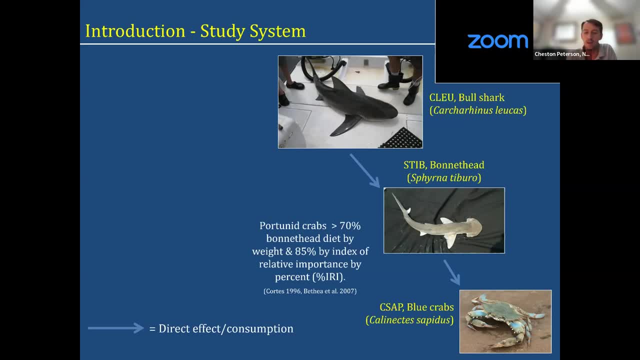 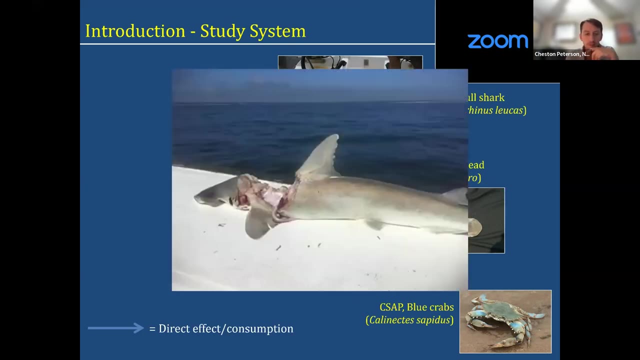 were some older studies from the 90s and early 2000s. But the meat, the point I'm driving here is that they like to eat blue crabs. They like to eat crabs. That's a big deal. And then this is another eaten shark image. but we know that. 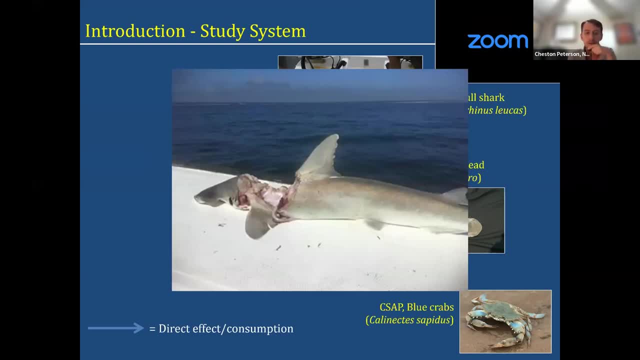 bonnetheads get eaten by bull sharks, because we've seen it happen in the field. So sometimes when they're caught in the net or on a long line, a larger shark can come up and depredate them. So we know this is a thing as well. We also know that elasmobranchs make up at least part of the bullshark wilds. 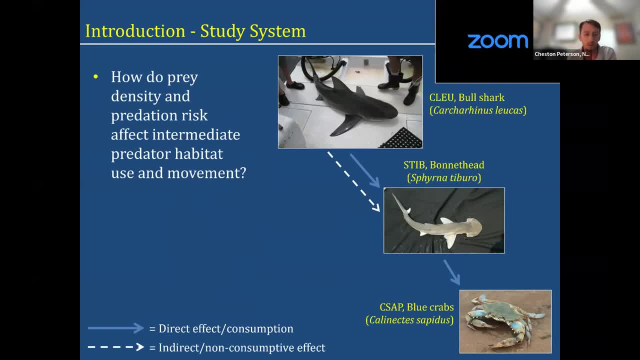 breaks make up at least part of the bull shark's diet as they grow, And so, all that being said, I'm actually not so interested in how often bull sharks eat bonnet heads or how many blue crabs bonnet heads are eating. I'm interested in indirect effect, or what we call non-consumptive. 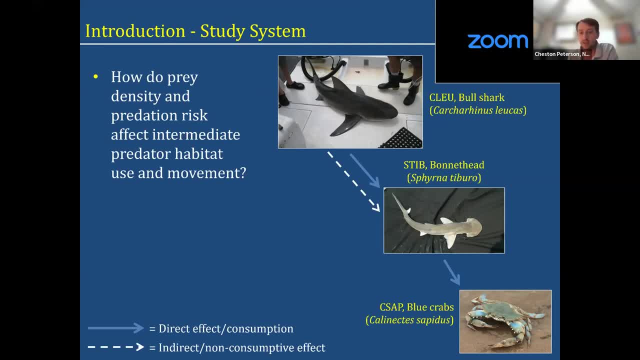 effects, And so this is when the presence or the threat of a presence of a predator may affect the behavior of our focal species. So this is exactly like what I was introducing and what Lance and I talked about. So we're more interested in how bull sharks indirectly affect. 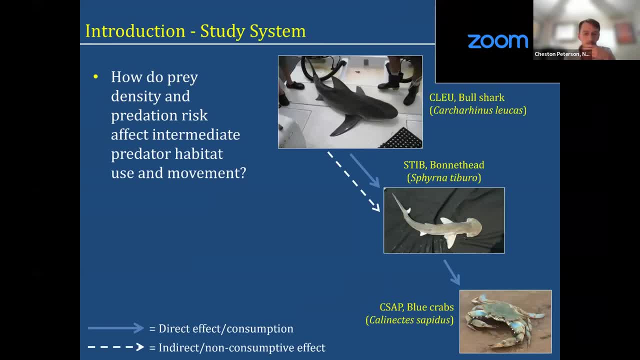 bonnet heads which can in turn indirectly affect the blue crabs, when we call that a cascading effect. And so this is kind of the main question here: How do prey density and predation risk affect intermediate predator, habitat use and movement And the intermediate predator here? 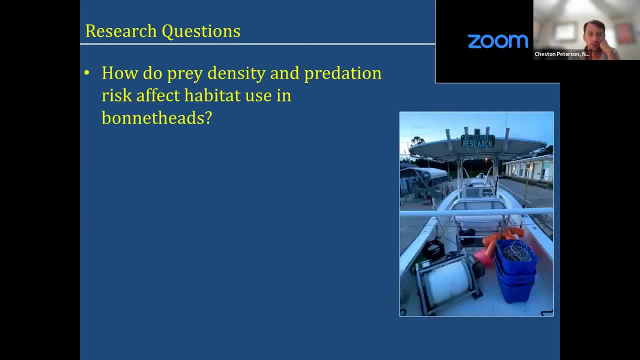 is the bonnet head, bonnethead, Um, can I ask another question? Yeah, sure, Lance. So, um, so we know bonnetheads like to eat crabs. What, how many, how many crabs can a, can a bonnethead go through in a in a day? 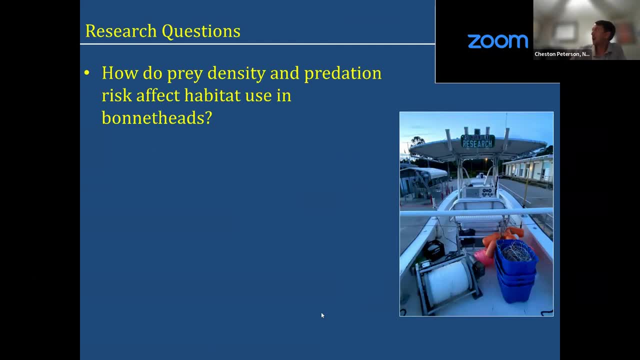 What would be there. Do you have a? do you have an idea on that? I don't know if there have been any like daily consumptive rates. I will say that, um, unfortunately, bonnetheads have a pretty high mortality rate, So we do a lot of um dissections to collect um aging structures. 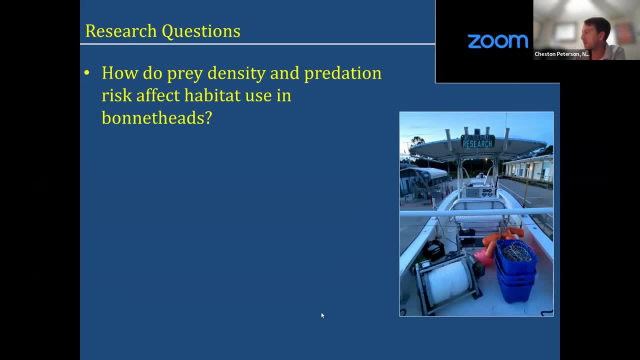 and guts to support management, And I will say that that every bonnethead I have examined had crab parts in them. Um, usually there are more than one. Um, the tricky thing is is the carapace of crabs uh, doesn't digest all that quickly and that will stick around for a while. So it's. 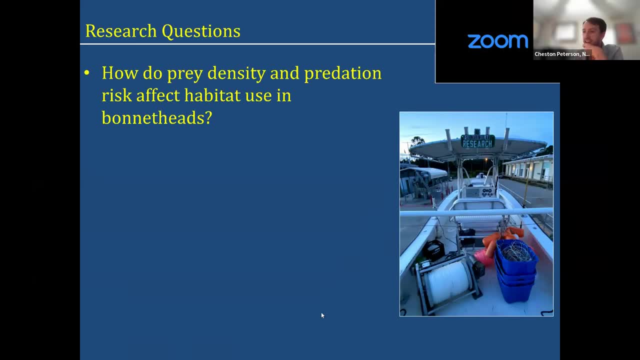 tough to say how long they've been in there, but my idea is that they're never empty. It seems like they've always got crabs in there. So I imagine you know, um, it would depend on the size of the shark and all and the size of the crabs they're eating. But, um, if I had to, 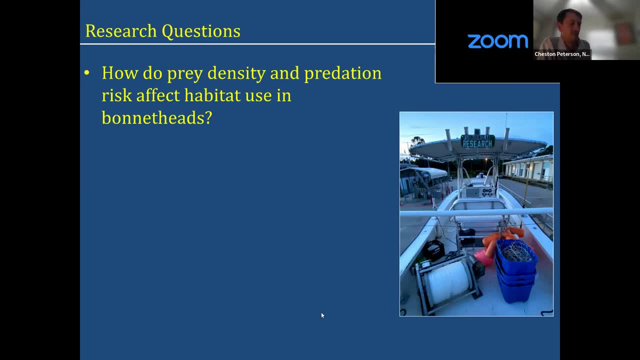 guess I'd say: you know, four or five crabs in a day is a good haul. That may be a lot. Um, I don't know. And and I my, my guess is that they wouldn't have to eat. you know, like a lot. 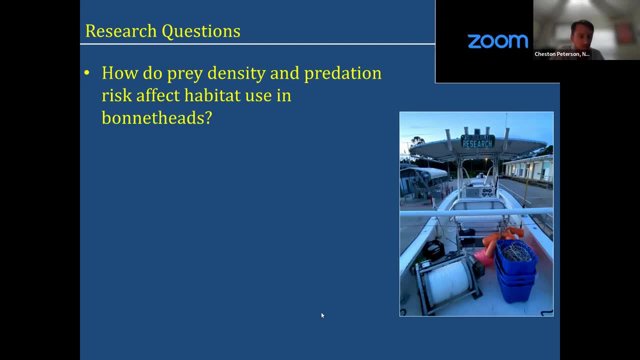 of predators like this don't always eat every day, or they eat in bunches, or maybe maybe you had a good day and I got four crabs. Um, I'll take it easy tomorrow, or I'll be, I'll be, I'll be good to go, in case that the the crab. 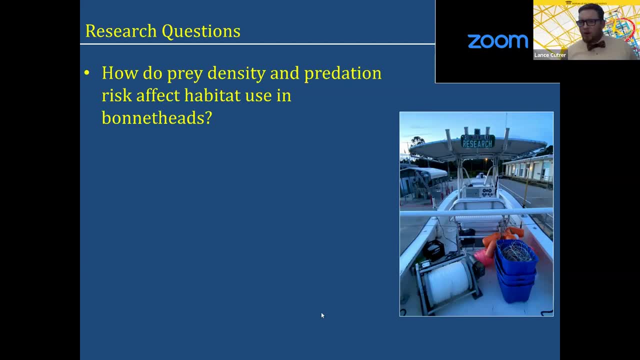 foraging is light, you know? Yeah, Well they're. they're pretty active sharks, right, So that they need that ram ventilation. They have to swim to breathe- Yeah, Right So they need to. they are ram ventilators, Yeah, Big, big uh energy um consumption with that, So they would need to. 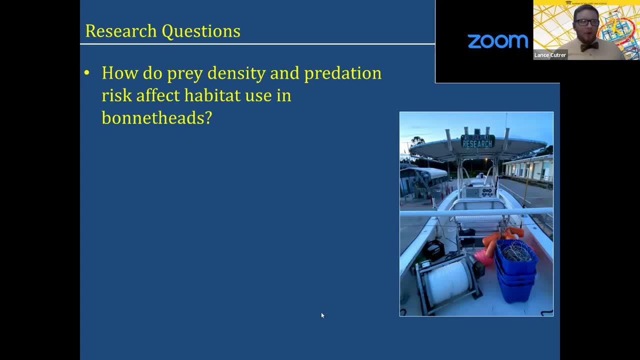 eat a lot. Right, We had a comment from from um a uh, a guest, saying that it's quite quite an expensive diet. The bonnet heads now, right, Yeah, Um are, are, are bonnet heads the? 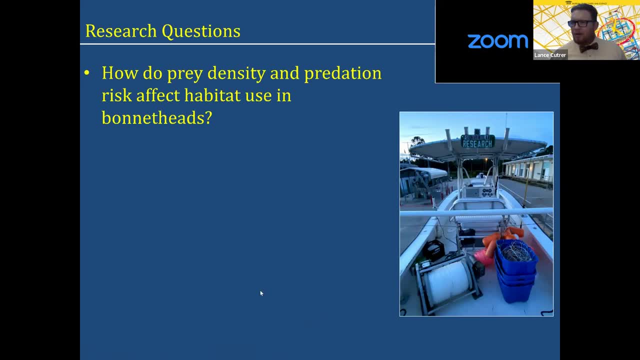 smallest of the hammerhead family. They are, I believe they are. There's been a couple, Um, there's. there's the wing head shark I'm thinking of. I believe bonnet heads are the smallest. There's just a couple of really obscure hammerheads that are- I forget how they stack. 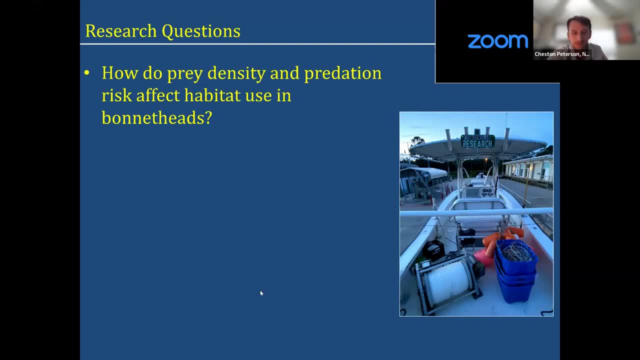 up size-wise, but I think bonnet heads are the smallest hammerhead. Cool, All right, Thank you very much. That was, that's a good question. All right, I'll, I'll, I'll uh meet myself. Okay, Thanks, Lance. So, um, I have a few sub. 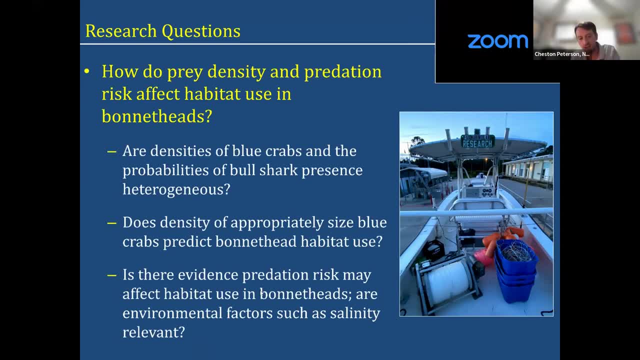 questions to that main question and that: uh, this is kind of all leading up to how. how can we answer this, this broader question? Uh, we have to answer these smaller ones first. So, um, one is our densities of blue crabs and the probability of encountering a bull shark. 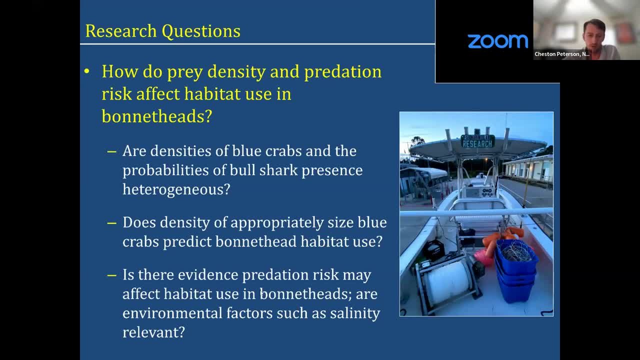 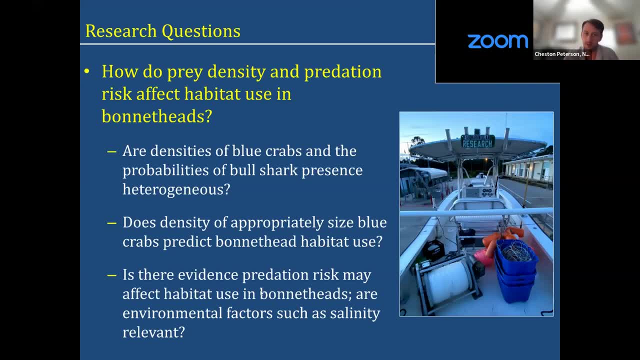 just completely even: There's as many blue crabs in the north as there is the east or the west, and same thing with bull sharks or not. Um, and then there's the density of appropriately sized blue crabs. uh, predict bonnet head habitat use, And that that's an important one, because we know. 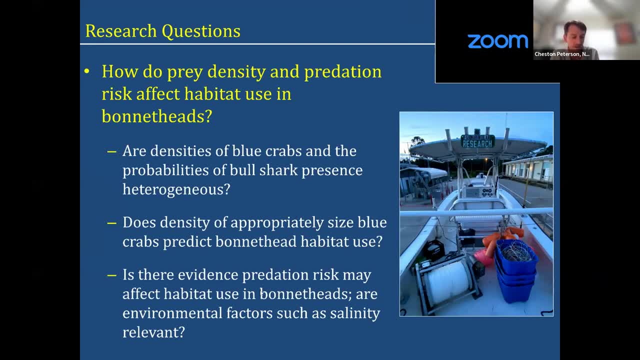 uh, that bonnet heads only eat, uh, uh, kind of a mid range of of crabs, Um, and there's especially a, a too big crab of a crab, So, um, so I corrected that in the data. And then is there. 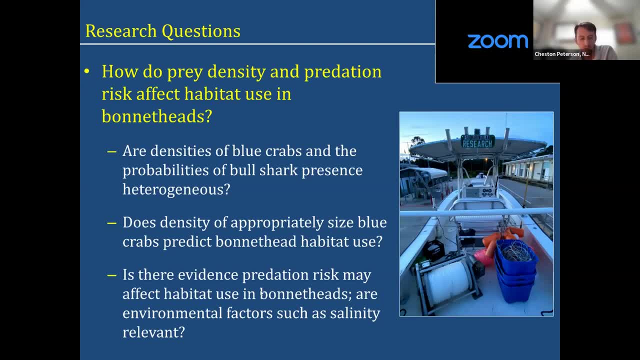 evidence that predation rates are more likely to occur in the north as there is the east or the west, And it's an interesting thing to note about this- How much risk may affect habitat use in bonnet heads um and how our environmental factors, such as salinity relevant. So we have to 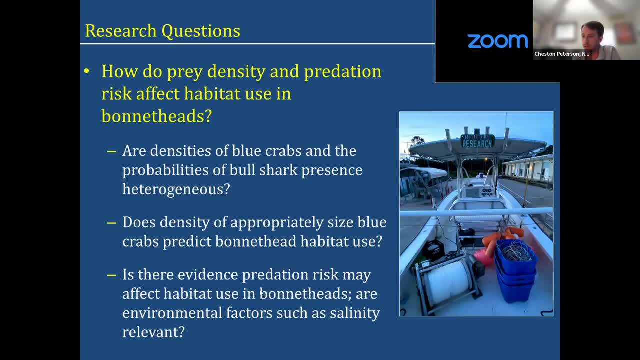 keep this in mind- and a river dominated estuary like this, there are some really intense um salinity fluctuations, uh, throughout the day, really, with the tides um major, major tidal effects, And so, uh, we have to consider that as a factor, since he, as you probably know, full. 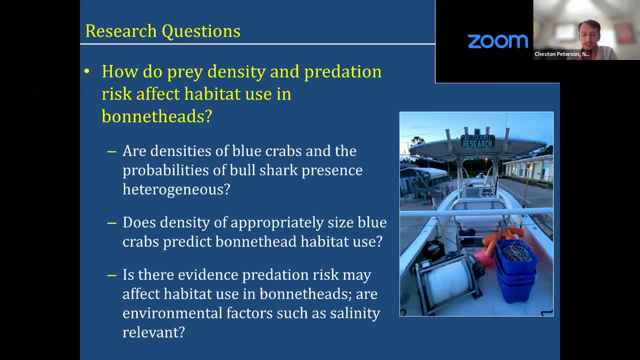 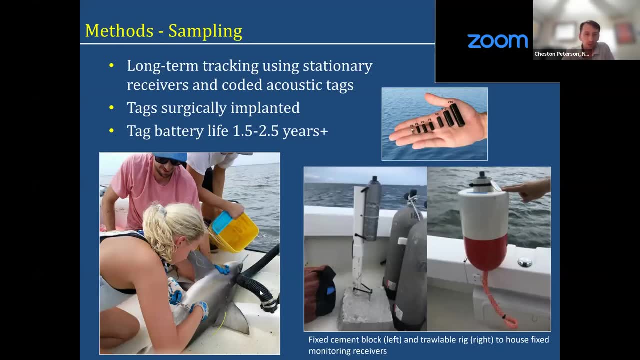 sharks um are able to go into fresh water and um, and so that's not as much of a factor for them. And so, just to get into how this works, we use long-term tracking with stationary acoustic receivers and coded acoustic tags, And so the image on the top right shows just the range of sizes- This is from a company called BIMCO- of their tags. 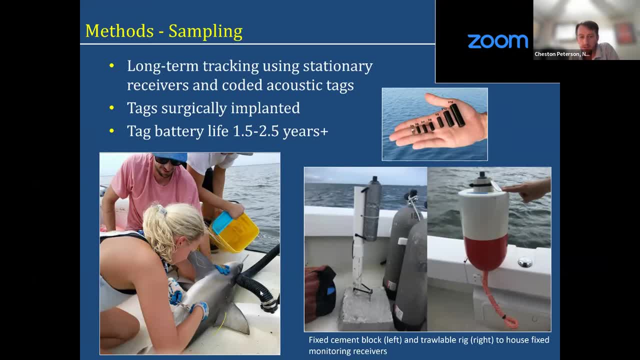 I use the two largest tags, the V13 and the V16, for bonnet heads and bull sharks respectively. And then the receiver, which I showed you a photo of earlier, is essentially just this black cylinder with a little node on the end. that's the actual antenna. 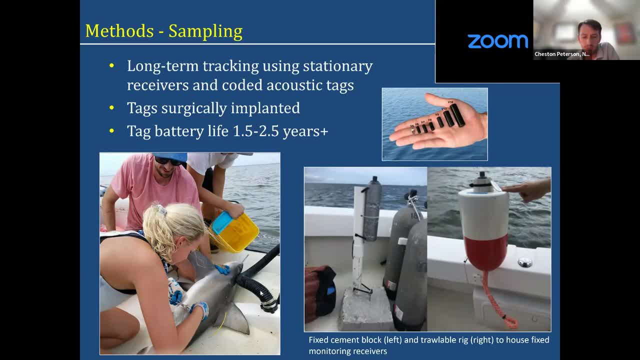 And then we had two anchor designs. One was just a thick cement block and a PVC pipe and that was moored to the bottom essentially, and had a buoy up to the surface So we could just go by. We could just go by boat and pick it up, pull it up on the boat and unclip it and download the data and perform maintenance. 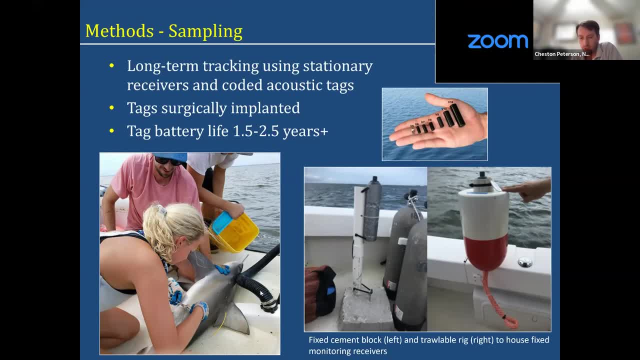 And then we had a fixed monitoring receiver in this bullet float or buoy that was anchored to the bottom. This was no buoy going to the surface here. We had to dive on these to retrieve them, And this was because of shrimp trawling, so we had to design a receiver anchor that could be trawled over. 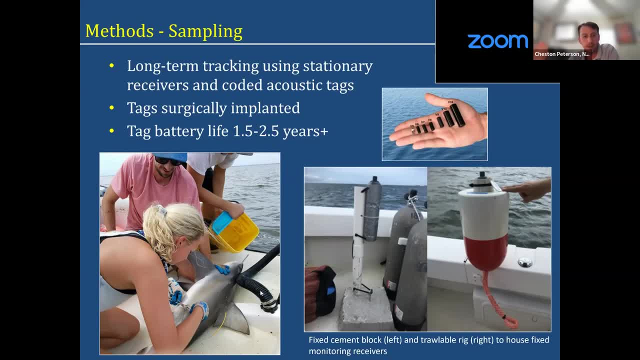 So the idea is that these basically just fold down as a trawl goes over them And then they pop back up. So the tags were surgically implanted. It sounds kind of rough, but it's actually really easy for a shark. 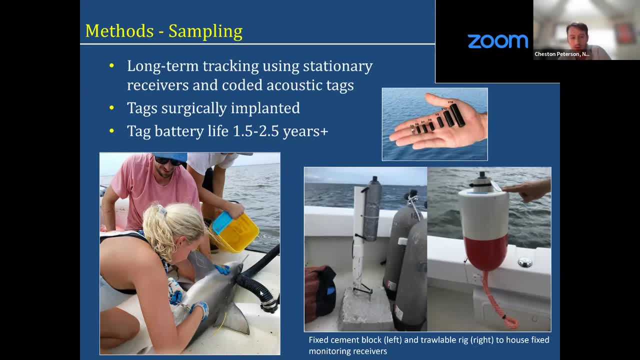 It's a small incision, one to two sutures, tops. We make that laterally or on the ventral side And then the tag. battery life was 1.5 to two and a half years. There's a lot of – you have a lot of control here when you design your tags from BIMCO. 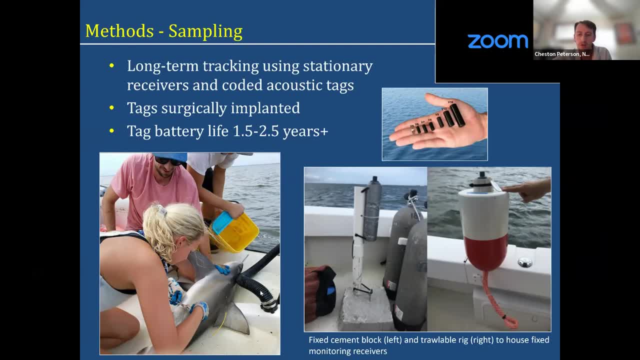 The tags can last up to 10 years, However – You have to compromise battery life and power And because of the high flow, high turbidity, meaning low water clarity, tons of suspended particles in Apalachicola Bay and that this was part of my graduate studies, so there is sort of a timeline on this. 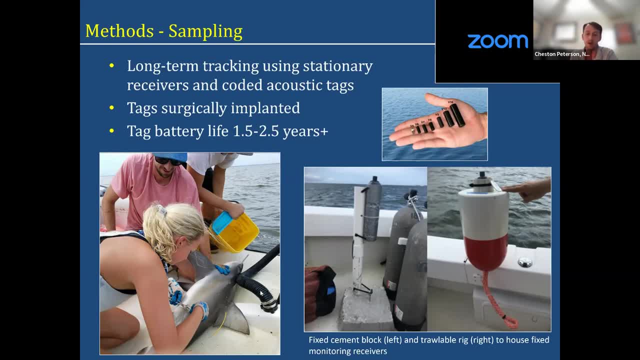 we optimized for shorter life tags with high power to maximize the probability that we would detect the animals. And so in that picture on the left, this was my student Ashley Doughty performing – tying the sutures. Early on when we were tagging we were like, oh, this is going to take a long time. 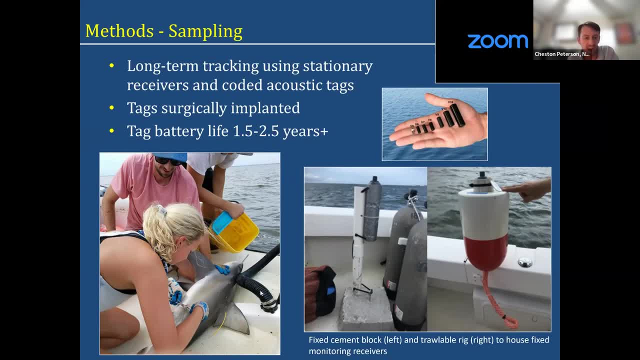 When we were tagging sharks I would do the incision and pop in the tag, But my clumsy hands full of adrenaline, like we talked about stress response, I turned it over to her. She had more dexterity with her smaller hands and was better at tying the sutures, so I let her do that. 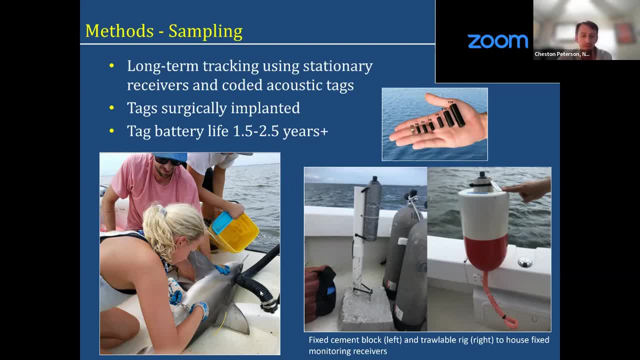 So you can see us doing surgery there. And then we've got an undergraduate volunteer just lightly pouring water over the shark. I prefer to use a bucket instead of a hose, because a lot of people love to like shove a hose in a shark's mouth. 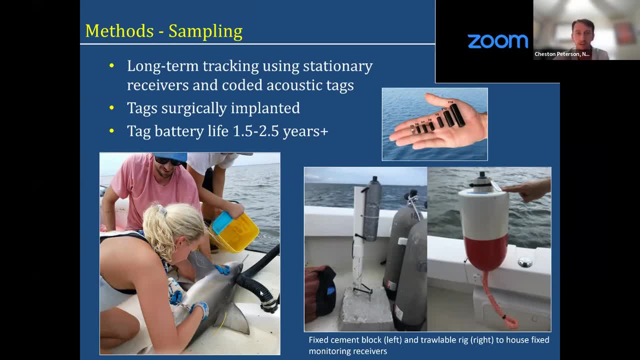 But if you don't temper that water flow, you can actually – I don't know if you can hear me, Ashley, but if you can hear me, I can hear you- water flow. you can actually damage their gills by just blasting water over their mouth and gills. 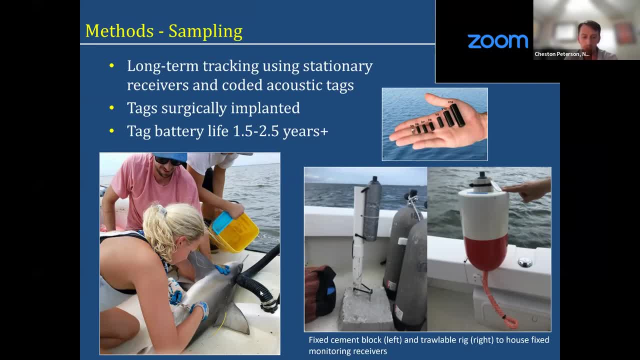 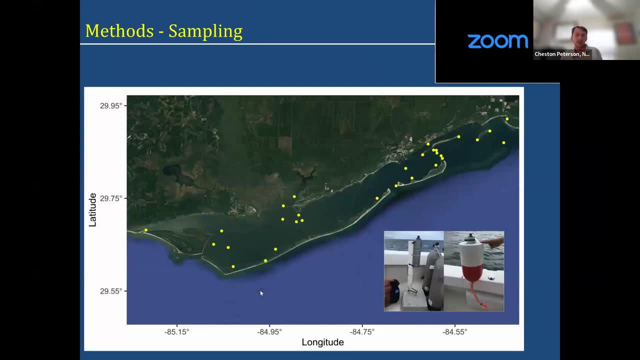 So we opt for just a little bit of flushing with a bucket of water to keep them aerating and keep them cool. And so this is our receiver array. Every yellow dot was a receiver in Apalachicola Bay. You can see that they're spread pretty wide. 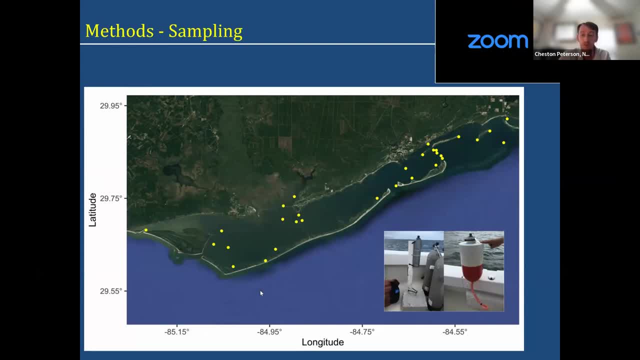 This was a collaborative project with a lot of goals, So this was not specifically designed by me for this project, So it kind of had to make do with what we had. But that's what the array looked like And if I don't have any questions about this part, I wanted to give a chance just in case if there are any questions on the methods and sampling. 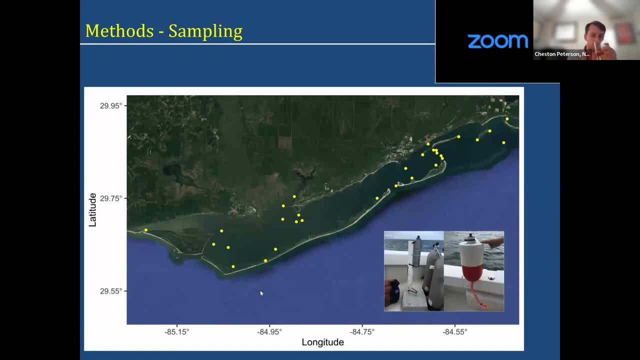 But otherwise I'll move on to some of the results. I should say, if you're curious –, Tell me again. those yellow dots are where you had all the acoustic receivers. That's where the receivers are. yeah, Right, Yeah. 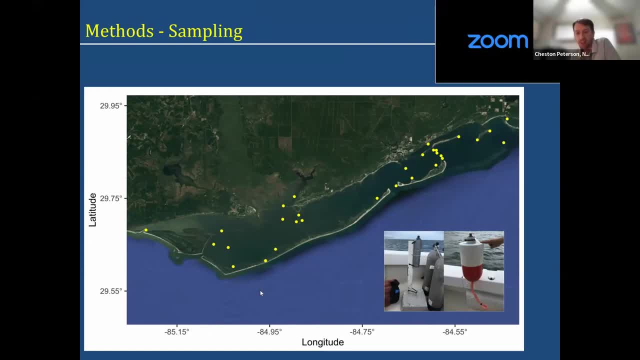 How did you go about deciding where to put them? That was probably a year of going back and forth with other scientists optimizing habitat coverage, So we tried to prioritize monitoring. you know soft bottom habitats, seagrass habitats, and then oyster reefs or hard bottom. 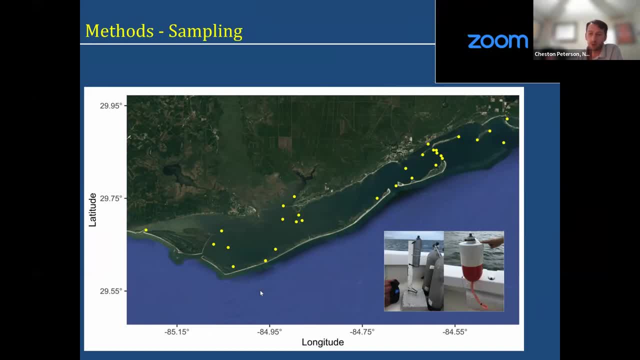 We also tried to cover the inlets. This was the array. at the end of the study, There's about, I want to say, a dozen receivers that did not survive And were either stolen or, more likely, missing. Unfortunately, our study, when we deployed the array, this was before Hurricane Michael and Michael did a number on us, unfortunately. 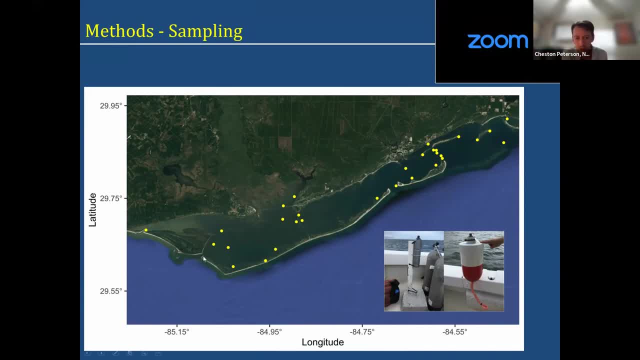 So, for instance, if you can see my cursor in West Pass, we actually had two receivers down here that were yanked out of the bottom never to be found, And so essentially prioritizing habitat coverage, trying to cover the inlets and outlets to monitor immigration. 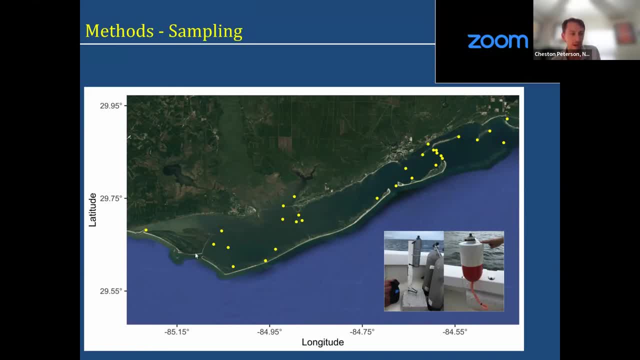 And then essentially just trying to compromise with other scientists, as you do, to meet everyone's goals and try to design something that'll work for more than one species. Right, Yeah, And so another thing, that's: How many tags did you get deployed? 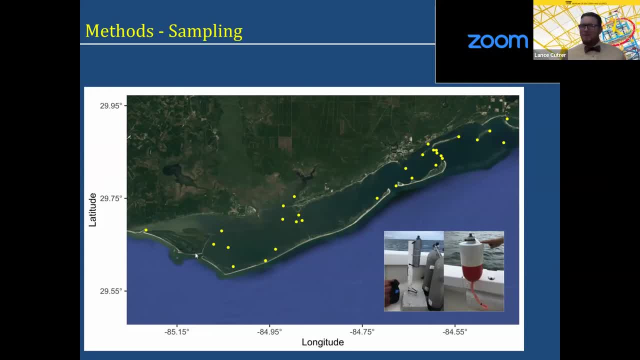 I will get to that. Okay, great, I'm cutting ahead. Yeah, I'll get to that. There were, I think, 32 receivers in the end And yeah, I'll get to tags. One thing I should have mentioned is, alongside this work, we had two other companion projects. we had 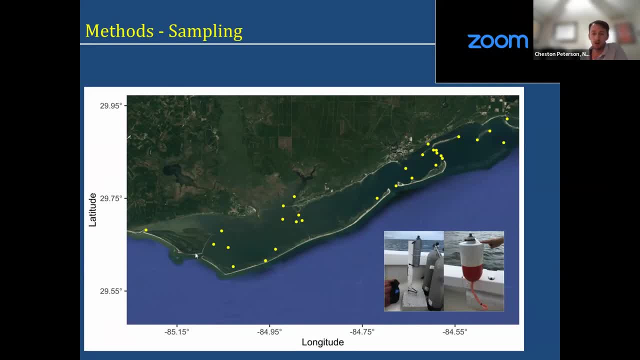 I was doing fishery independent surveys, so essentially doing longline and gillnet surveys for sharks, which provided a lot of our tagging opportunities. And then I mentioned my student. Ashley was doing an undergraduate honors thesis that she just got published a few weeks ago, actively tracking bonnethead and bull sharks. 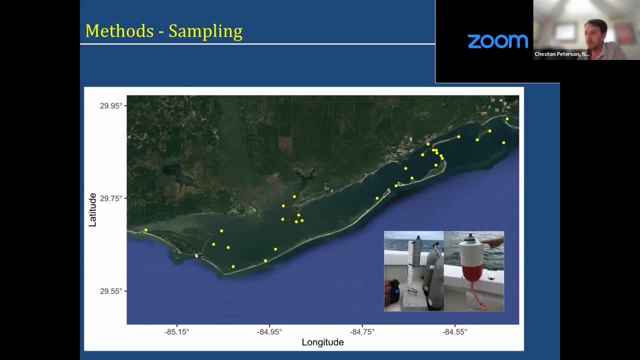 And that's when we actually lived on the boat. We tracked a shark for 52 hours and followed it around with a similar but slightly different tagging technology, And those provided a lot of tagging opportunities as well. So for some of these animals, we actually double tagged them with active and passive acoustic tags, followed them around for two days and then had at least one or two years of data after that as well. 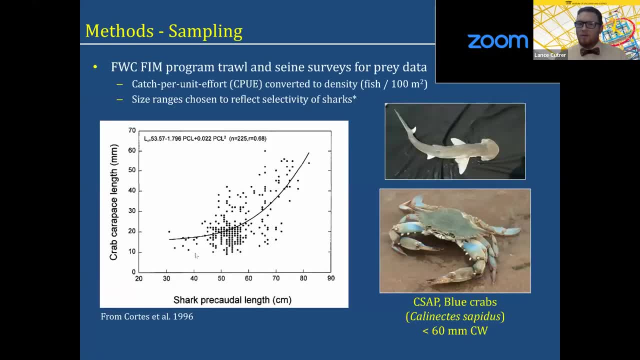 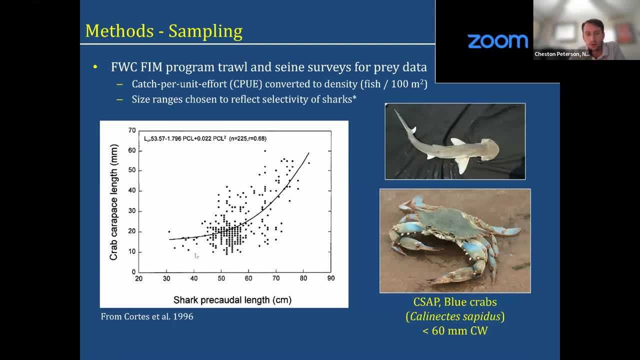 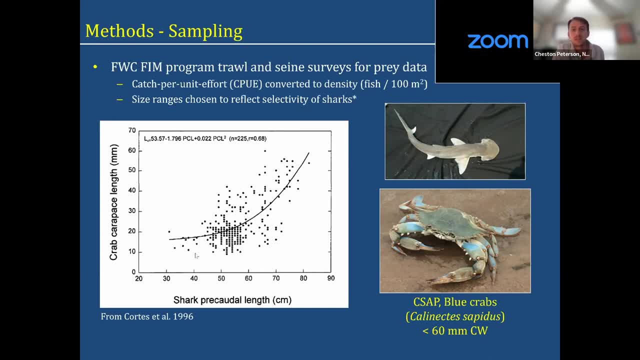 the water or the spatial coverage. So here it's: fish per 100 meters squared of trawling coverage. And then the size ranges were chosen to reflect the selectivity of the sharks, And so this is a figure from Enrique Cortez's paper from 1996 where he looked at, and this is specifically 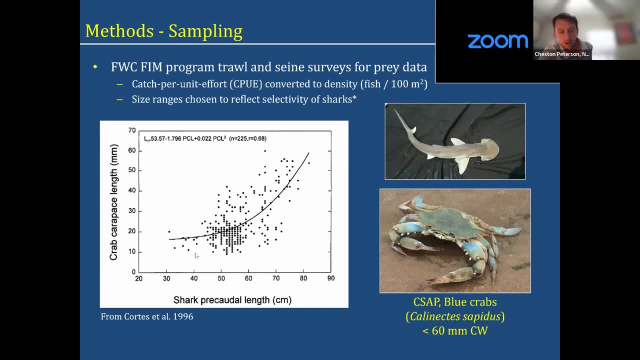 blue crabs, shark pre-caudal length, which just means the length to the base of the tail and then crab carapace length, And you can see there's kind of a middle ground there where the smaller and kind of medium-sized crabs are more popular for the bond heads. And so to get to Lance's question, I was able to tag 20 bonnet heads and 20 bull sharks. That actually took three years- 2018, 2019, and a little bit of work in 2020.. We were lucky to be able to continue our work throughout the pandemic. 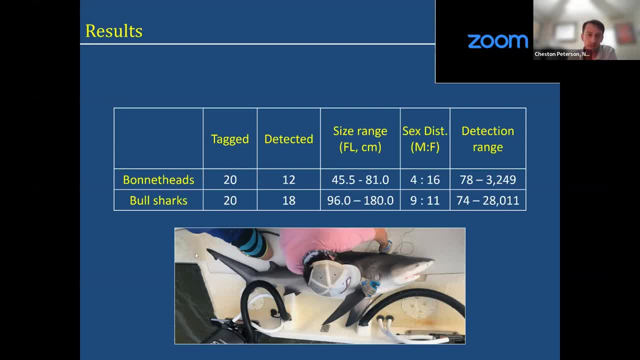 thanks to the wonderful staff at the FSU Marine Lab, We only detected, however, 12 bonnet heads and 18 of the bull sharks. You can see the size range here. So we tagged some pretty small- these are in centimeters- small- bonnet head sharks, so probably. a foot and a half to two and a half feet long or so. Our sex distribution was heavily weighted towards females. We catch a lot more females than males here, for some reason, And we had as few detections as 78 for one individual and as many as over 3,000.. The bull sharks were a little more. 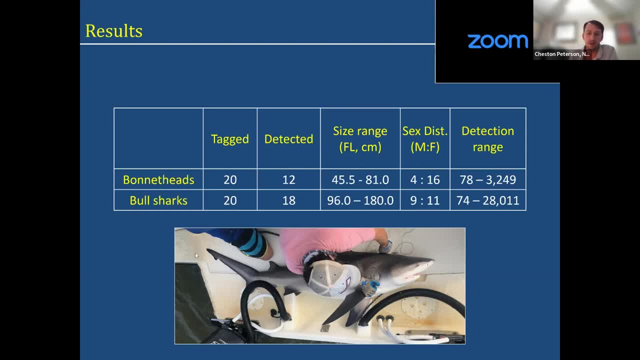 productive in terms of the data. So their size range was right at a meter to 180 centimeters, So probably coming up on five and a half, almost six feet long. for the largest Sex distribution was almost even at nine males and 11 females. We had a similar minimum detection number of 74. 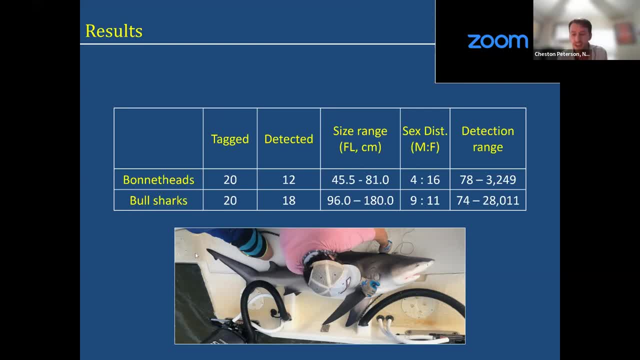 But for some of our bull sharks we detected them actually over 28,000 times. Now the tags are pinging every 20 seconds or so. So those thousands of detections, if they're kind of patrolling around a receiver and they're not, they're not going to be able to detect them. So we had a similar 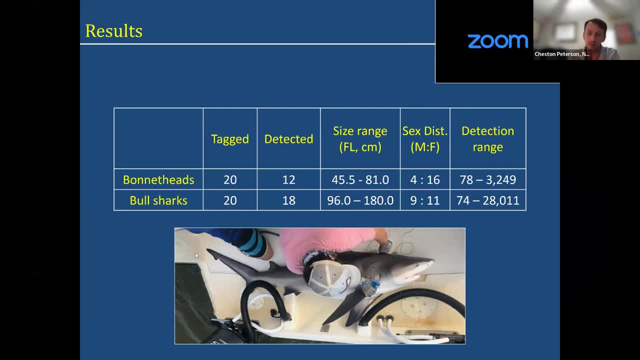 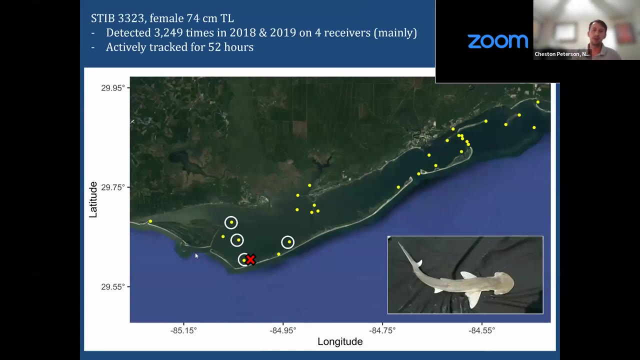 number of bull sharks in that habitat and hanging out for hours, and they're going to really rack up those detections. And this is just another photo- kind of a weird perspective- of me with one of the last bull sharks that we tagged, And so I have a couple maps here showing some. 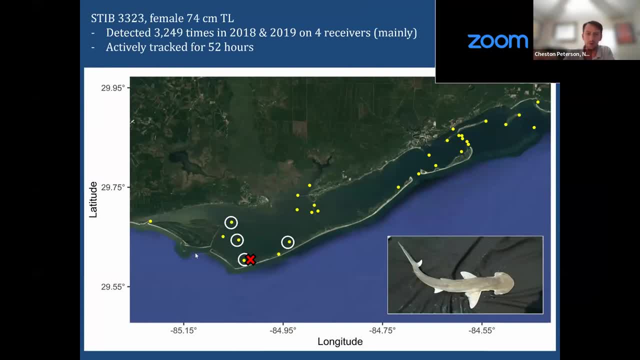 individual sharks And I did this just because I wanted to show you kind of what we would expect from one individual. You know, obviously the goal here is to study a group of individuals and make some broad conclusions about what they may do as a species or a population. But just to give you an 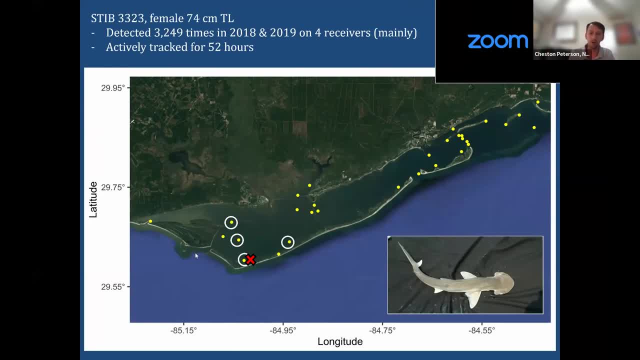 idea of like: hey, we tagged, you know, stib number one. what did it look like? How does it compare to some of the others? And so this is tag number 3323, which is a 74 centimeter, about three. 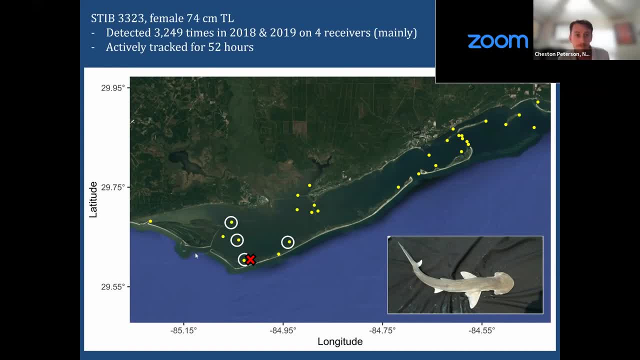 what would that be? Two and a half feet, two feet, bonnet head. And she was detected over 3,000 times in 2019, mainly on just four receivers, And she was also actively tracked So that red X marks the. 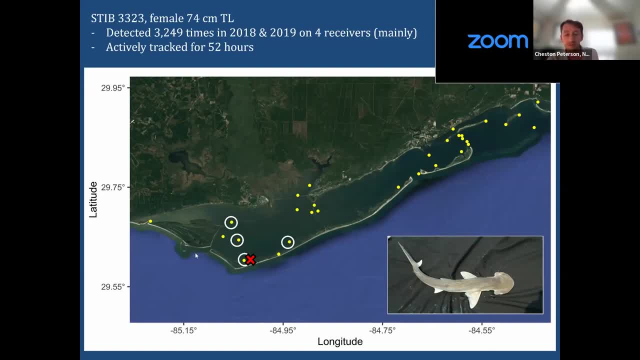 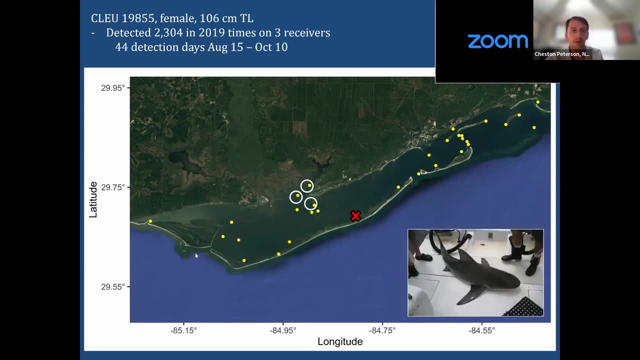 location she was tagged, And so you can see that for this bonnet head there are a lot of detections, but really only on that one set of receivers. And then we had bull sharks. that kind of showed a similar pattern where we had a lot of detections on just a few receivers like this: 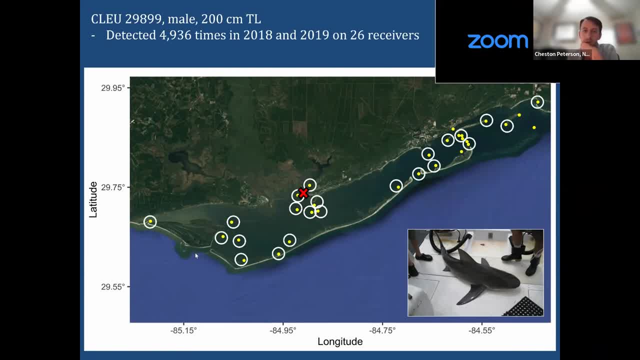 Or we had this large male that was a 200 centimeter male that was detected on almost every receiver in the entire system, 5,000, almost 5,000 times, And yeah, so you can just kind of see the idea of what. 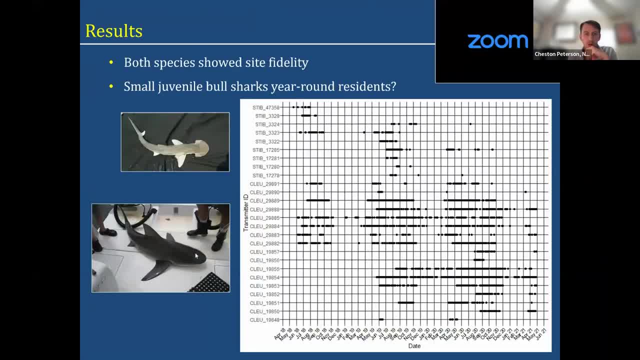 the difference here. So one of the things that we like to look at when we use this acoustic data. we kind of answer some other alternative questions And one of the things that I was hoping in this study is that sharks would be coming back year. 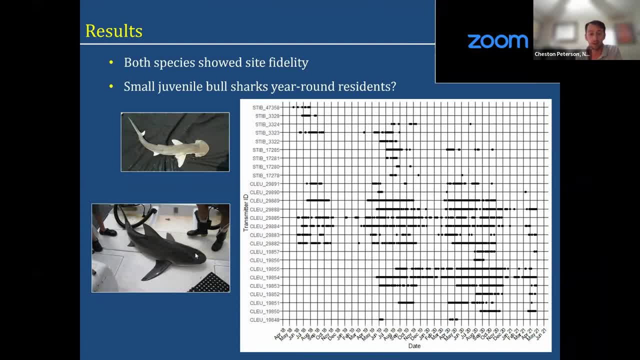 after year, so that if we tagged them in 2018, they'd come back in 2019 and we'd get a whole other year of data from them. And for the most part, that was true. We had site fidelity in both the bonnet heads and the bull sharks, And so this is just a plot. looking at, you've got the months. 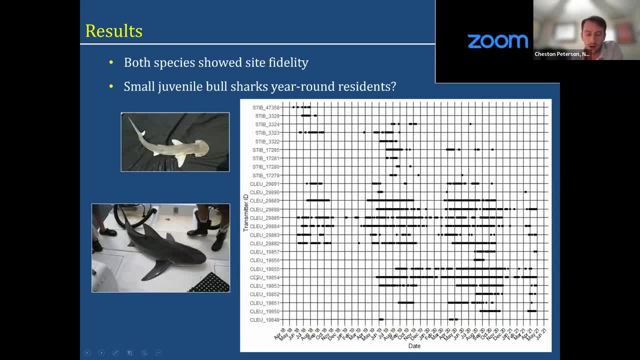 and the year on the X axis on the bottom, and then the sharks and their IDs on the Y axis And the dots are just when they were present, And so you can see that you've got these kind of like pulses here in the summertime when the bull sharks are showing up, And what's really interesting is for 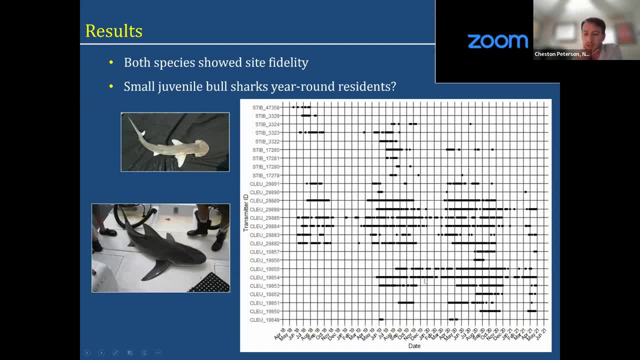 some of the juveniles, the winter between 2019 and 2020 was rather mild, And so it appears that they may have actually been a resident year round, And so they may only migrate or emigrate out of the bay when temperatures get too low. 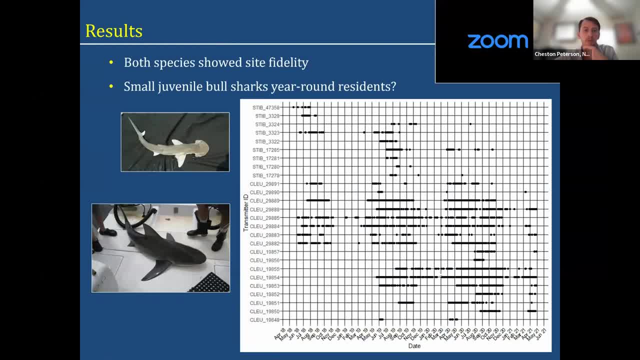 And if they don't get too low they may not have to, And so that's kind of that's the first thrust here, of our basic results, how you know kind of the goals of the study, our methods and our main. 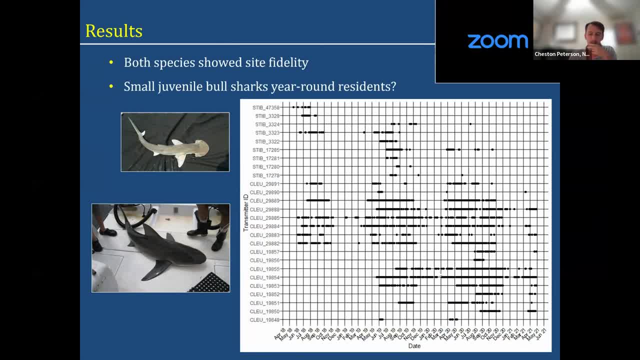 research questions, And so I'm going to start talking about the main analysis now. I'll talk about two analyses. One are network analyses, which is a way we just look at how each species use the array data, Which receivers they move to and from, and in what order. which receivers are the most popular. 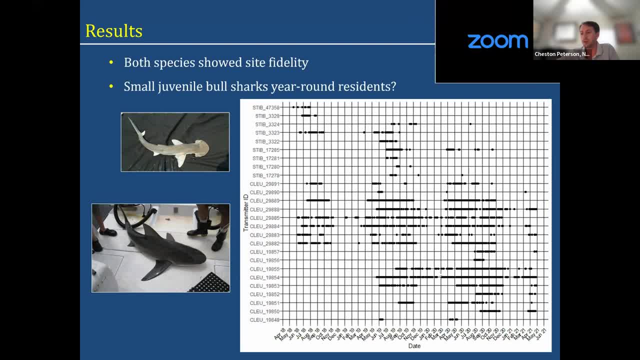 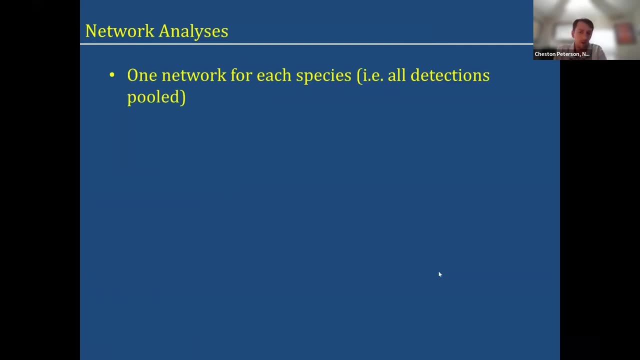 And then I'll move on to some statistical modeling where we actually tried to quantify some of this stuff and get at our main question of: was there an effect of predator and prey distribution density on the bonnetheads? So the first thing I'll talk to are network analyses, where we have one network. 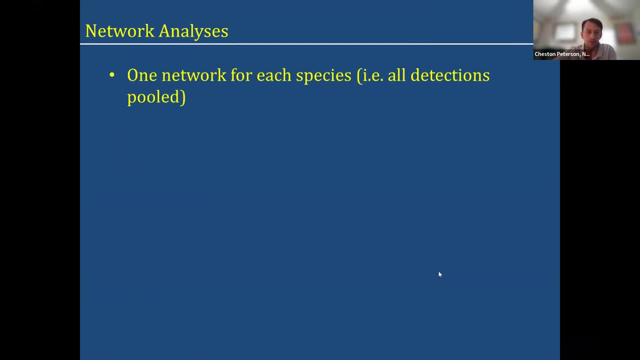 for each species. So we pooled all the detections for each individual. We had to bend the detection, so we used only the summer season, from May to August, And then detections were bent in six hours just to kind of condense the data. because you get so much data from these tags And then we 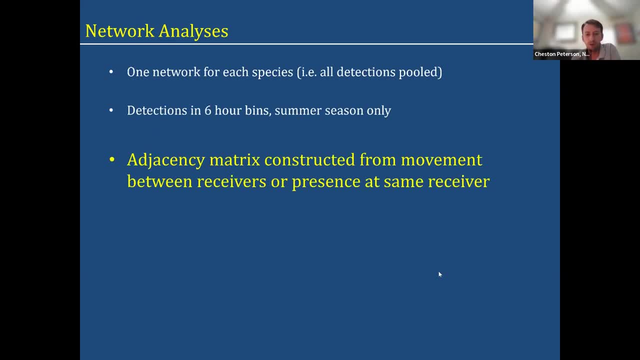 constructed an adjacency matrix for movement between receivers or presence at the same receiver, And so an adjacency matrix is basically taking pairing every receiver with every other receiver and looking at movement between receivers, And then we also looked at the movements from receiver A to receiver B and how many times that happened And that creates a whole. 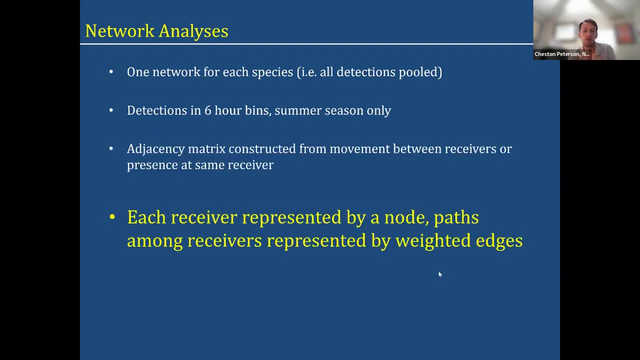 matrix of data that we use in the network. Then each receiver is represented by what we call a node- It's just a circle on the plot, And paths among receivers are represented by weighted edges, which is a fancy way of saying a line drawn from each node And the thickness of the line. 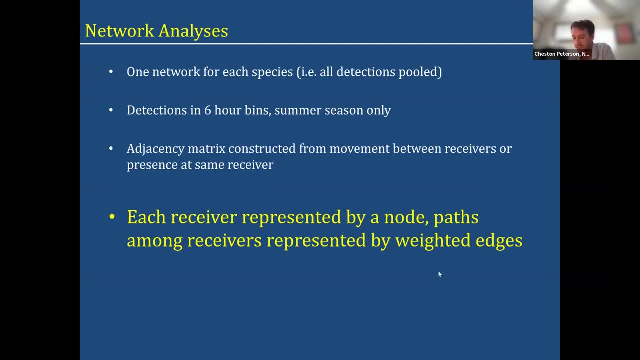 represents how much that path was used, And so I should preface this. network analyses are a way of looking at the data that we use in the network, And so I should preface this network. network analyses are a way of looking at the data that we use in the network, And so I should preface this network. 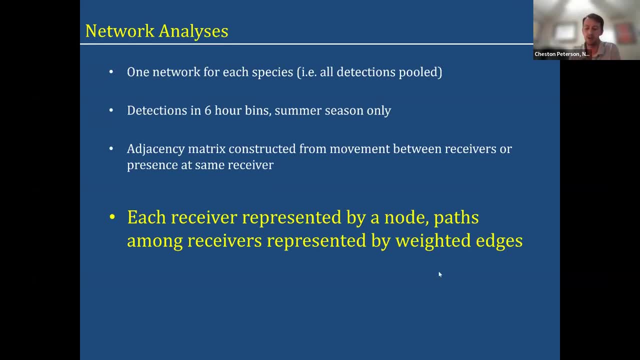 analyses did not originate in ecology and these are being adapted And so you can see, some of these kind of the terms we use aren't really intuitive, especially for a biological question. But that's the background there. And then we calculate a couple metrics to describe the networks, The 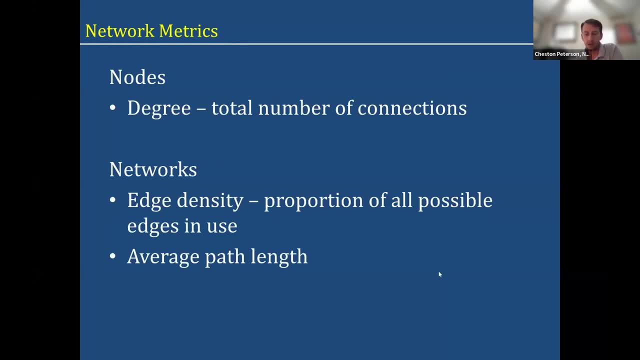 metrics are the nodes, the degree, the total number of connections. Edge density is the proportion of all possible connections or edges in use. So that means, of all the different combinations of paths, how many were added, how many were not added and how many were not added. And 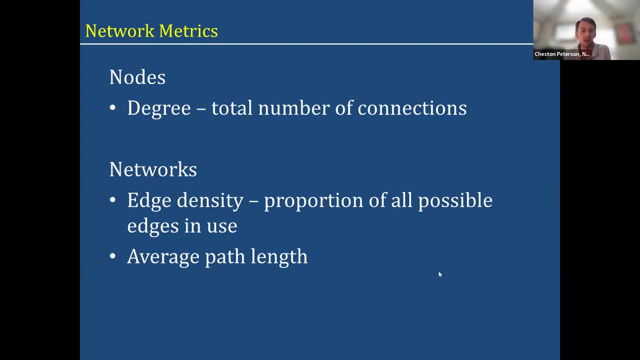 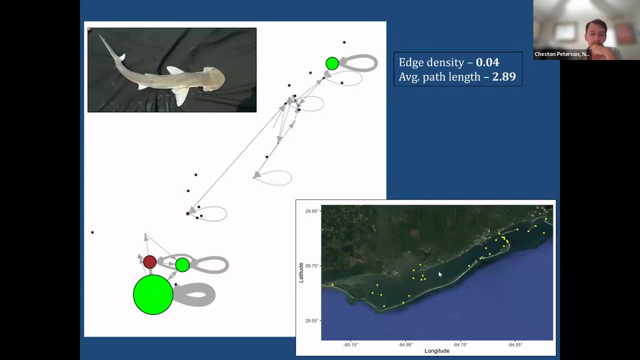 how many were actually used by those species, And then the average path length. And so here's our first plot of a network. This is for the bonnethead sharks, And so, just to orient you, the access of the array is kind of tilted. The network seems to just have to do that Looped arrows. 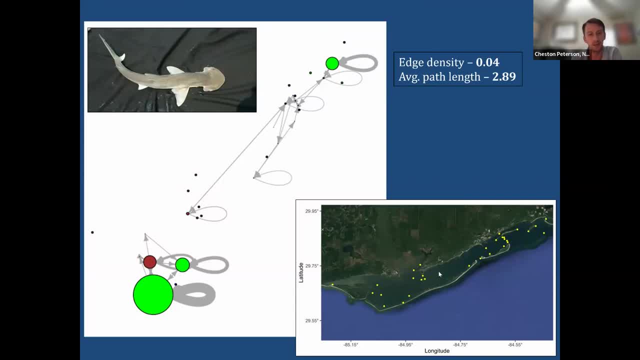 mean that in a six-hour time, then in the next six hours that shark was still there. Otherwise you can see some of the paths that they took. The larger the circle means the more common that node was used And I did color code the. 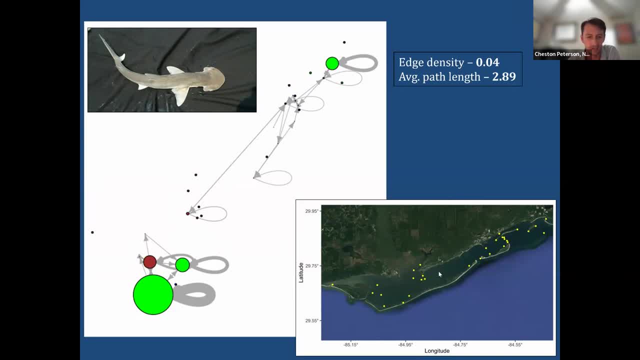 nodes. So the green nodes represent seagrass habitat, which the bonnetheads tend to really like. The brown nodes represent mud And you can't see all of our inlets are represented by a blue color that you can't really see. So the edge density was 0.04, which means 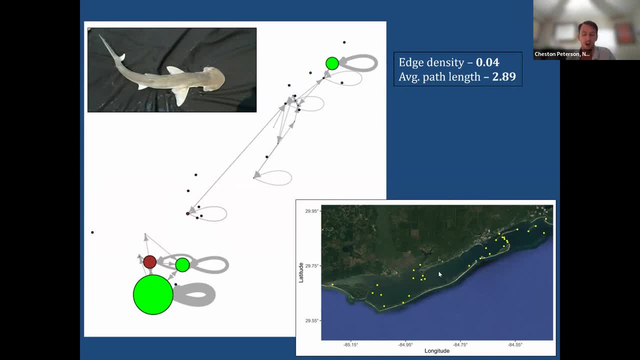 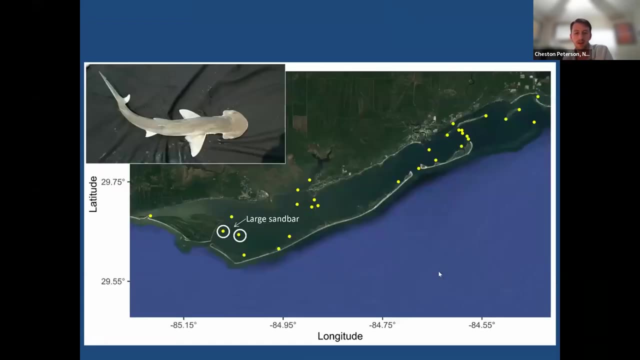 the bonnetheads were using very little of the possible space in the array. They're really only just kind of honing in on these couple areas and then making these little sort of foraging trips to the other sites, And so one thing I'd like to point out is there's a big sandbar of these two popular 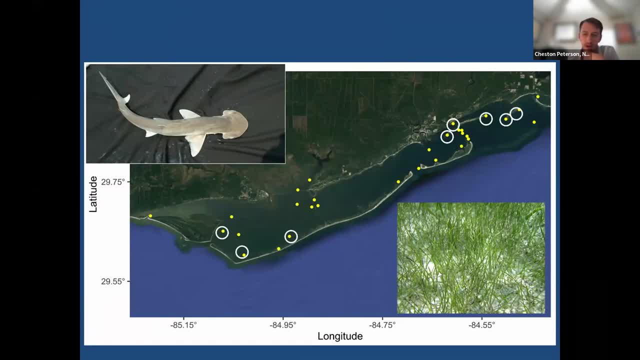 receivers here And then every receiver that I've circled are. these are receivers targeting seagrass habitat. So, as I mentioned, they really were. they picked up a lot on these receivers because they're in there foraging on seagrass or not on seagrass foraging. 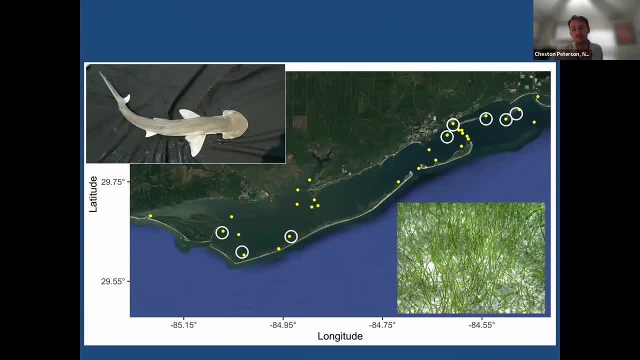 on blue crabs in the seagrass. That's a whole nother can of worms for some of you. folks think that bonnetheads are riverous and grazing on seagrass And I have my own opinions about that And we can talk about that later. 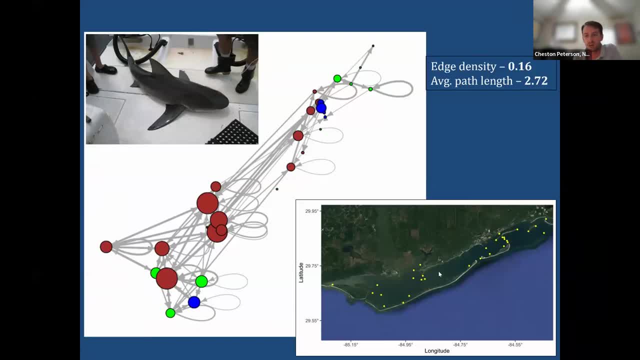 Then for the bull shark network you can see their edge density was 0.16.. So they used way more of the whole space in the array. You can probably just see that in just the nature of the plot where you don't have one or two really giant circles and a bunch of 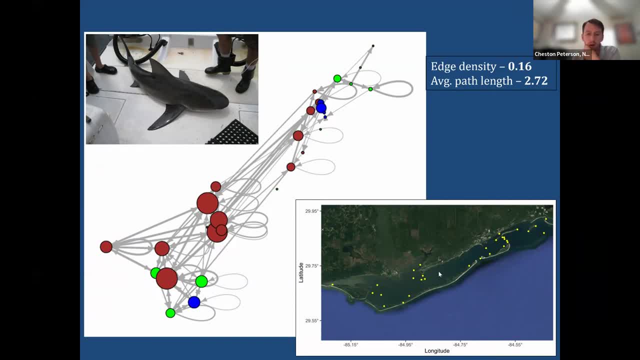 teeny, tiny ones. It's more even, And so they are going all over the place. They're going all over the place and they're using a lot of the possible paths between receivers, And some of this is intuitive, because bull sharks are a larger animal, So we can expect that. 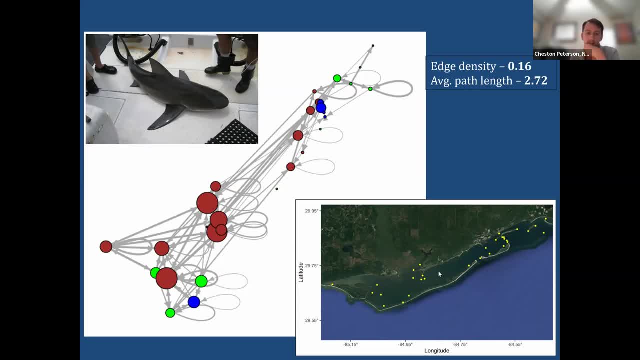 they move more, just in terms of body length and everything. but this was still really interesting And so just to remind you, to compare the bull shark and the bonnethead networks. So can I ask, let's go back for one second, Just to make super, super clear. I want to. 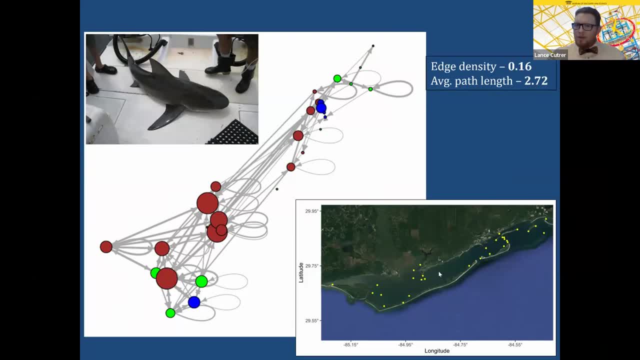 understand everything really well. So each. so we look at the map down here on the bottom right And each of those yellow dots is an acoustic receiver. So then we take that to the plot of data. So each one of those circles: the bigger the circle, the more frequent that they were there. Is that right? 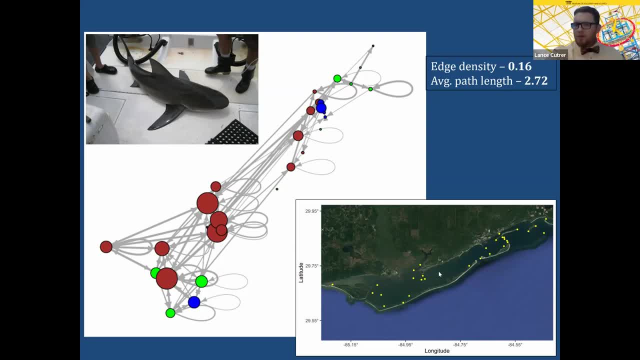 Correct, Okay, But each circle and the ones that are just simply black dots they maybe they didn't go to So so it kind of is associated along the same, The same axis here. So so the little the red dot on the far left side over here represents. 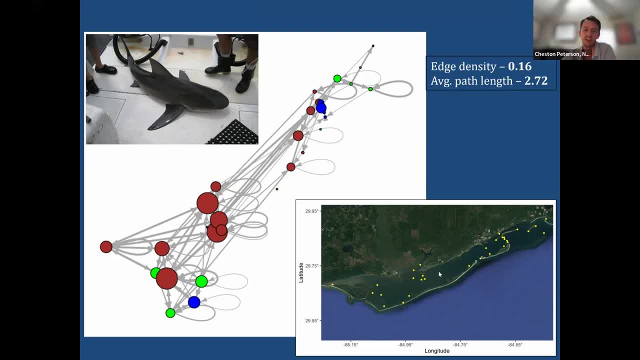 the same If you look on the map at the very left side over there, right? Okay, Yeah, Lance, that that's I'm not I, I, I tried so hard to get these plots to use the latitude and long data just to twist it, And I, I, I really struggled with it And so I eventually. 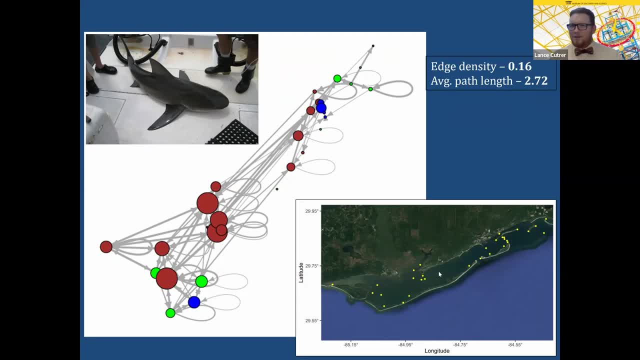 just went with it. I said, yes, I get it. I get it, It's, it's a good, it's a good way. It's just twisted up a tad, but yeah, you're right. The the, the red circle on the farthest. 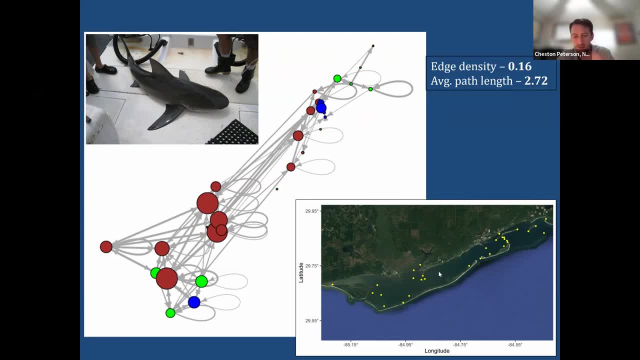 left when you're looking at the plot is the Western most receiver in the map Right. Okay, Yeah, That makes sense, That makes sense. And so the thicker the line, the more commonly they were that that shark was was there. right Loops represent stay. there and straight line represent them going from 1.5 to 0.5.. Yeah, Yeah, Okay. So so there's that, that, that, that that that, Yeah, Yeah, Yeah, Yeah, Yeah, Okay. So we, we, we're kind of just jumping out, But now you're. 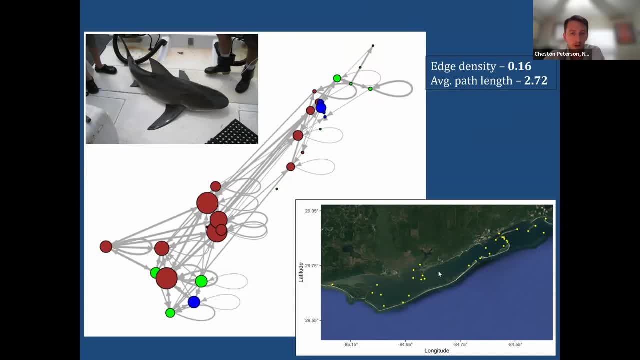 point to another. exactly that makes sense, and so those thicker lines basically mean that that's like, that's a, that's a common path. now, there's some nuances to this. what it really means is: we detected. that's the order in receivers. chronologically, they were detected on, and so 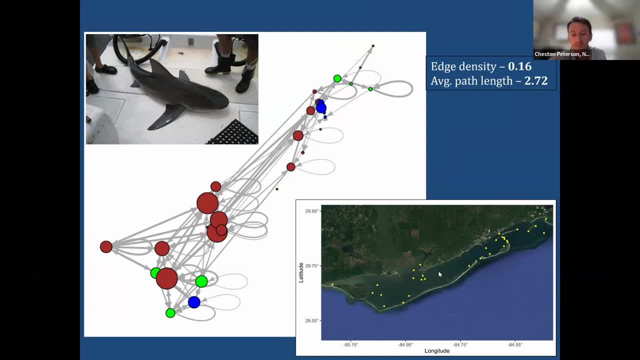 technically, you know, i'm sure bullshark movements aren't all these straight lines from all our perfectly arranged points. right, it's just showing you. you know the order that they showed up in, so we don't know what they're doing between one or the other, but, um, it still gives us a really good. 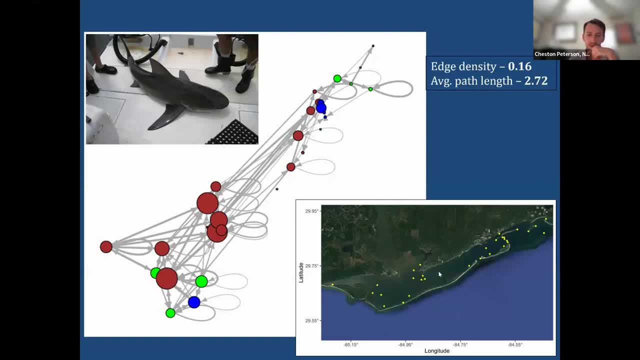 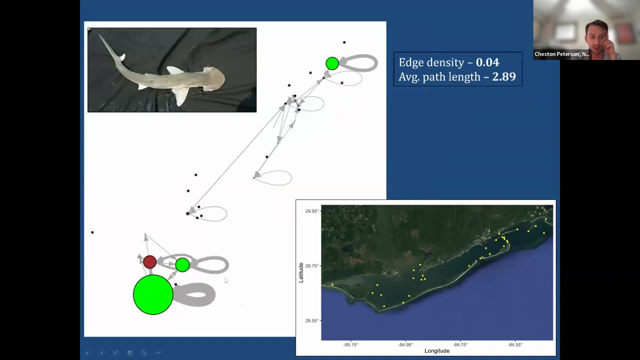 idea of um, of what they're doing, and and what i like that you mentioned is seeing those loops when you know they're staying in the same places, and so that was especially true of bonnet heads, like this giant kind of fat um loop coming off this main receiver that's in in pilot's cove it's. 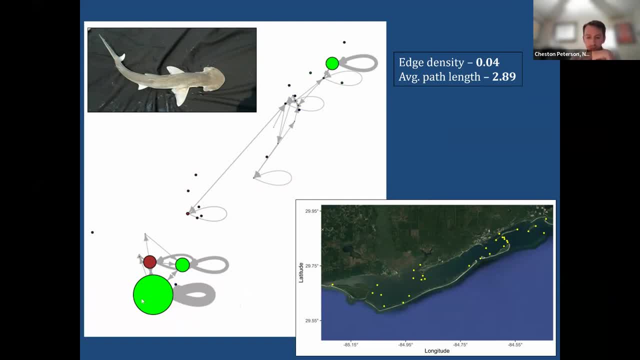 this beautiful seagrass bed. it's quiet. it's, uh, protected from much. the rest of the bay, there's a ton of stuff in there, um, and the bonnet heads really seem like that. that. that was true of any of the bonnet heads that were on the western side of the bay. 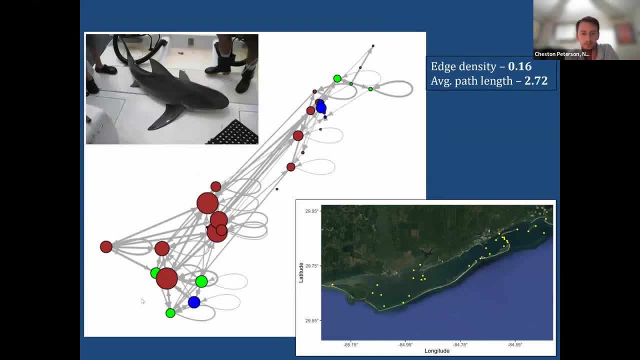 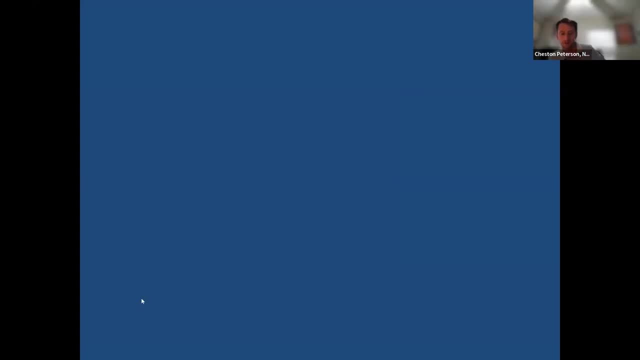 they really liked that habitat, cool, okay. so another little breather here and i'll get into um some, some of our statistics and modeling, so i've included everything. so you can see it. i'm not going to talk about it all in detail, um, but i'll try to explain um how we did it, what we put. 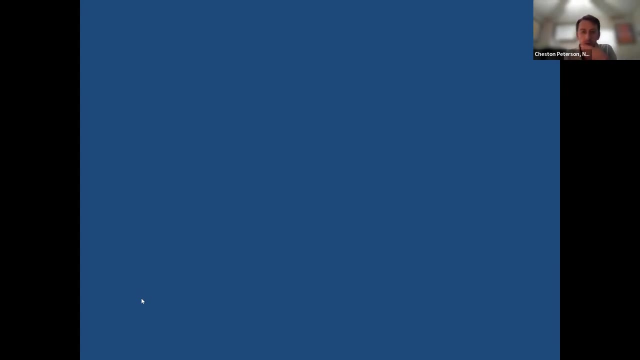 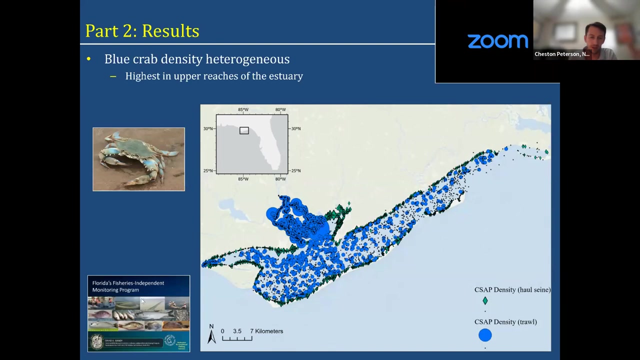 into the statistical equation and and and what we took away from it. and so, um, one of the answers to the sub question before of: are blue crabs heterogeneous or homogeneously distributed? meaning are they, are they evenly distributed or are they patchy? and they are definitely patchy or heterogeneous. so this is just a plot of the fem data and you can. 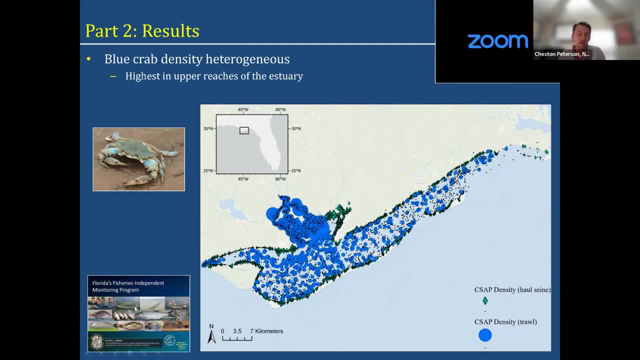 see um just florida's uh fwc's fishery intermittent independent monitoring program. there i'm led by dave dandy and apalachicola um, and so we we can see very clearly that there's these. you know, blue crabs are heavily distributed up in the northern reaches of the bay um, they occur throughout the. 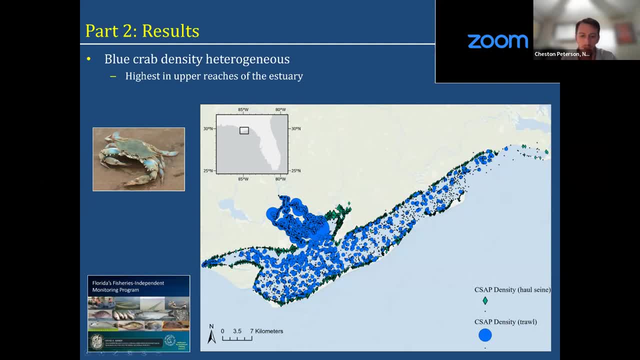 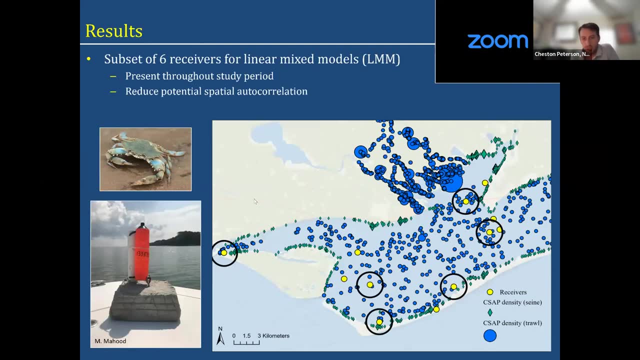 bay. obviously they're along the coast and everything um, but you can see that it's not perfectly even um. and so, to look at this, we took a subset of our data where the bonnet heads um occurred on the western side of the bay, uh, to kind of control in that space. so we took a subset of 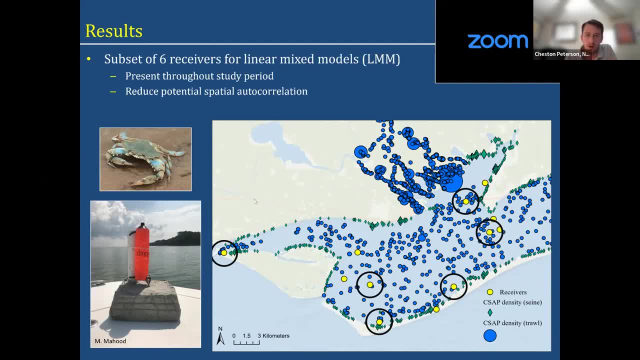 six receivers, um, and we used a an analysis called linear mixed models, and so we chose these receivers because they were present throughout the study period, so they were never removed by the hurricane, they never had to be replaced, and we also chose receivers that were separated fairly well from one another, or at least representing different habitats. so 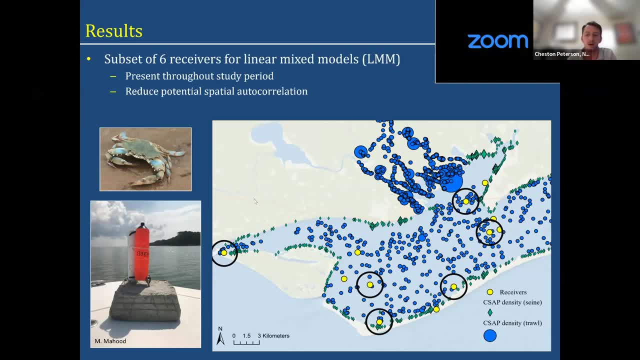 we didn't have any spatial autocorrelation, which means that, um, when you know, say, for instance, this patch of three receivers, we could have used all three, um, but when a shark's in there, they're more likely to be detected on the other receiver. and so we chose these receivers because they were present. 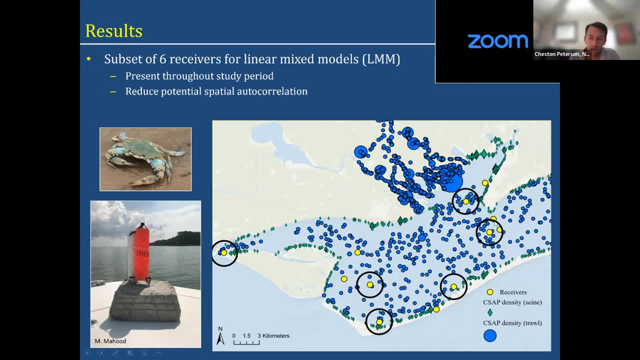 throughout the study period. so they were never removed by the hurricane, they never had to be removed by the hurricane. so we chose these receivers, um, just by by the nature of being there at the first. so we didn't want to um, to kind of weight the statistics too much. 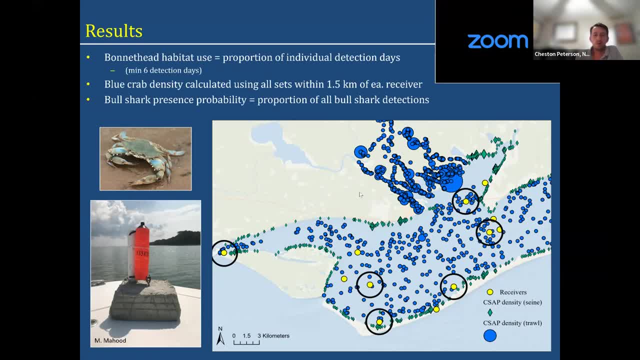 and so to quantify bonnet head habitat use we used the proportion of individual detection days, and they had to be detected a minimum of six detection days. and then blue crab density was calculated using all sets- fwc sampling sets- within 1.5 kilometers of each receiver. that was designed to essentially look at the detection range of the receiver. so 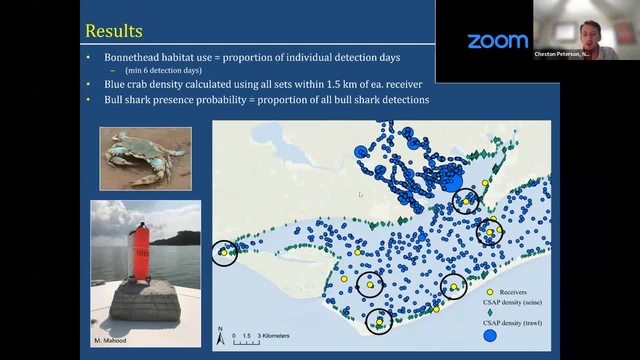 one thing i didn't mention is that we do range tests on all this. so when we deploy the gear, we we manually set out tags just in little mesh bags, at regimented distances, sequential distances away from the receiver, to look at our detection range and our detection probability. so we have an idea. 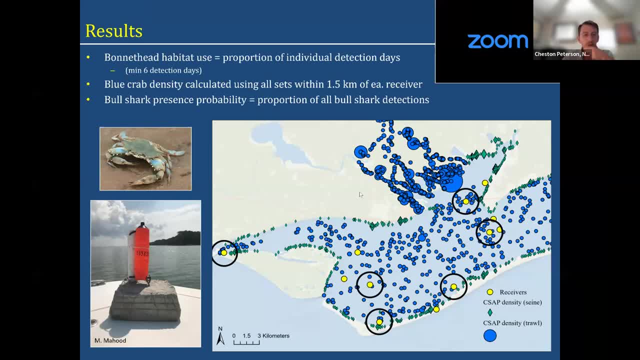 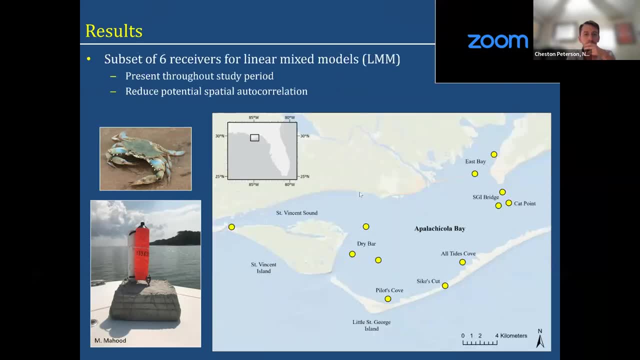 of what we're kind of starting with, if you will, um, and then bull shark presence probability was the proportion of all bull shark detections at those receivers, um, and so let's see, this is just showing you the names of some of our receivers, so i'll walk. 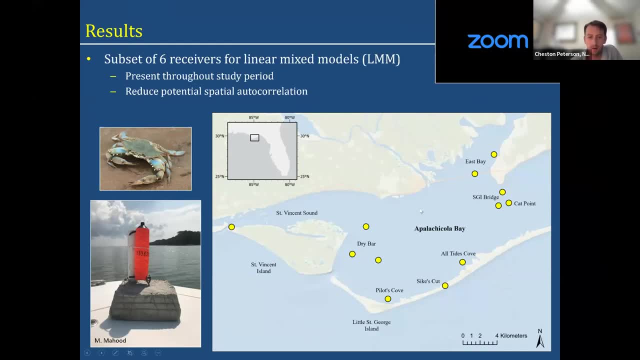 through this just a bit. this is an um apalachicola bay proper and so, uh, we had all tides, cove sykes cut and pilot's cove. then we had dry bar. this is called indian pass or saint vincent sound, east bay, st george island bridge and cap point. 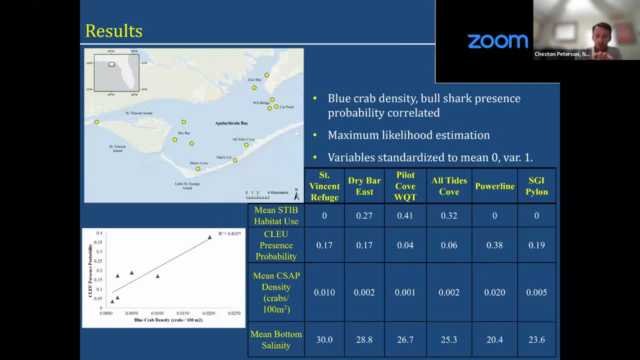 and so these are some of our- uh, our- results here from the model that i'm not going to talk about too much, but blue crab density and bull bull shark presence were correlated, and so in this plot in the lower left, i have blue crab density on the x-axis and the probability. 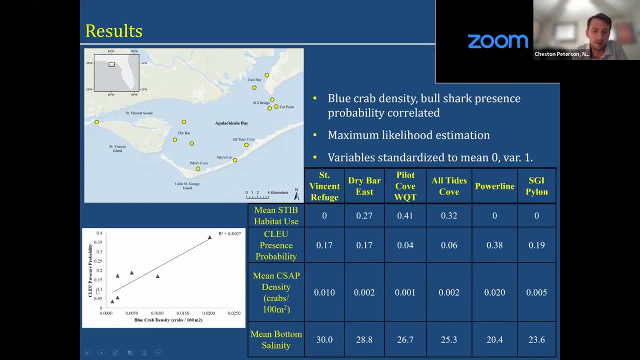 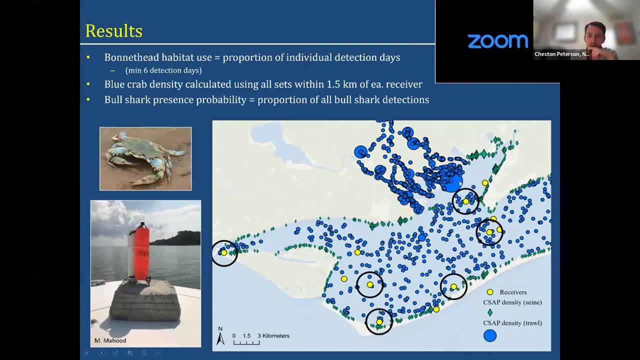 of bull shark or sea loo presence on the y-axis, and you can see that, um, bull sharks were more likely to be present in the areas that blue crabs were the most dense, and that makes sense because, uh, blue crab density is really high up here in the, in this freshwater area, um, or this. 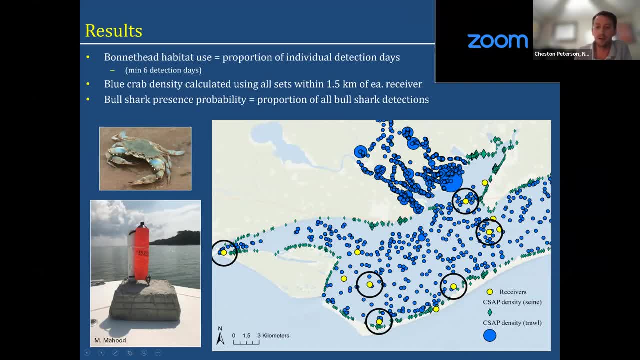 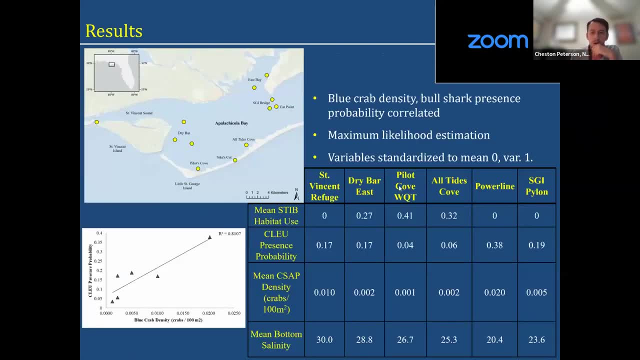 uh, i'm sorry, not freshwater area, but a river dominated area where you have more freshwater influence, and so i think bull sharks were more common up there. uh, we use maximum likelihood estimation, uh, in the model, and the variables were standardized to a mean of zero and variance of one. this was just, um, uh, just to simplify the statistics, and so 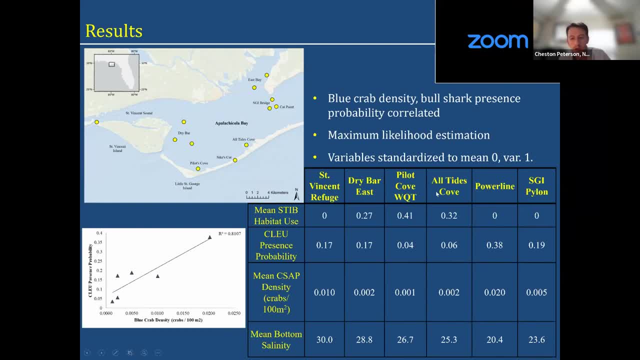 um, i have each site here in this table, um, and some of the numbers for the density of the crabs, uh, the presence probability uh of the bull sharks, and then mean bottom salinity, which was very important because, um, salinity was lowest at those Northern receivers and East Bay. 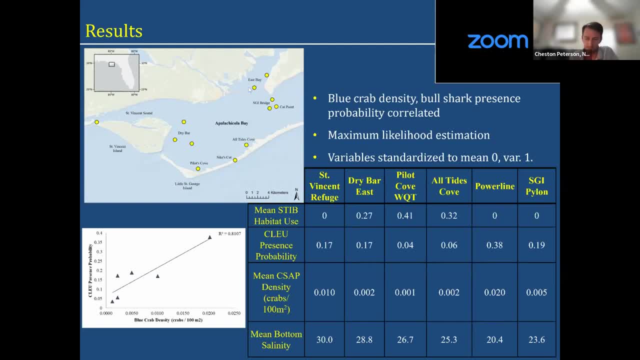 um, where the density of blue crabs was highest and the probability of bullsharks present- excuse me- was also highest, so that's an important factor to keep in mind. we included a random effect in the model for individuals, so we had six bonnet heads and we 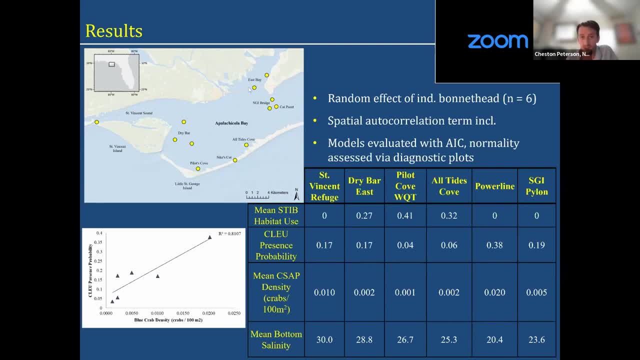 want to try to incorporate the idea that there is individuality among those individuals, so among those sharks. so This is in the model that's just going to throw some noise in the statistical model so that we don't assume each individual is the same because technically they aren't right. 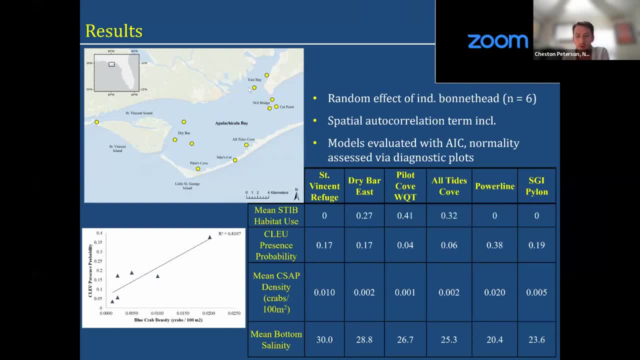 And then there was a term for spatial autocorrelation included in the model. We evaluated the model with AIC and normality assessed via diagnostic plot. So this was kind of the industry standard, the Akaki information criterion. Kind of in the woods here on the statistics, but now you know how this all goes. 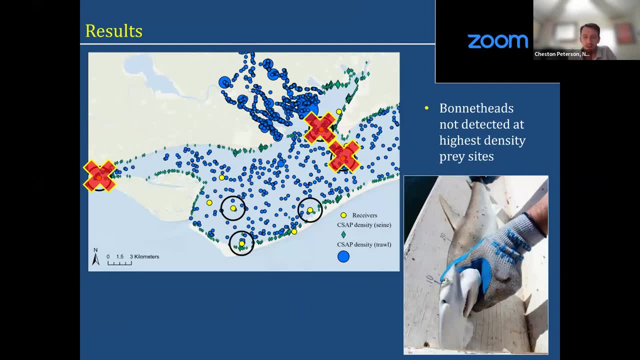 So the really interesting thing here was that bonnetheads were not detected at the highest density prey sites- That was over here in Indian Pass or St Vincent, then at the power line in East Bay and Cat Island. They were obviously detected at the places I mentioned: at Pilot's Cove, All Tides Cove and at Dry Bar. 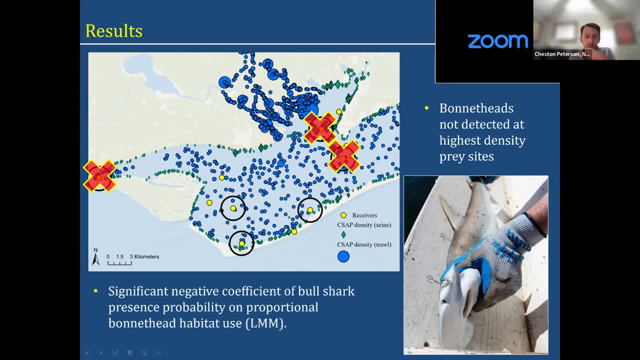 And so this is just our champion bonnethead shark. So there is also a significant negative coefficient of bull shark's presence probability on proportional bonnethead habitat yields- And this is a slide out of my dissertation defense. so that's a really wordy way of saying that there was a significant effect. 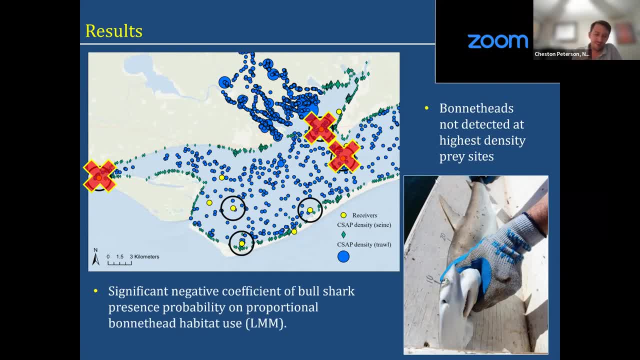 When you go through grad school and you've got a committee that's going to try to ping, you try to phrase stuff really specifically, And so that's why this is. I tried to really Be explicit at what we looked at, but the thrust here is that there was a significant effect of bull shark presence on where these bonnetheads were being detected. 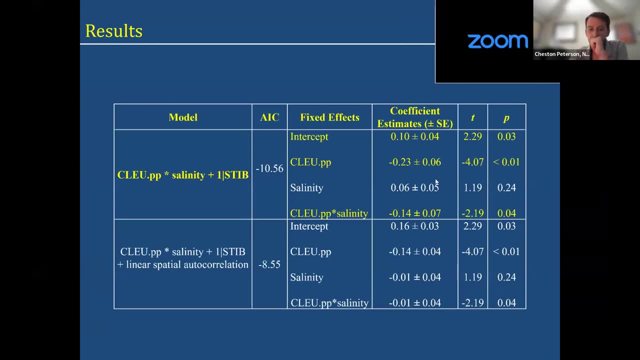 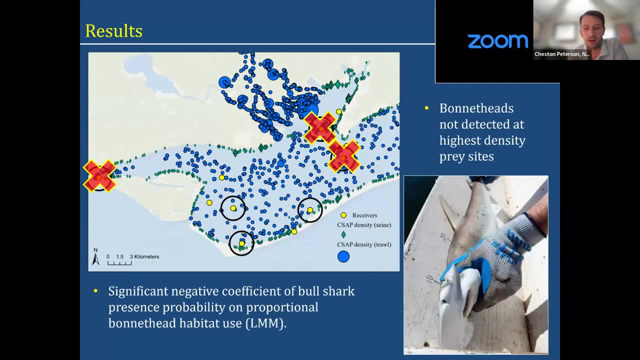 And we did include. I did include salinity in the model. Salinity did not have a significant statistical effect, but I wanted to mention that because that's like the. to me, the most obvious question about this is: what about the salinity? 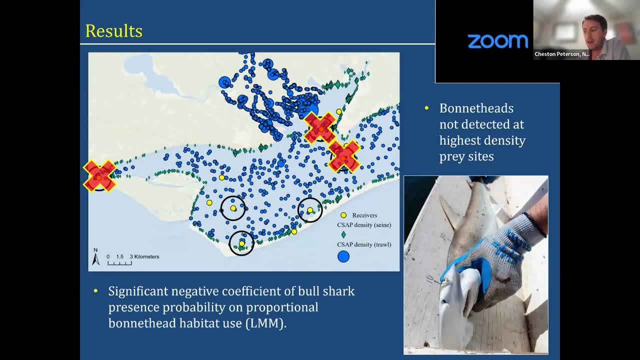 And it looks like salinity wasn't a major factor, And in fact, since we've done this study, we've learned more and more that bonnetheads actually can tolerate much lower salinities than we once thought, And so we saw salinities coming down. let's see. 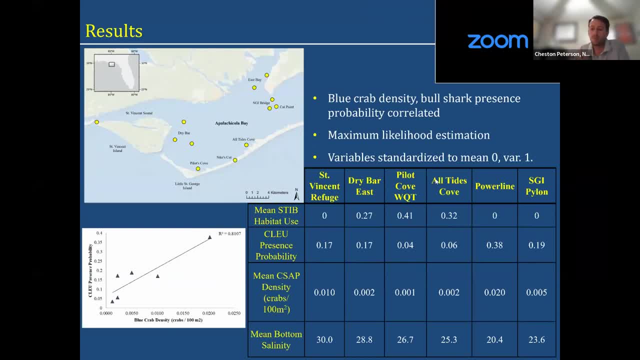 down to this is in parts per thousand, but salinity down to the basically the 20s, It can be as high as 30 to 35,. so St Vincent Redfuge, which is a essentially full strength salinity, And then up in East Bay at the power lines it was about 20,, but that's well within what bonnetheads can tolerate, And so 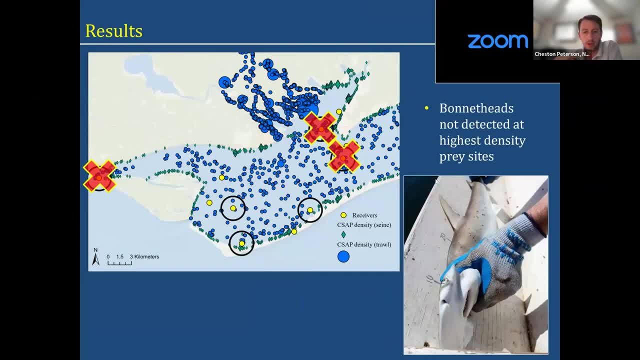 we. we think this is a real pattern. We don't think this is influenced too much by environmental covariates or that kind of thing. The low salinity could be a stress factor. So in addition to the presence of predators, other things, it could be that. 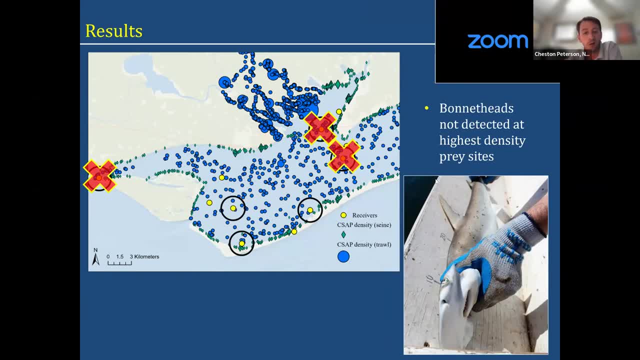 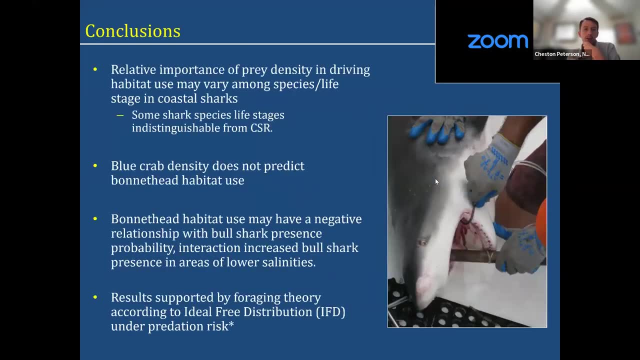 this is just a really stressful environment to be a bonnethead in, because salinity is low, water clarity is super low and there are predators around, And so just to make some conclusions: the relative importance of prey density and driving habitat use may vary and- oh I'm sorry, that's from a different study- Blue crab density does not predict bonnethead habitat use. 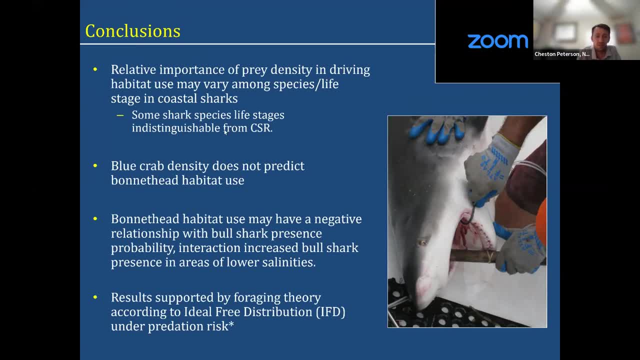 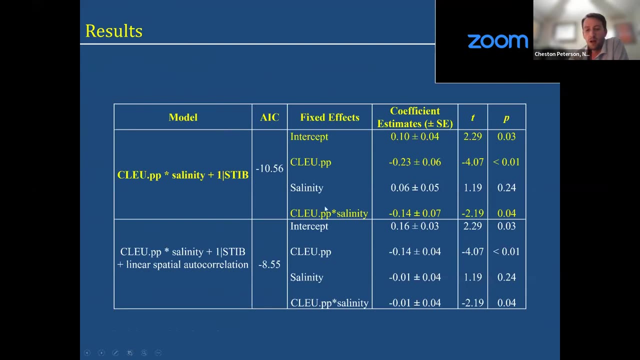 Bonnethead, habitat use may have a negative relationship with bull shark presence probability And the interaction increased bull shark presence in areas of lower salinities, And so what that means is we- oh, I'm sorry, And that's what I missed- There was a significant interaction of bull shark presence and salinity, meaning that they were probably correlated. So I didn't actually quantify that, but the 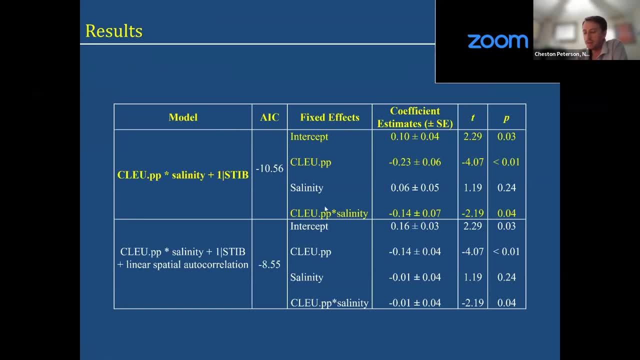 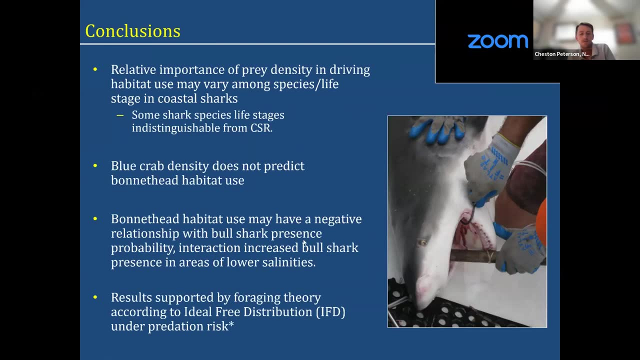 the idea here is that in the areas of lower salinity you had a relatively higher chance of encountering a bull shark, And so that was that interaction there. I'm referring to that, And this results supported by the forging theory according to ideal free distribution, which I didn't talk about under predation risk. but 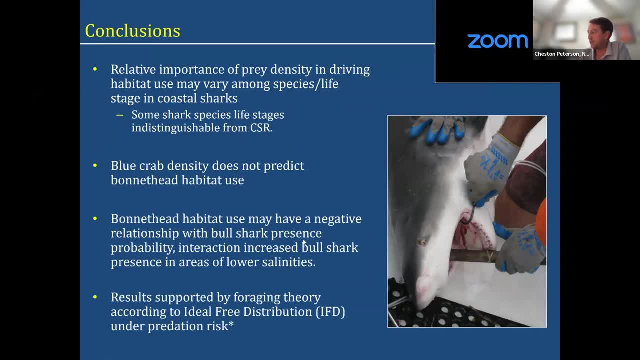 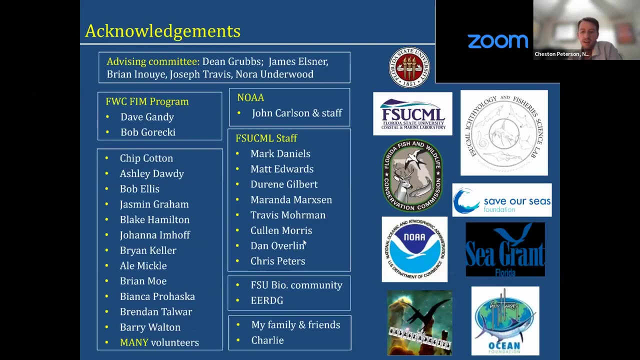 the idea that you are not going to be going in perfectly distributed. the sharks are not going to be distributed in a perfect way and they're not going to necessarily be going into the optimal habitat when under the risk of predation. And that got a little wordy, so I'll just stop there and I'll do that. 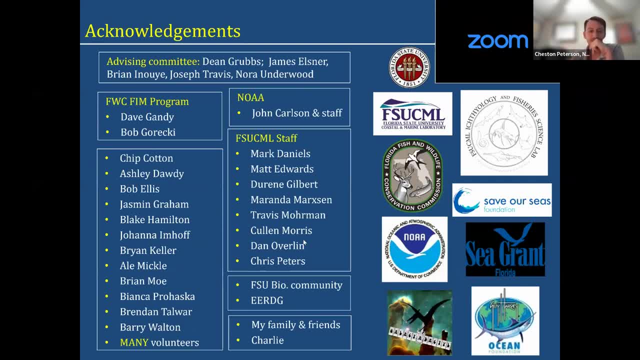 at the end. i'm sorry about that, but just um some acknowledgements for uh, for the project. basically just for this one. i acknowledge my advisor, dean grubs, was extremely supportive, as well as the staff at the ffsu coastal marine laboratory. i imagine this audience is mostly located in south. 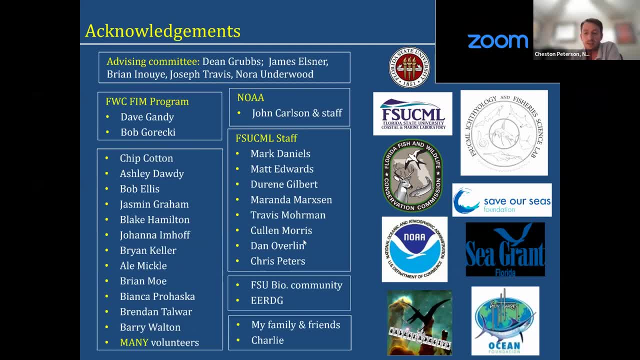 florida, but if you're ever up here, the fsu marine lab is not very well known, i don't think in the greater scheme of things, but it's a. it's an amazing place. it's a really great group of people. they do open houses every other year. it's an awesome place to visit. uh, i just want to. 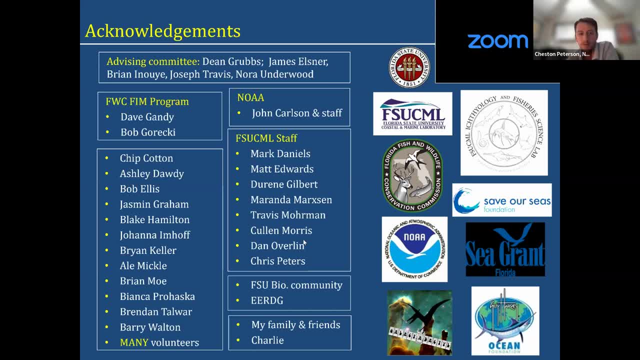 acknowledge fwc dave dandy and bob garecki for sharing the blue crab data, and then, of course, noah and especially save our seas foundation, who are the primary funders for the project. i did get support from um, from florida sea grant, as well as the guy harvey ocean foundation, um after the 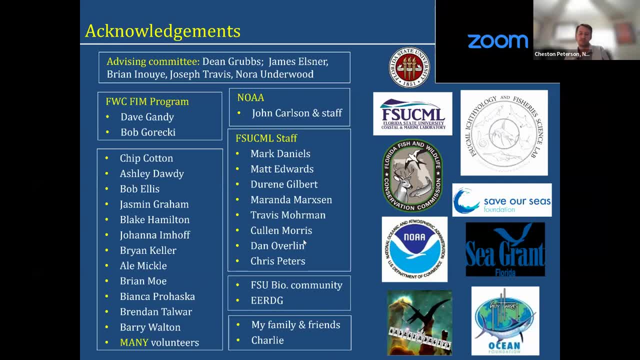 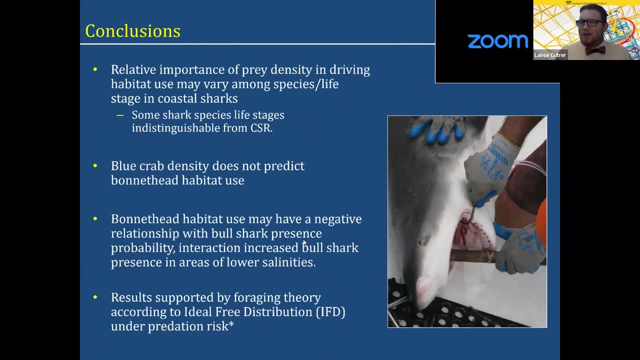 save our sea support and uh, just have some follow-up slides in case you have any questions. but, um, that's it for me awesome. well, that's that's. it's really amazing. i, i know that, um, for a lot of our audience, some of the, the scientific jargon i guess you could say can can get a little dense. 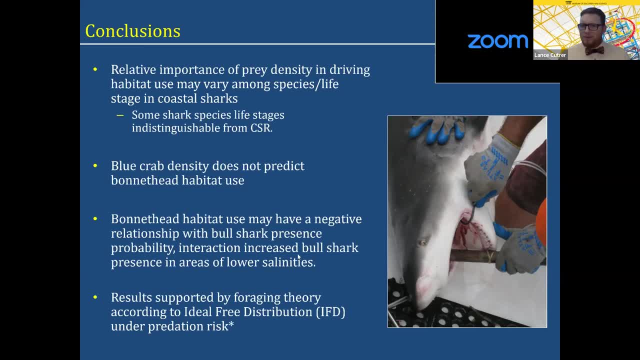 but i think that's. that's good, though, to to present this sort of data and to to really know you've done your due diligence and studying this right, so when you know what you're talking about when you say it, because you've done, you've done a lot of the analysis, which is really 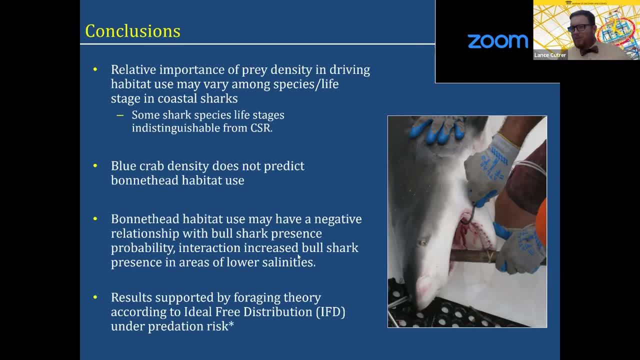 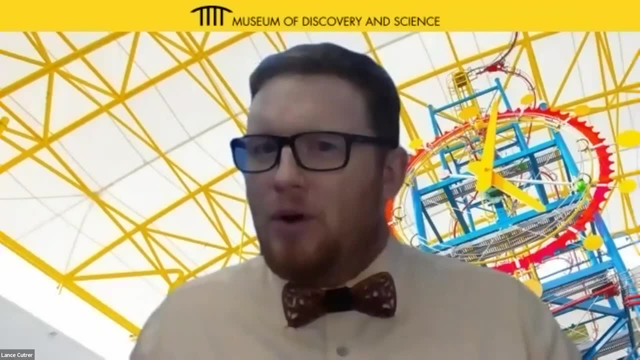 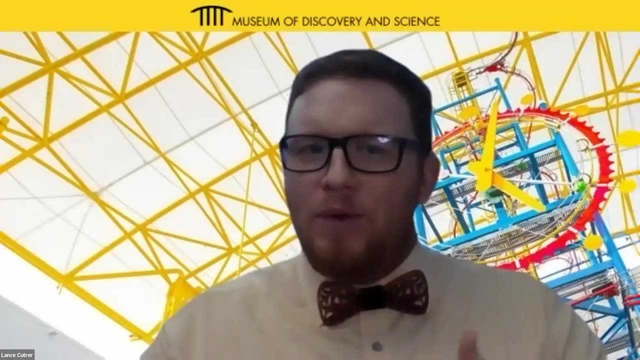 impressive, right, a lot of presentations kind of gloss over that part, but i think it's. i appreciate you including it. so thank you for that. um, we're gonna turn off- oh, turn off- the slide there for a second so we can see each other. um, so, so in the end, bonnethead sharks were affected by the predation. 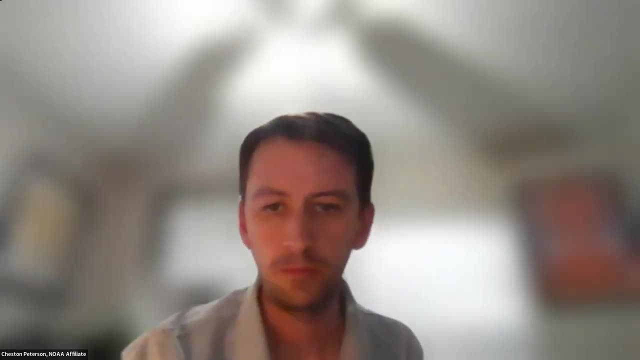 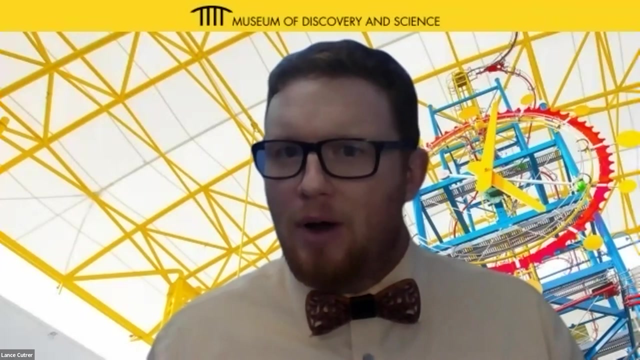 risk of bull sharks, right, and so i think that's a that's a pretty amazing. i think that's a pretty interesting piece of information about footprint, so it's really interesting to hear what's been said afterwards as this gets going. it's been interesting to be able to. 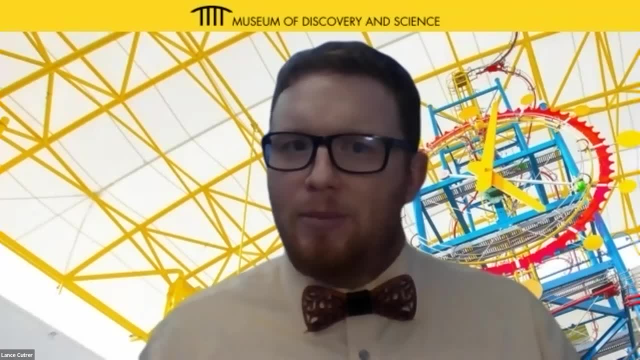 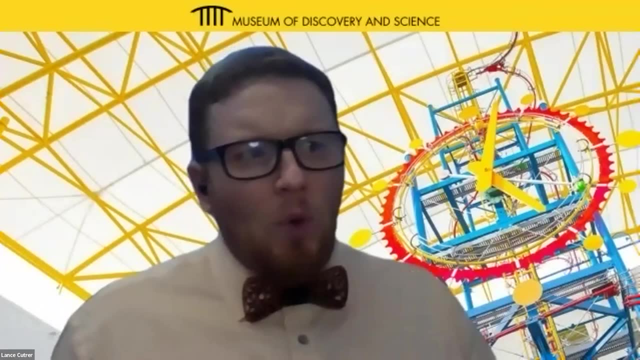 be able to look into what's been said about Europe, so kind of back, that sort of thing. you your piece of information that you were able to glean from. from that right i mean to to be able to look into this, this species, and be able to tell some that detailed information is is quite 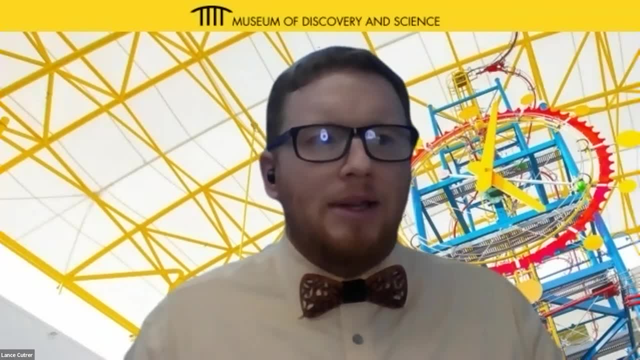 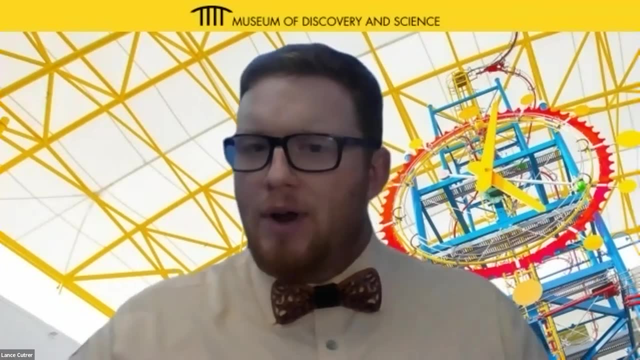 impressive, i think, so kudos to you for thank you getting that done. yeah, thanks, um, we had a few did. do you think temperature could have had any sort of relationship to the sharks, as the water at different temperature coming out of the river as opposed to what it is? 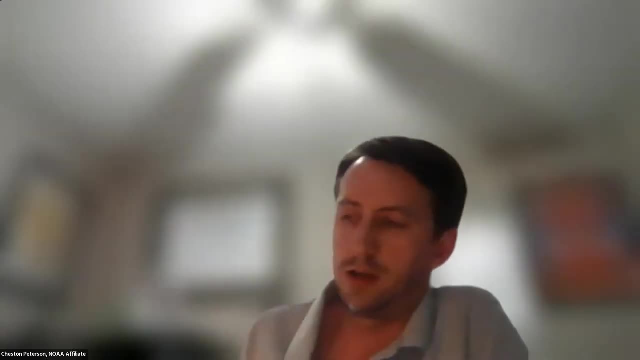 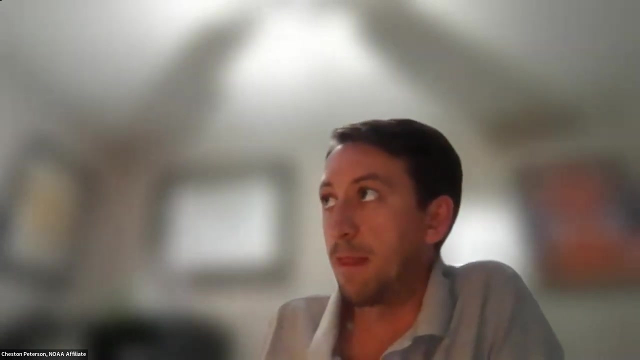 in the bay itself? yeah, that's a great question because generally temperature is a major influential factor for shark movement and habitat use. the there actually was not and one of the reasons we we constrained the study to the summer time, even cutting out some of the spring, was to 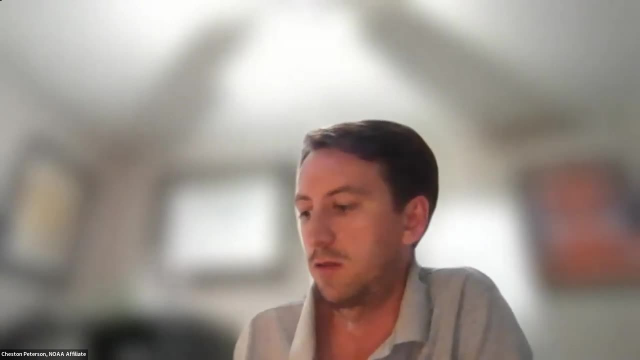 control for temperature. one of the neat things about apalachicola is the there's so much water flow that the bay actually doesn't get as hot as saint george sound. the area to the east and temperature stays pretty homogenous, so there can be some really crazy halo clines where you have 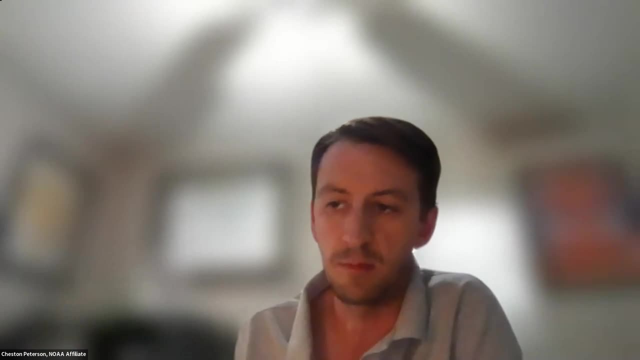 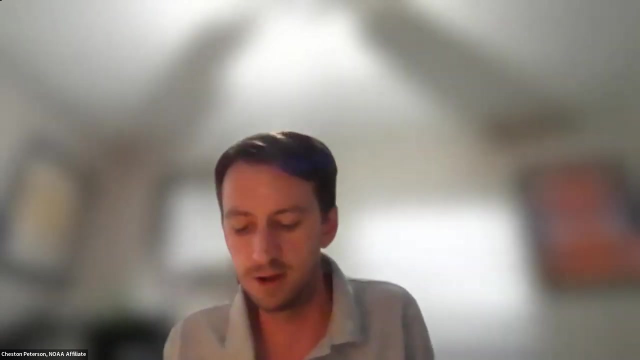 low salinity water at the surface and high salinity water at the bottom, just because of the density of salt and everything and how it separates. but temperature is pretty homogenous. so we don't think. uh, and i did include temperature in some of the early models and that. 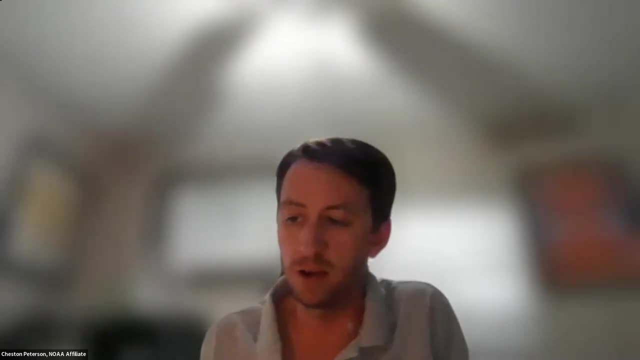 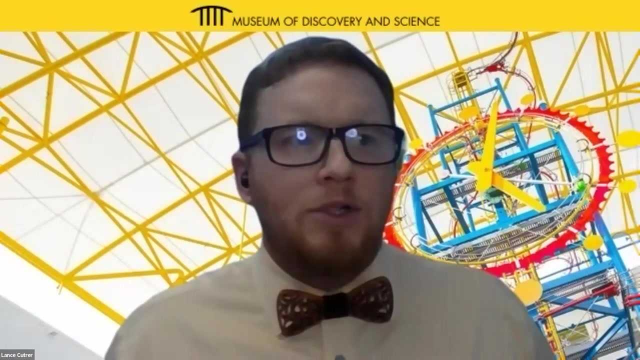 they weren't an influential factor, a useful variable. so that that's a great question, but, um, don't think it's a factor here in the summer time. yeah, nice. and then we had another question about you showed that distribution of when they were there and you said that a number of the 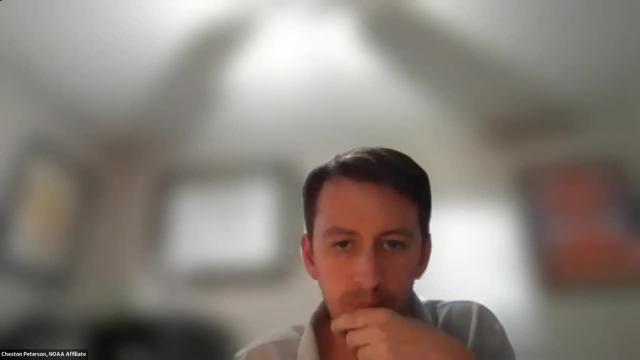 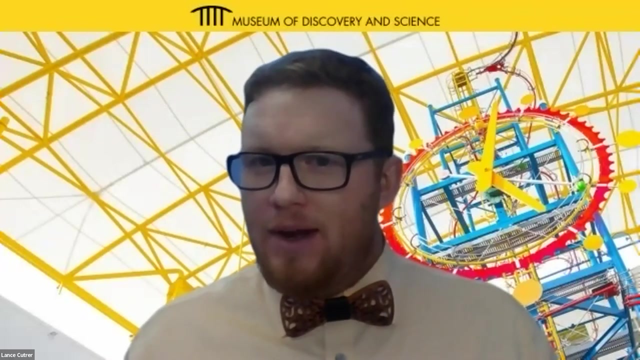 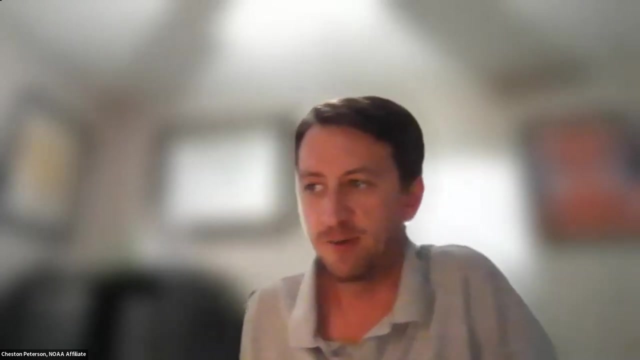 individuals you were able to see year after year, which was really nice. glad you didn't waste your tags. where, where did they go when they're not there? and, oh man right, how long of a period are they typically gone for gone? yeah, excellent question, um, and so for some we can't answer right, um, but 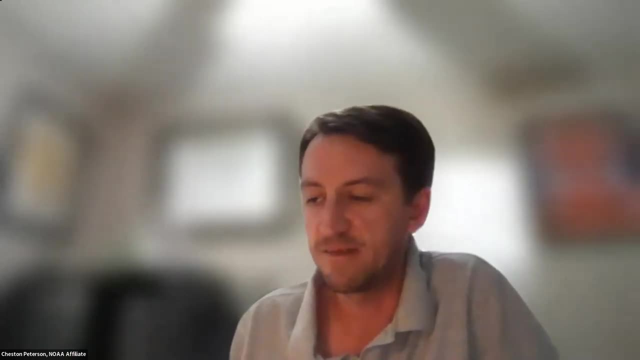 this is one of the really cool things about these studies, um, something that that folks can kind of be aware of. um is there a ton of uh acoustic receiver arrays and we're part of the itag network, which is another thing that's run by fwc. so shout out to them and uh, the fwri, fwc research. 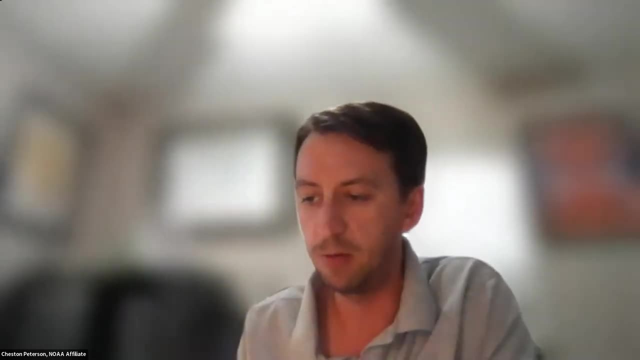 institute um uh, where we have a collaborative network. so if your animals are detected on somebody else's receiver they will let you know, and so we. most of our sharks have been detected in south florida. they've been detected um in tampa bay. they've been detected offshore of tampa. 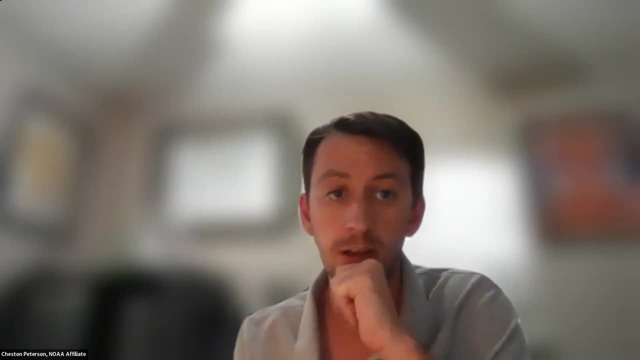 some of the larger sharks have been detected way offshore and like hundreds of meters of water. bull sharks. these are the bull sharks. yeah, um, same thing with the bonnet heads. we would expect them to be going south, but along the coast, so not not just going straight through the gulf of. 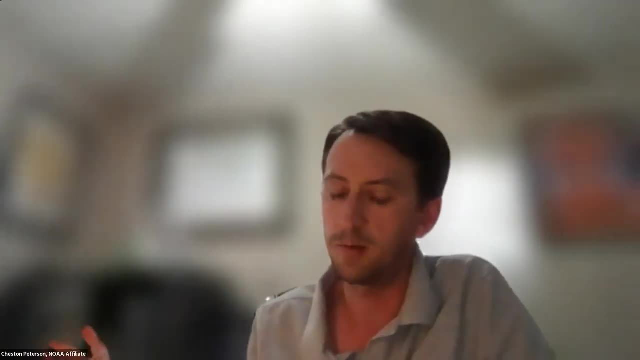 mexico they make some um. brian keller, who's another uh grubbs lab graduate and well supported by save our seas, did a bonnet head migration project and they on the east coast and they made these major coast-wide migrations. so i did not have any bonnet head detections in other arrays, um, so i'm not sure. 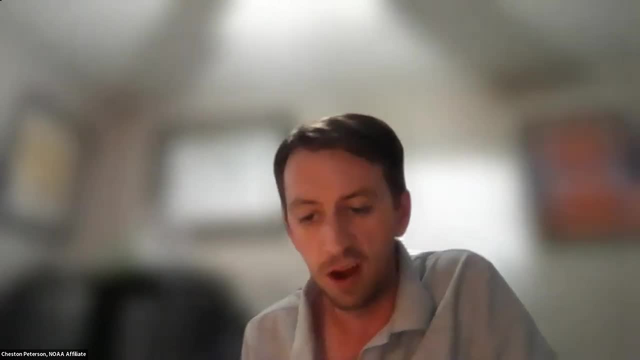 how far they're going or exactly where. unfortunately, you know, we had fewer bonnets be detected and fewer bonnets coming back, and obviously they're more risk, right, so they can be eaten, um, they can also be harvested, um be lost to bycatch and that kind of thing, and so it's tougher to say for them. but but we've had. 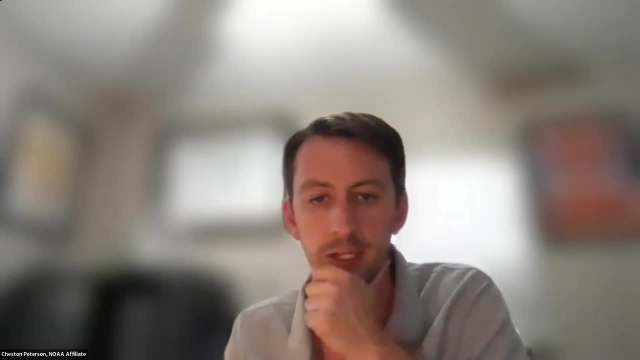 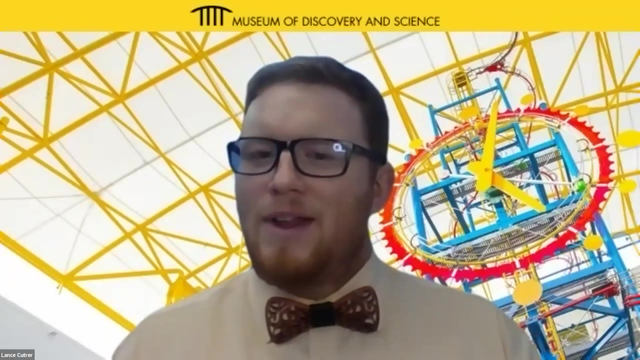 other species that also go south, like lemon sharks, black tips, do this, and so, um, usually if somebody's doing it, other other species are following suit. that's interesting. yeah, that's, that's a. that's a really interesting, uh, collaborative effort. i didn't realize the state had absolutely such a. 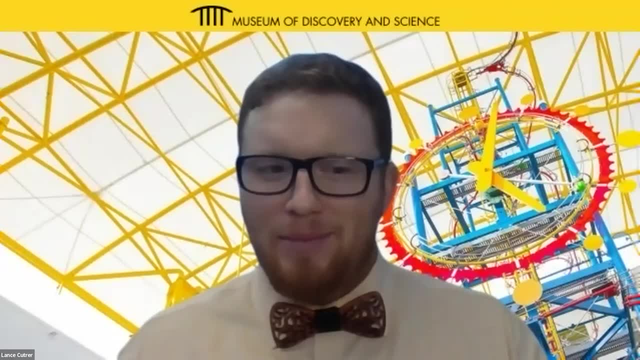 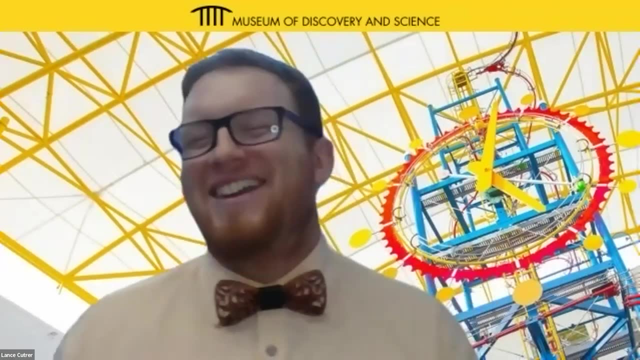 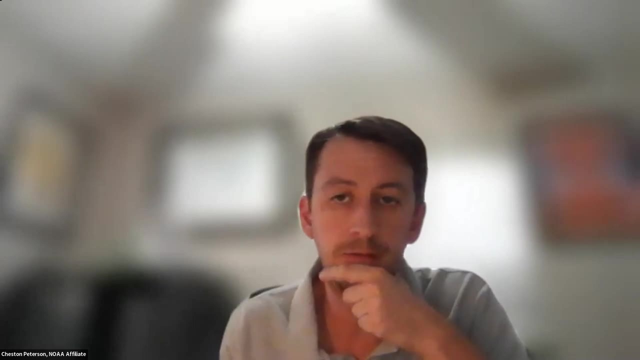 widened network of acoustic film, uh, acoustic, uh tag, um, you know stuff in the water. that's really neat, that's yeah. and it's so nice that they share their data with you. right, it's really great. and there's also the fact array on the on the atlantic, on the east coast, so, um, they have websites if, if. 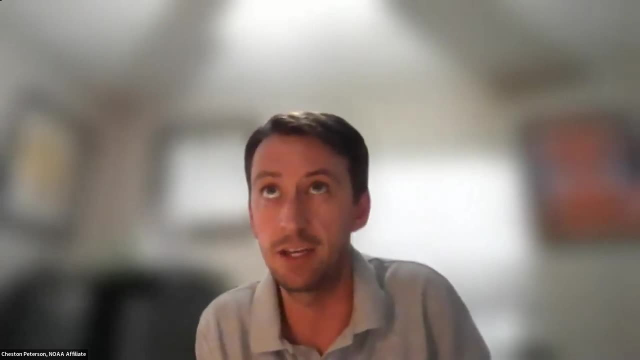 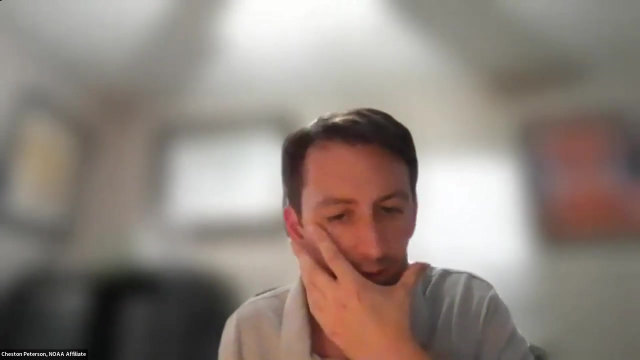 um, you know the folks that attended, yeah, it's a fact, f-a-c-t and i-tag just i-t-a-g. but um, those are, they have, i believe they have some interactive website kind of stuff and just really neat uh networks. we'll have to look it up and share it with with the audience. i-tag f-w-c. i see it now, okay. 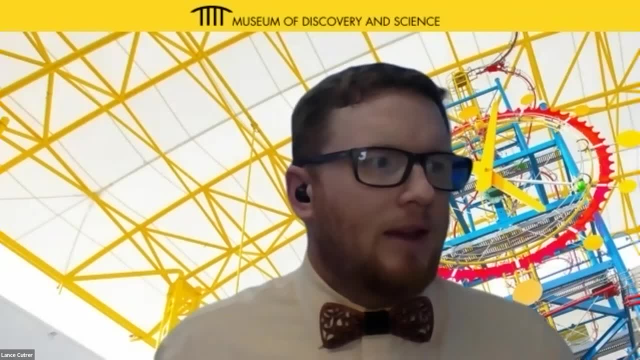 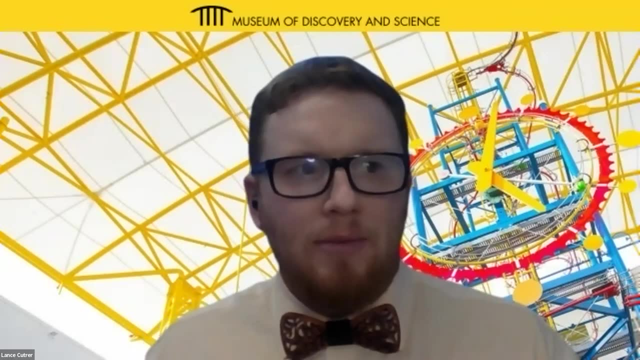 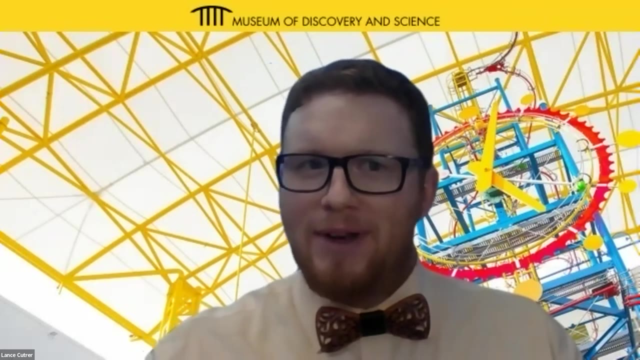 um, i'll drop the the link in the in the uh chat. um, so we have a few more minutes for uh for a few, a few last minute questions. um, about five more minutes or so. um, and i i know that your journey has um kind of started with you growing up in tennessee. i'm, i'm. 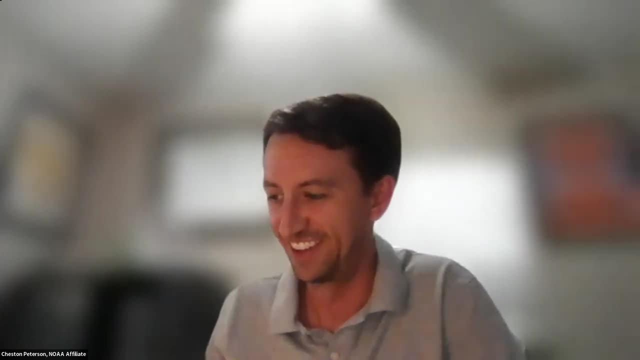 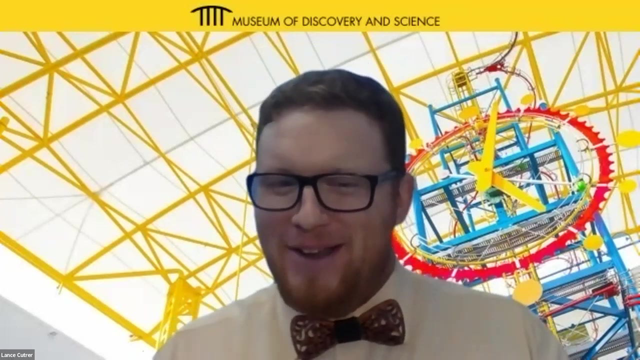 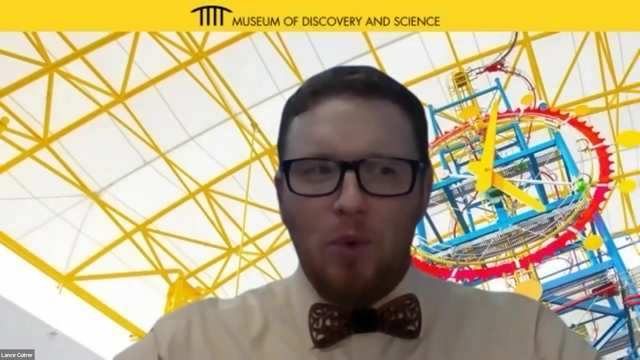 i grew up in tennessee as well, starting with frogs and salamanders. just like you, migrated down to florida to study sharks. you and i share a very similar journey, except you, you went on and did your phd. i, i went and taught in the classroom instead, but um so, so could in. 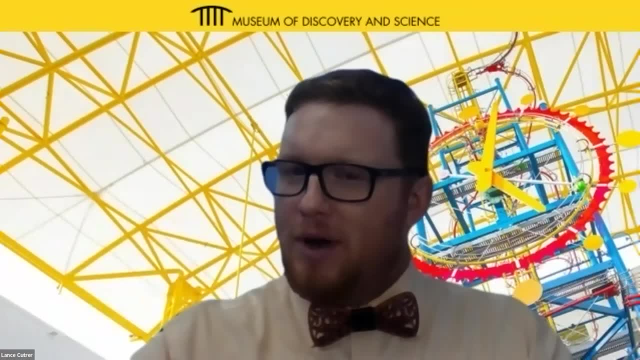 case there's any anyone interested in, in following a career, um, in fisheries, in science, uh, in general, could you, could you kind of give us a synopsis of why you got involved in this, why why it still piques your interest today? um sure, yeah, your general journey, yeah, um, well, you know, as you. 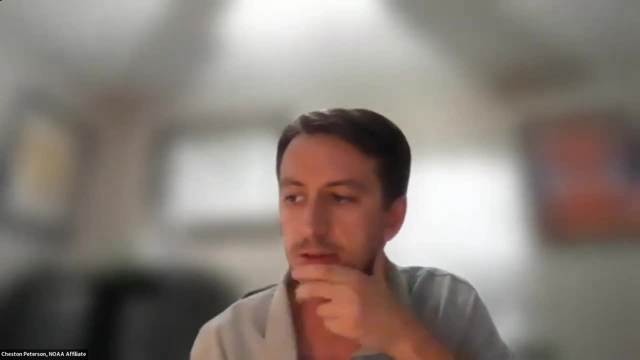 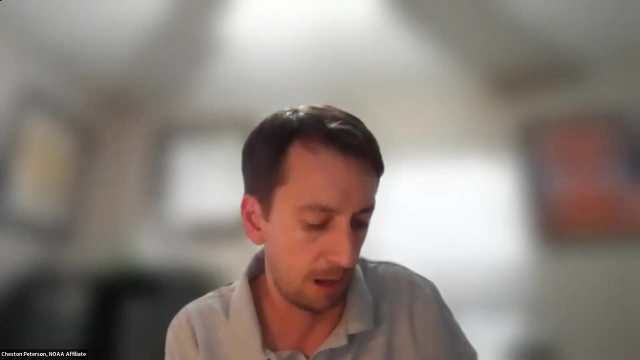 mentioned my introduction, i i kind of just got interested in fishes, um, uh, naturally, just being, you know, i was always interested in life and critters and that kind of thing. and then, um, i decided that, you know, i kind of followed the idea of pursuing marine biology as an undergraduate and 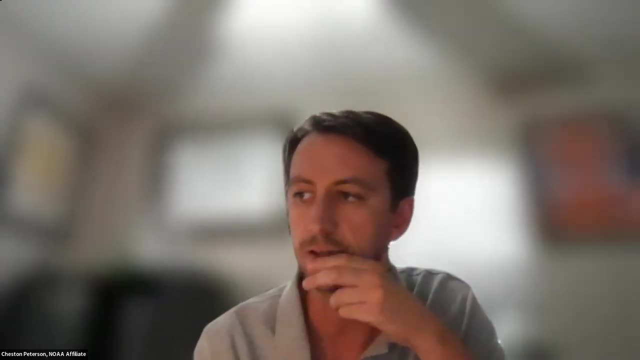 um and then i got really interested in the idea of just doing science, that that um served a broader purpose and information for the sake of information, which is important and worthwhile um. but i really got interested in management and then my path to um, to doing research, actually started. i i got a position as an undergrad working with oyster larvae. 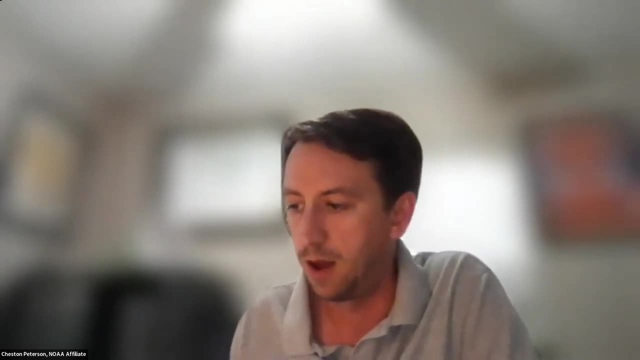 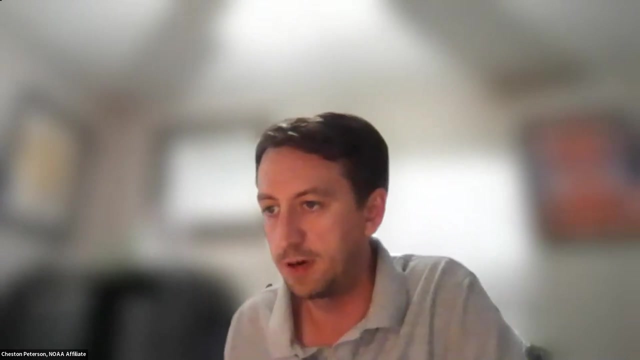 in a hydrodynamics lab and um i i was in a position where i could, you know, volunteer my time where i could. if i had spare time, i'd try to get out with other grad students to get experience- um, i was able to snag that job. you know, i made myself as available as 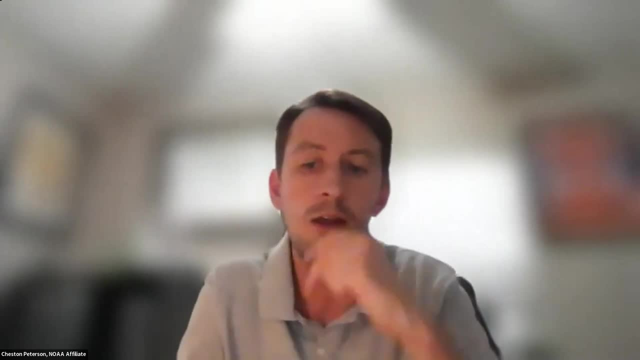 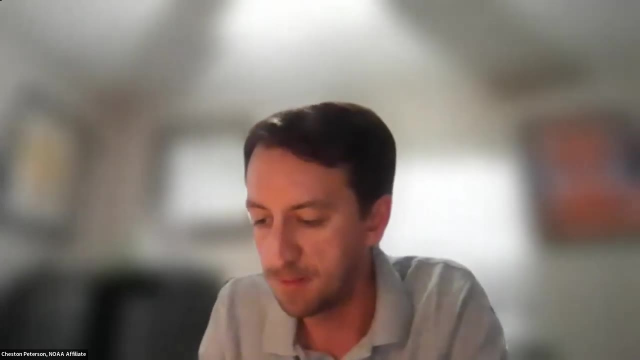 i possibly could, which which isn't always easy, you know, if you're working and um supporting yourself in school and that kind of thing, but um trying to get involved as an undergrad just to get experience, and then, um, i would say my first kind of big break was an internship at moat and that. 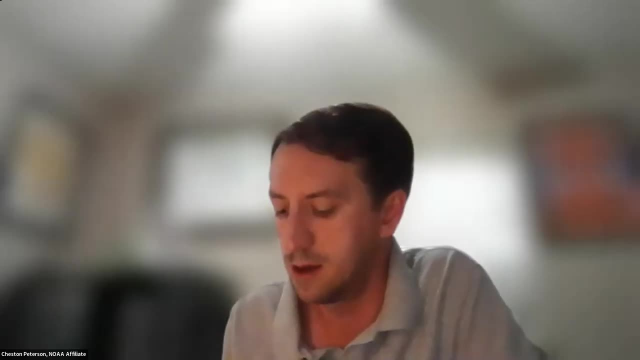 that really set me on the path of sharks and that kind of thing. and then, um, then it was just, you know, getting the grades and, um, trying to do research and build some experience to go to graduate school, and um, you know, i think there's a lot of ways to get there. i 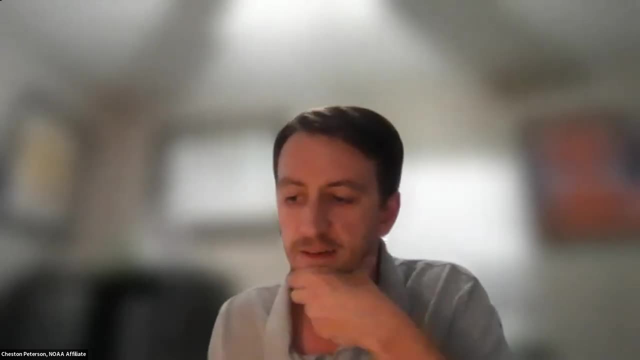 i think what you have a lot of freedom in in undergrad. you really don't have to major in marine biology. it can be biology, it could be not be biology, but the biggest thing is um trying to get experience and my, my advice to anyone that's like: 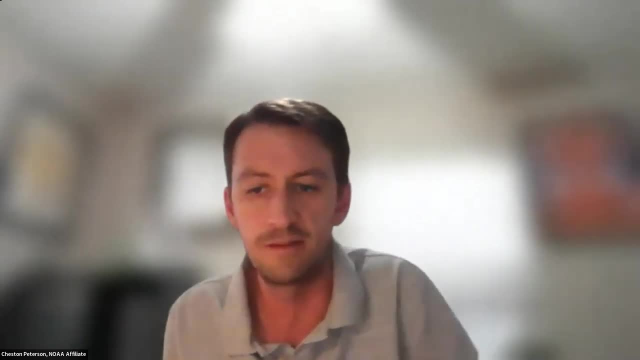 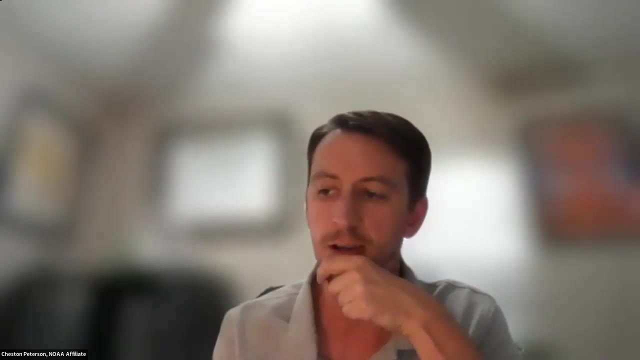 considering this fielder is a little bit younger- is just to try to do as many different things as possible, um, and see what you like, and sometimes that's hard to do with how much time you have and and everything. but the field is moving more, i think, away from unpaid internships as much as they can. 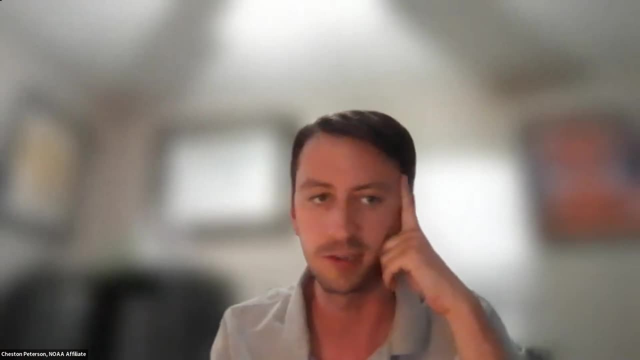 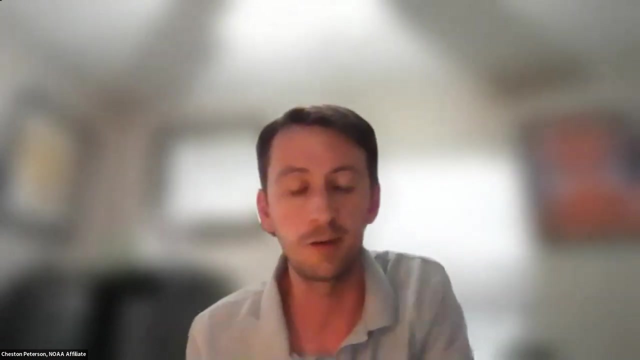 to paid opportunities or um, trying to increase the representation diversity in marine science, and that's a big issue. but a lot of times you know funding's limited, we need a lot of hands, so i was absolutely dependent on undergraduate volunteers as a grad student, um, but yeah, that's kind of that. 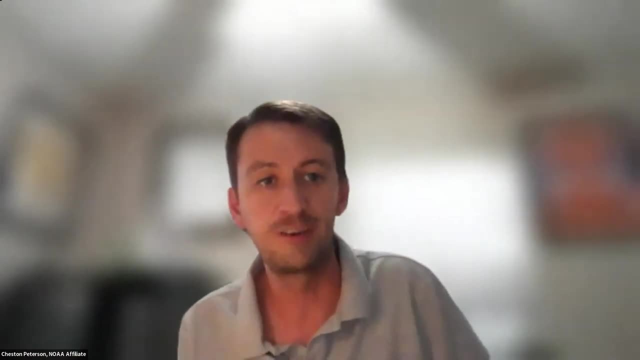 is um. and then the other thing i would say is, like i said, oyster larva, i've had students that told me, like killer whales are nothing like. i'm really sorry, but that's a top tier species that only very few people ever get to work on, and so you've got to be open-minded and recognize that. 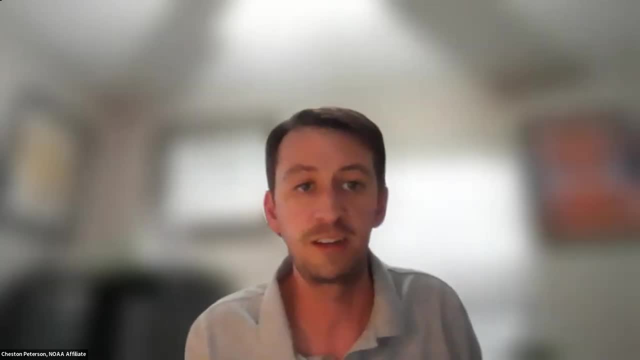 when you're early in your career you know research is research and hopefully it's good quality and all but um. don't turn it down because you think it might be boring or you're not interested in whatever it is. you need that experience and you can specialize later um, so that's, that's important. 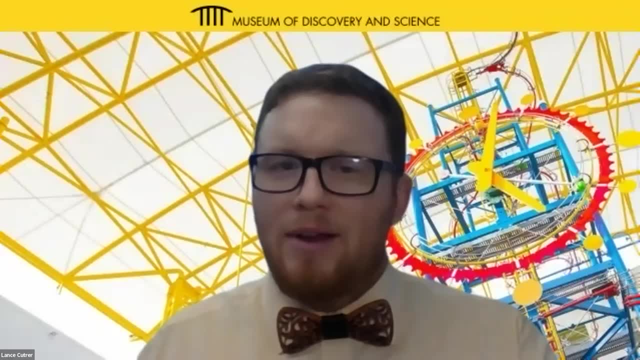 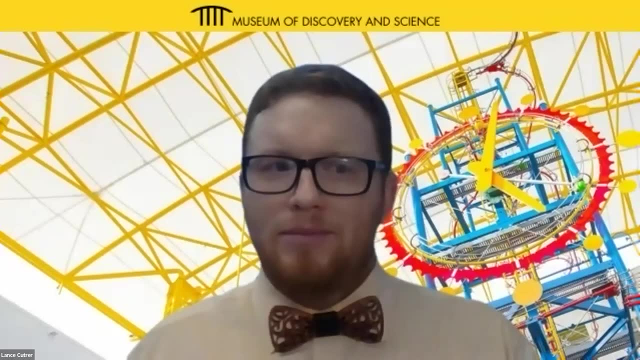 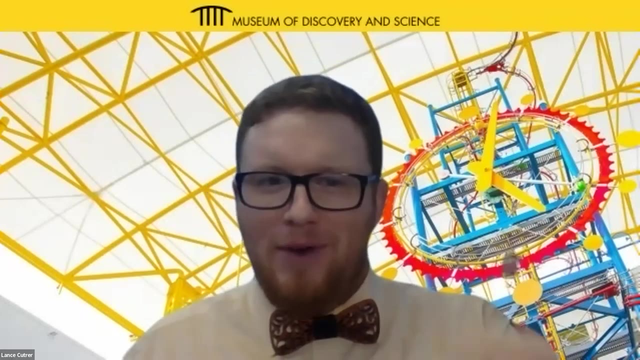 piece of advice. yeah and and uh, it's been a common answer across all of these, all of these series, um, from other guests as well- to kind of ask questions and just follow what you're interested in and just you know, go after an opportunity if there's a volunteer, if there's a volunteer. 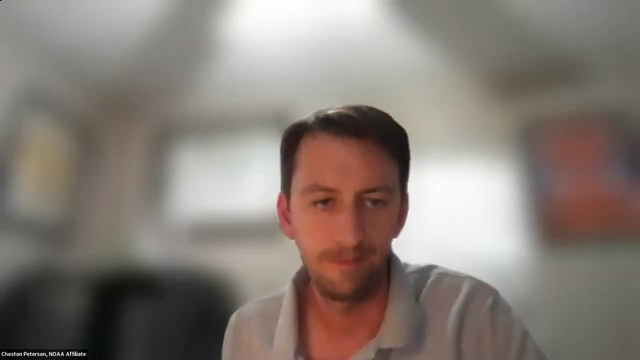 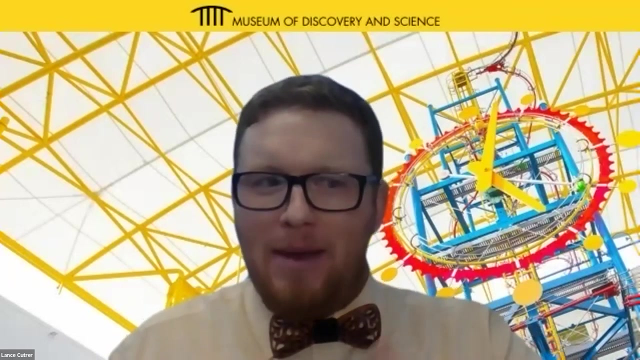 opportunity to go help a researcher on a boat. go, yeah, yeah, right. yeah. well, that's cool, that's good. thank you for that. um. so for for the rest of the audience, that maybe isn't maybe a little further into their careers and maybe more vested in their careers. they can't just switch to. 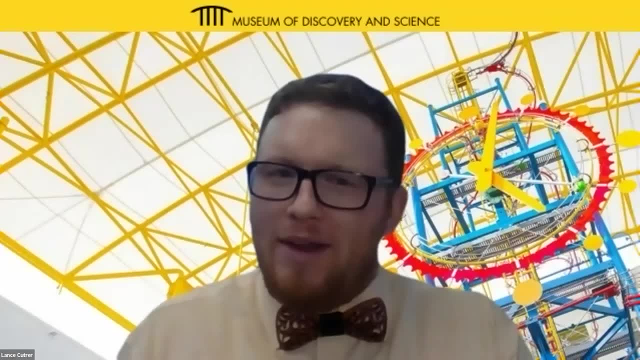 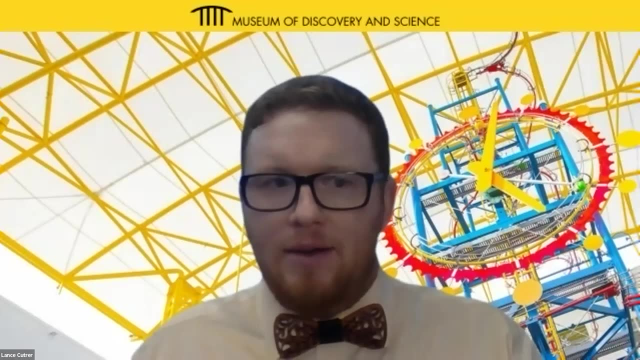 become a fisheries biologist. um, what, what can, what can we do to help advance conservation, especially of marine coastal habitats? you know we have a very? um important coastal marine habitat here in south florida. we have biscayne bay, biscayne bay national park and florida bay on the other side. 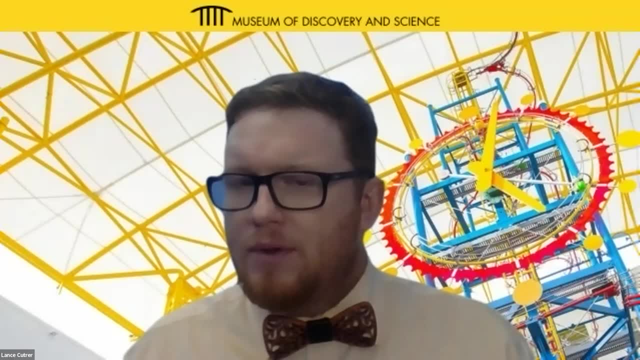 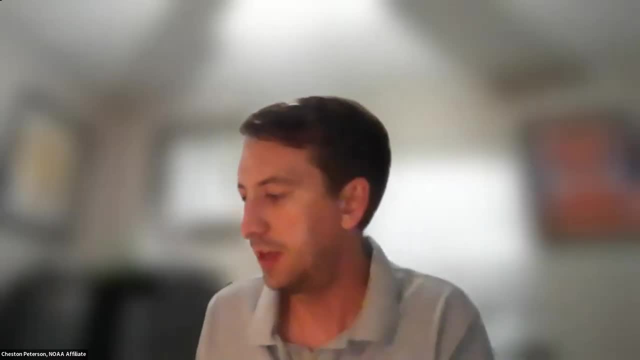 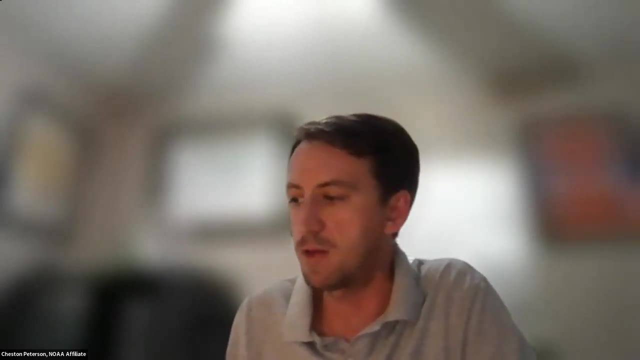 how can we do that and what would be some, some ways we could get involved, um, in helping to conserve some of these places and some of these really important species? yeah, um. so i think, um you know, there are obviously like little practices, like reducing your use of plastic and things like. 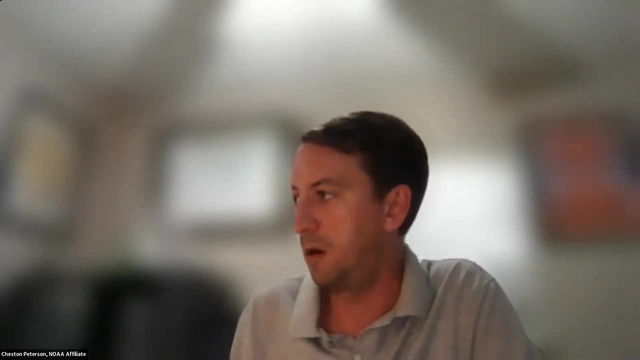 that that we all know about um. the other things i would really advise are our engagement with coastal conservation groups. coastal cleanups um are really important, and then, uh, we're at a. i think it's in florida where, um we have many interests politically, and i don't mean to turn this in a. 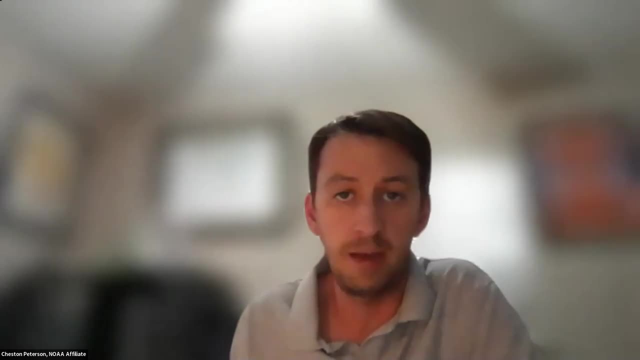 political direction, but having some awareness of what's happening um how at a local, county or state level, that policies are being um implemented that affect these things. that's really where we're we're at, and so, um, just being engaged and and trying to understand the risk, coming to talks like this is a great way to be, to be educated um, you know, interacting with 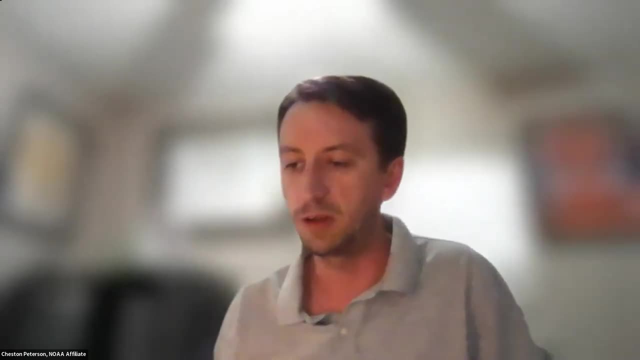 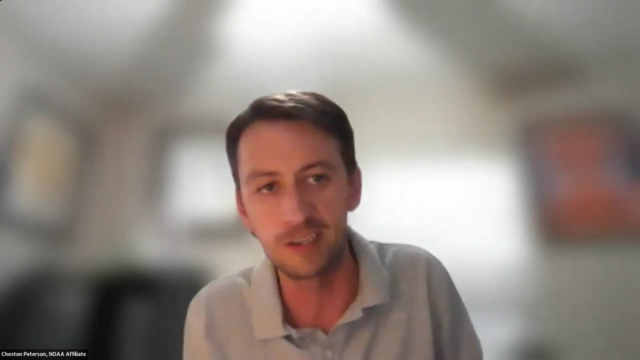 um, and then just kind of spreading the the word to other people and and trying to um. you know, i i grew up with an interest in this stuff and it took me a while to realize that not everyone is inherently interested in this or or has opportunities to go to the beach or whatever, and 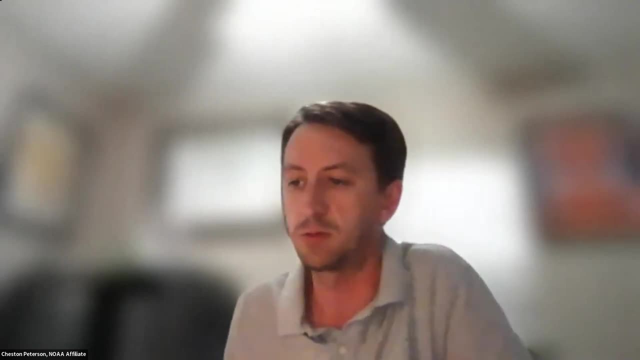 so, um, one of my favorite things to do as a graduate student was working our um, uh, the saturday c program, which works with school kids, just to show, like, take them out trawling and show them the habitat and what's out there and and tell them about it, and so 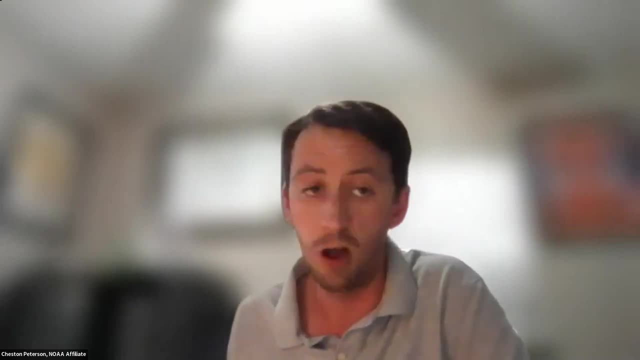 from a from a fishery perspective. you know you hear a lot about sharks, um. they're threats worldwide, um, but domestically we do great and a lot of people may not want to hear this, to realize this, but our shark fisheries are very well managed, um, we have sustainable fisheries. 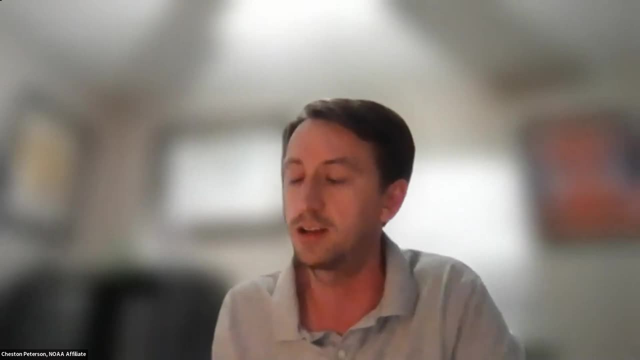 for pretty much everything that is not, that is fished or harvested and protected, and so at home our threats to these animals are mainly through habitat destruction and the destruction of habitat seagrasses. mangroves are extremely important for things like lemon sharks or um, the endangered small two sawfish. um depend on mangroves, which are um, you know are, kind of always. 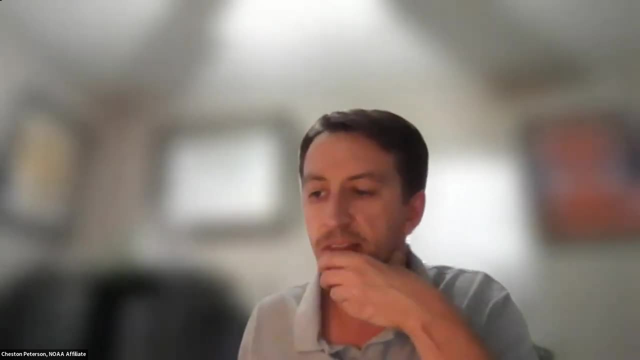 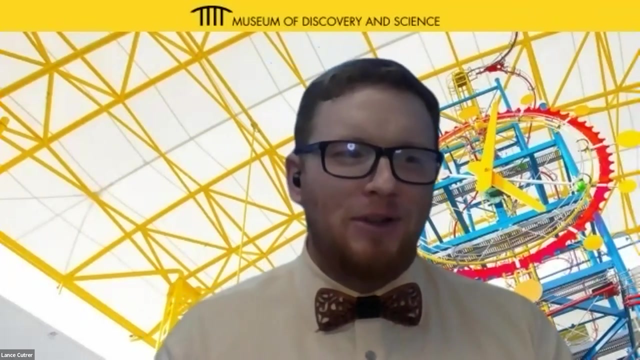 under attack for coastal development and these kind of things. and so i, that would be my advice, that you know at any career point or or stage of life that you could try to get involved in there and then, um, you know, vote with your mind and your environment. yeah, that's, that's a good, that's good. 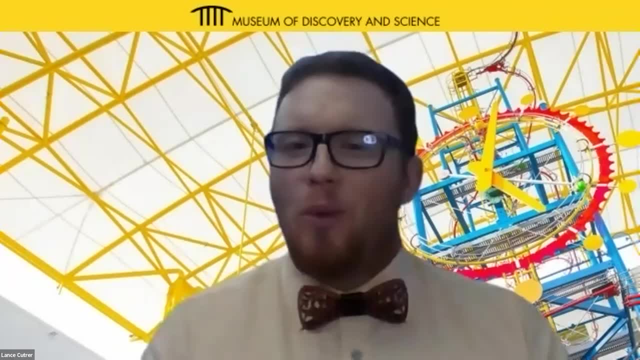 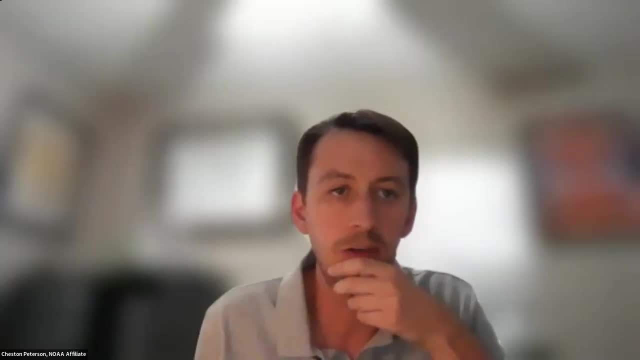 advice. i really appreciate that- and just just being more aware, right, yeah, what's happening around you, um, and and the scale that affects these processes. you know it took me a long time as an adult to realize that like, oh, i got to pay attention at a lower level than you know. 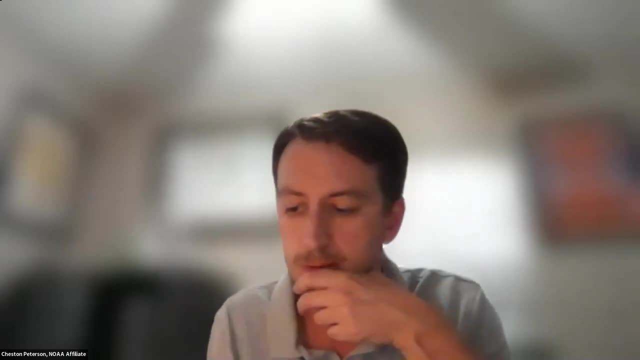 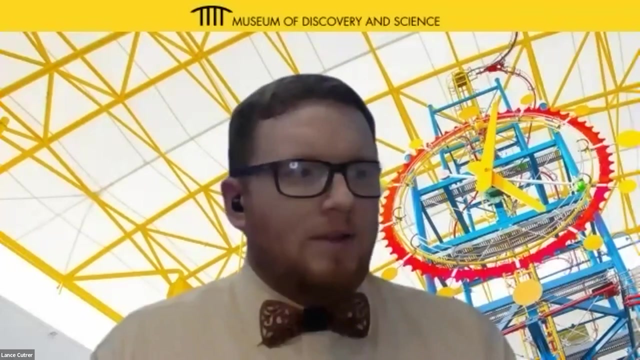 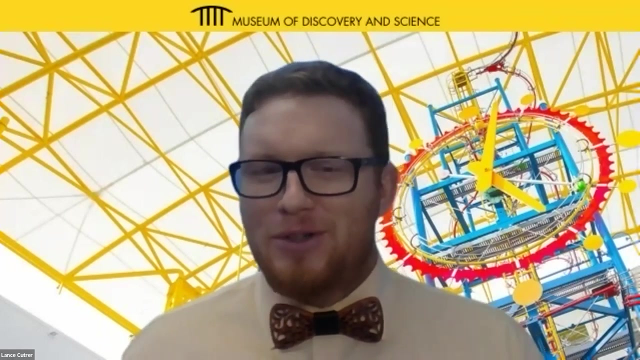 national news and mainstream stuff, just because of, uh, who's making the decisions that affect this kind of thing? right, yeah, all right, all right. well, thank you so very much for your time this evening. we really appreciate you coming on and highlighting your research. um, it's, it's really impressive what you've been able to do, and congratulations again on your phd. 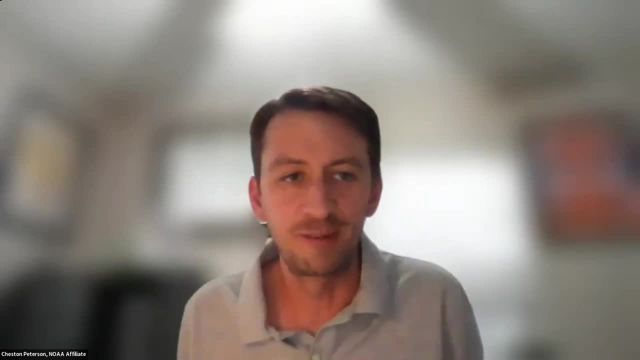 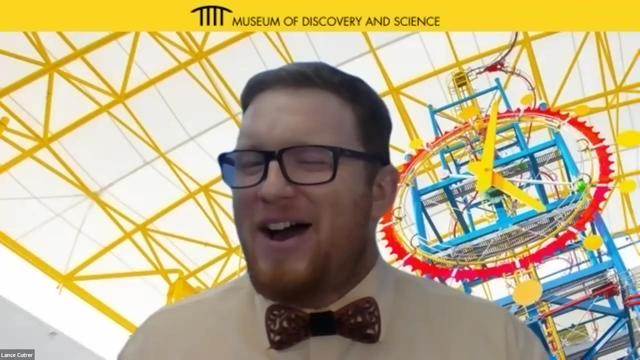 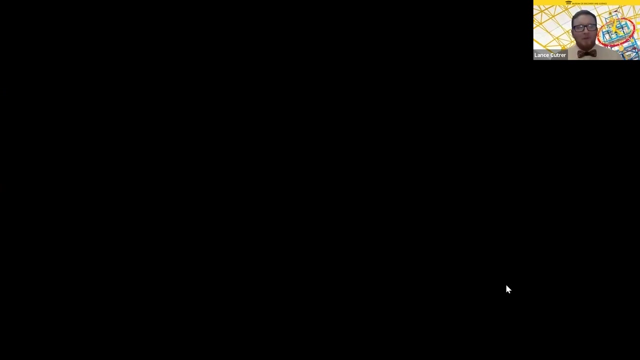 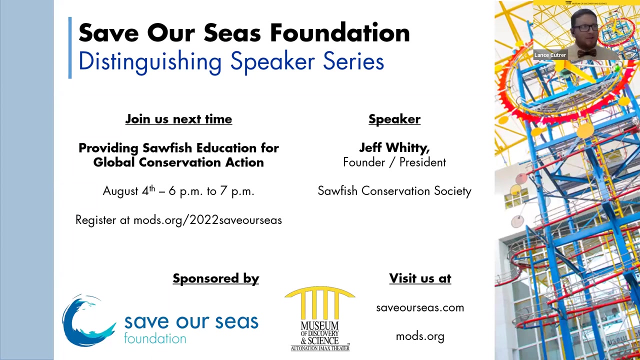 completely. thank you very much. it's a very appreciate it. this is a lot of fun, excellent. yeah, we're happy to have you back anytime. so thank you all for for joining this evening. um, we'll call it there um for next. uh, next month, on august 4th, we have another distinguished speaker series from the save our seas foundation. 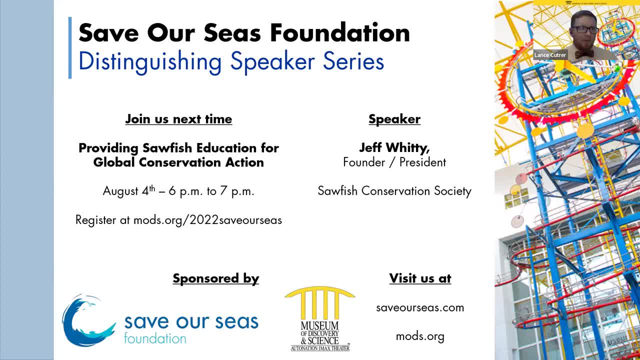 we're going to be talking to researcher jeff witty from the sophist conservation society. so jesson just mentioned the importance of mangroves and sawfish. next month we're talking about them. providing sawfish education for global conservation and action is the name of jeff witty's um project and his presentation, so please. 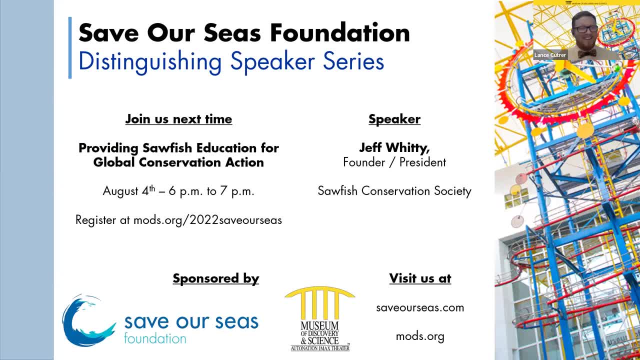 join us then um six to seven ish um on august 4th for that presentation and in the meantime, please, if you're local or not, please feel free to come on into the museum um learn more about um all of our natural ecosystems. we have here um in the museum. all right, thank you so much. 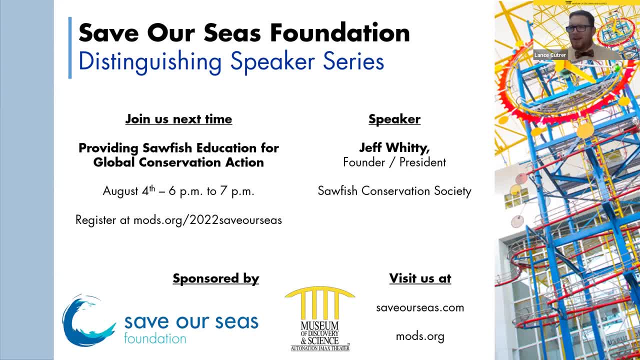 again. dr peterson, thank you very much for joining today and you're quite welcome. thank you everyone for coming. yes, thank you, thank you. we're looking forward to uh next time. thank you so much. thank you all for your time. thank you so also. very much thanks, y'all.